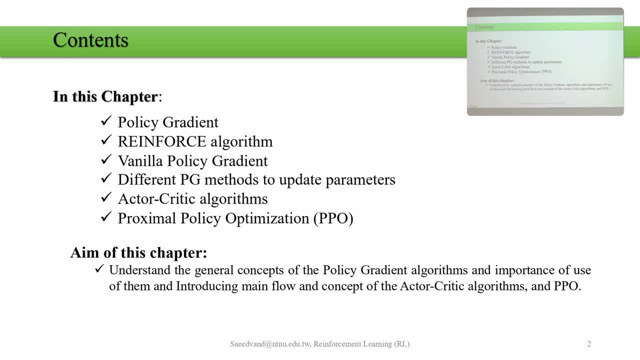 and how it is performing. Then we will see different policy gradient methods to update the parameters. So we are not only limited to one technique like two techniques, like reinforced vanilla. Instead, we also can replace the updating the parameters by policy gradient. 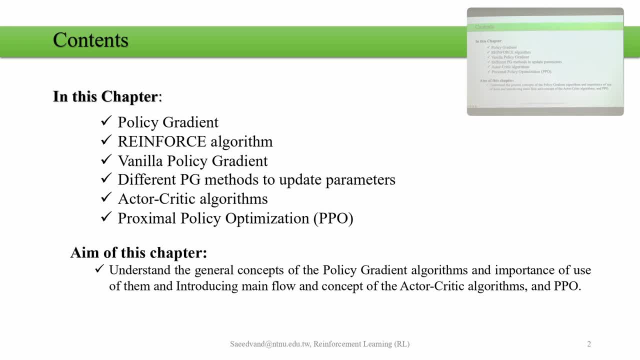 technique. After that we will go through the actor-critical algorithms. We will see, okay, how we can bring the benefits of policy gradient with the already known value function approximation. We will try to measure them together. Finally, we will have a look at the most recent algorithm that is commonly used as proximal policy optimization. 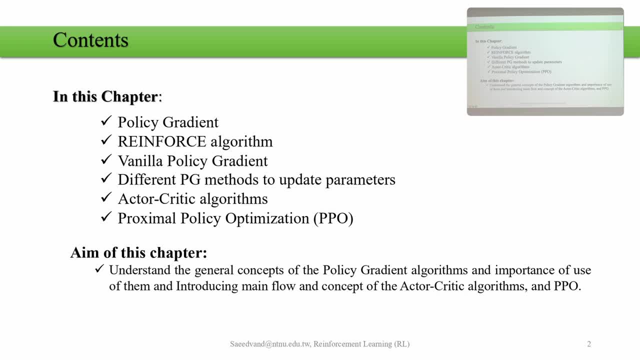 as known as PPO And, as you can see, there are multiple different versions and different implementations. We will see just the base line and we will see how the general idea is working there and what is the motivation that if you want to implement what, you need to do Before starting. 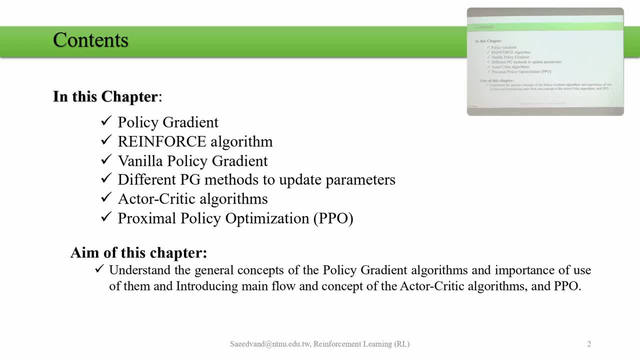 today's course. do you have any questions about previous topics And also better to mention after we finish these slides? I asked to TA to come and introduce you to some of the other tools that we have available. We also have the previous slide, which is available now. that you can use in the next slides. I actually have to say you will have to play with this and see what are the basics and what are the measurements and what are the other features that you can use to do a good task. So this is the first part of the talk and let's get. 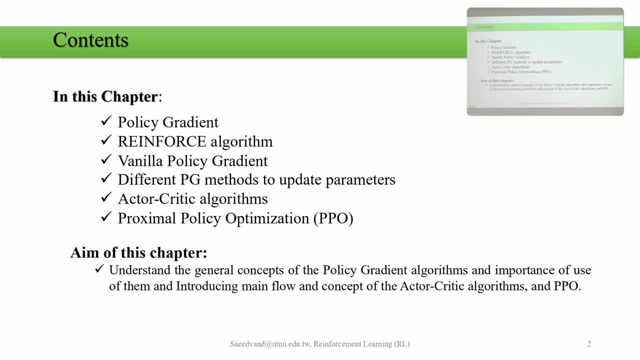 started you at the last part of class- introduce the Isaac gym simulator for you that you can perform the studied algorithm there on GPU. that is, that will be a brief introduction of the simulator- that in future, if you want to develop, develop algorithms that are can be performed faster like the algorithms that you're 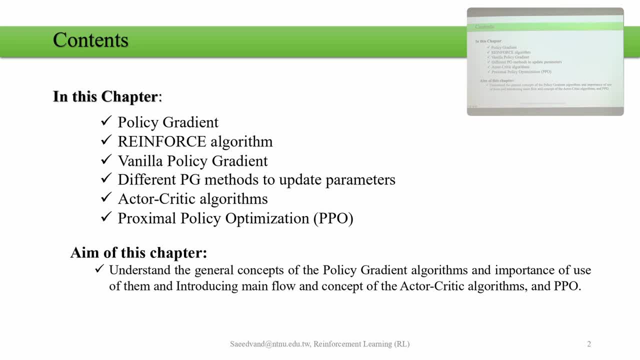 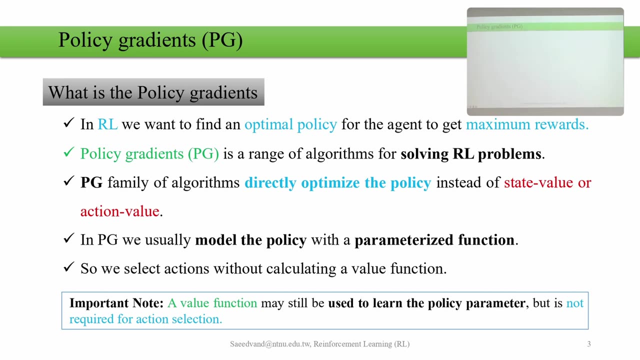 training in 12 hours. 10 hours can be reduced to one hour based on performing on GPU. so if there is no question, we can dive into details of today's course. first of all, let's see what is the policy gradient before also starting. I want to mention almost most of the topics that we studied so far from 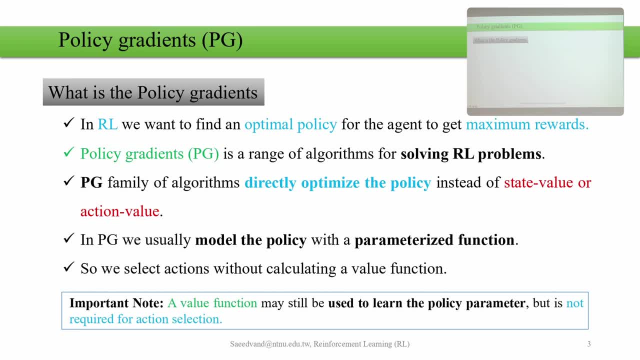 beginning are going to be directly or indirectly used here. so did all the concepts that we discussed. different algorithms are going to be engaged here and you will see how beneficial were. if you remember, I mentioned that in the enforcement learning class, understanding the basics are more important than import learning the big algorithm because, if you know, 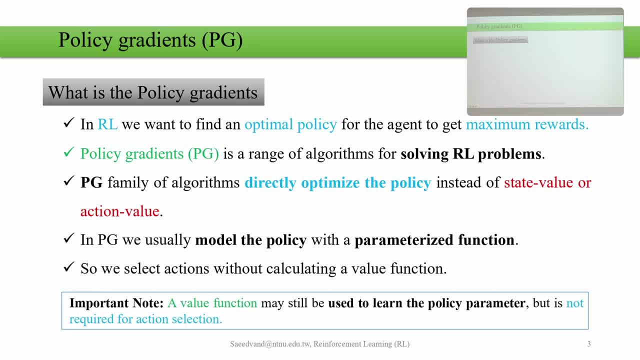 the basics when you study yourself even, can easily understand what's happening. and today you will see, based on flow of policy gradients, that is, in the calculus of policy gradients too, and we now have a few examples that are seen in the report of the policy gradients and you can analyze in detail so that we can see why this is so important. 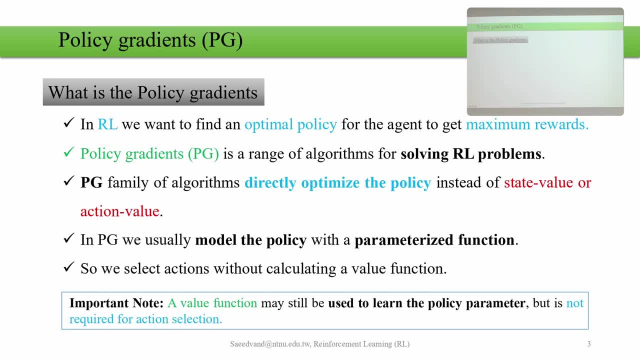 what is the policy gradient that we are seeing in the reinforcement learning process? we can see the same thing here in the reinforcement learning process. so the main objective is to find the optimal policy gradient for all students. right now we have two economics. we are looking at the target class in some cases. 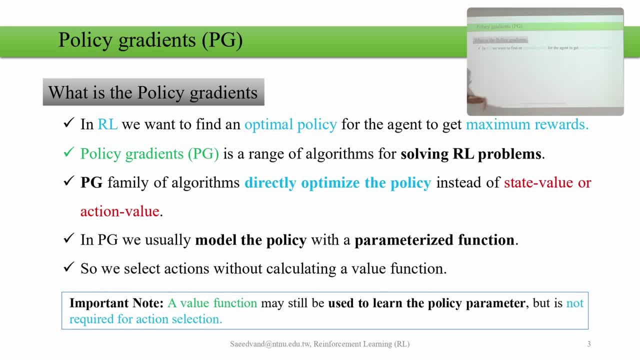 for the agent to maximize reward. So our agent is trying different actions in the environment. We wanted to find best policy that finally we collect maximum possible reward. This was the general idea that we had. So now we're saying OK in policy gradient techniques. 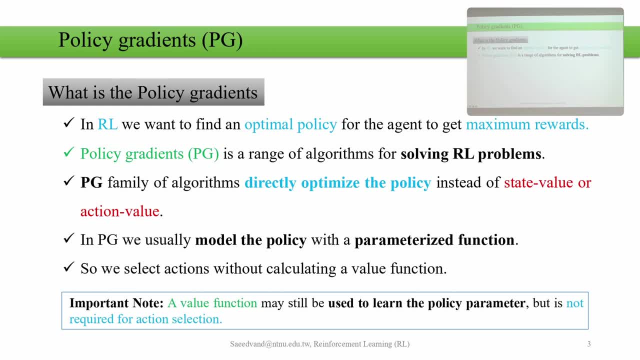 we want to also solve the same problem, same reinforcement learning problem. But here, what we want to do, we want to, instead of working with value function, we want to directly optimize the policy. What does it mean? It means that we don't want to calculate the value anymore. 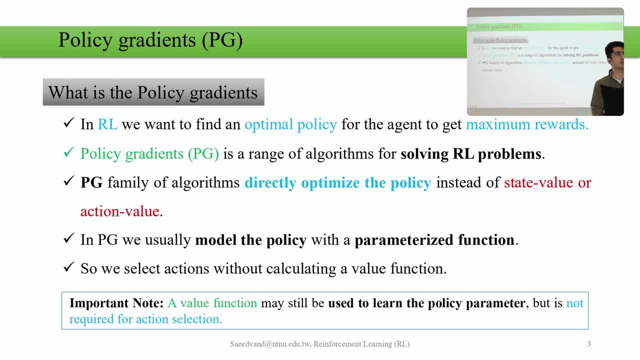 So we had two kinds of value: state value and action value. That one was considering the actions for each state but one was calculating only value for each state. But now we are trying to find a way to not calculate the value just directly work. 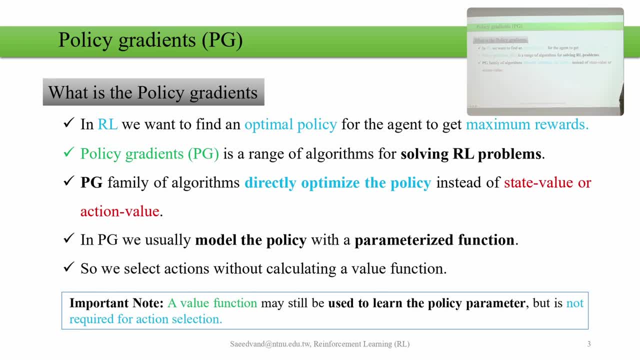 with policy itself and try to improve and optimize the policy itself. And what was the policy? The policy was saying in this state, if I discrete the action, if I have discrete the action, move forward right, left, back. I want to improve this directly, not calculate the. 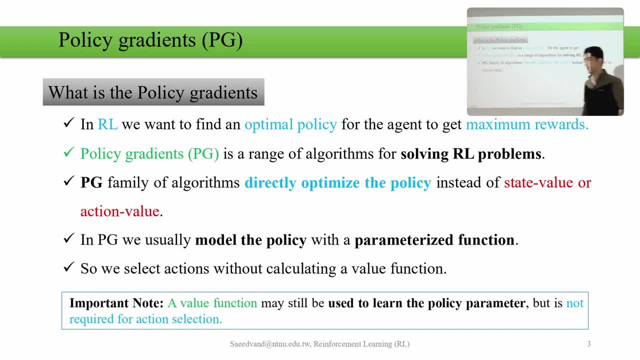 not rely on calculating the value actually anymore. That's that, This idea, This motivation opens a range of different techniques for us. So we say, in policy gradients we usually model the policy with parameterized functions. So now you should think that when 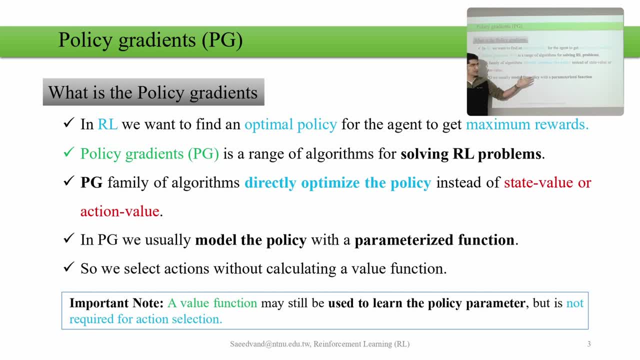 you want to parameterize the policy. we actually what we did with parameterization. we use, for example, neural network in order to calculate some weights. Now we want to do the same. So we have a calculation of weights, but on the policy. 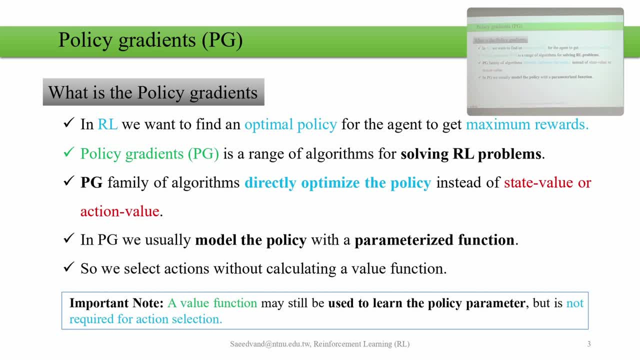 And we will see how. today We are not, of course, limited to neural network or deep learning, but that's the best option that we have for policy gradient series of algorithms. So, as I mentioned, we don't want to calculate the value function. 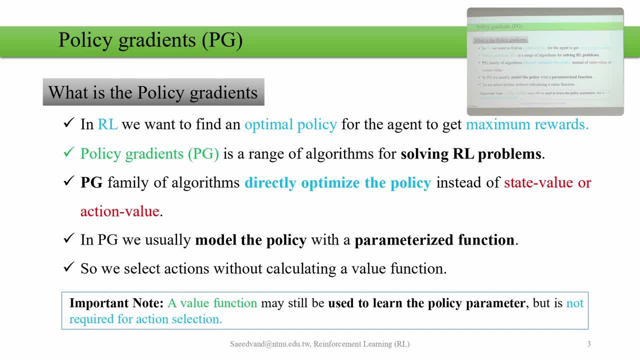 directly, But actually we say a value function. it may still be used to learn policy parameters but it is not required for action selection. We kind of we will see that OK. to evaluate kind of the policy we need to have some calculations. 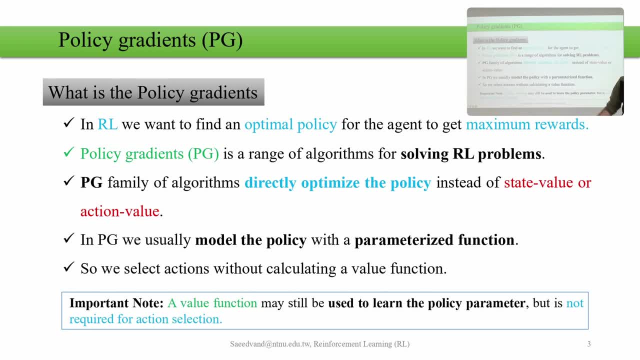 It's not like from error that this action is good and better than the other action. We need to have some calculations, but we don't want to rely on specifically value function approximation, And the reason will be clear soon for you. soon for you. 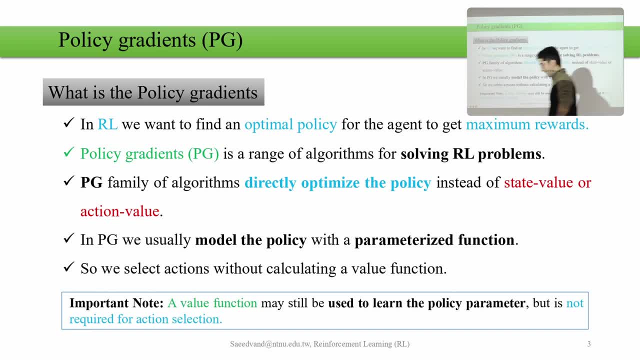 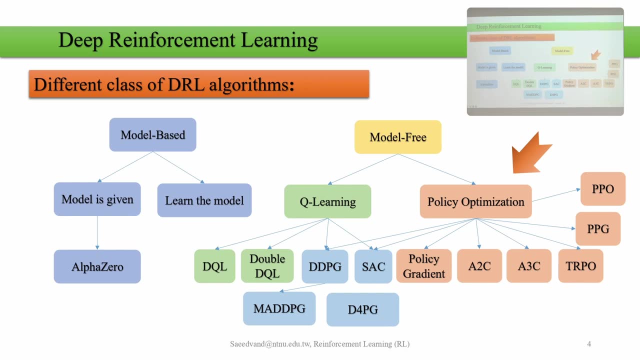 why that's the that we want to avoid it. Although we're calculating, we don't want to optimize based on the value function directly. So, lastly, we've had a look at the different reinforcement learning algorithms. Let's see what's happening and where we are. 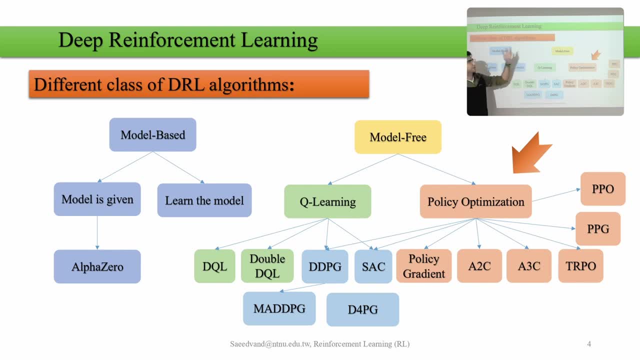 Already, we discussed the model-based techniques in the beginning of the class, In the model-free techniques also. we discussed Q-learning itself, OK, But lastly, most importantly, came to discuss the deep Q-learning And we saw that also it is capable. 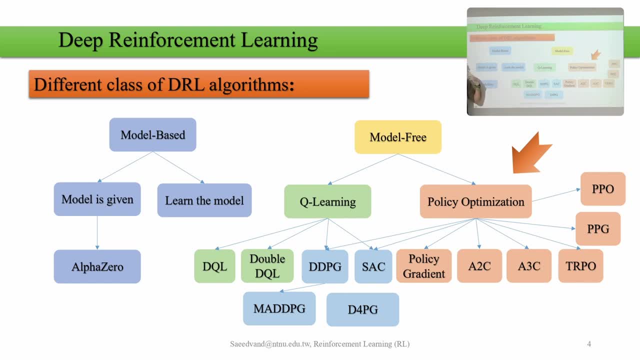 and in some applications it does very well. But on the other hand, now we want to move toward the policy optimization And in policy optimization one of the initial and base algorithms that we have is policy gradient. So we will start with discussion and seeing 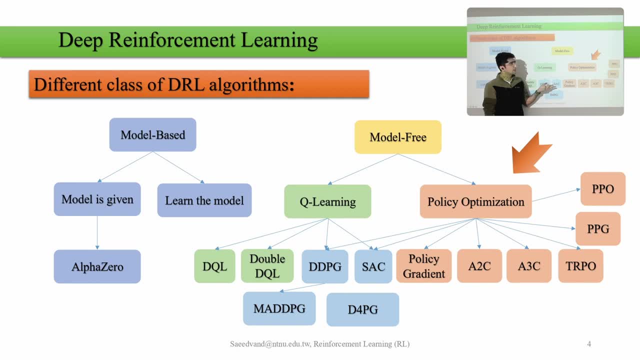 how policy gradient idea is And how we can formulate it. Then we try to see one basic algorithm of actor-critic over here And we have too many algorithms here, like maybe over 50, 100 different. But I will try to today cover the basics. 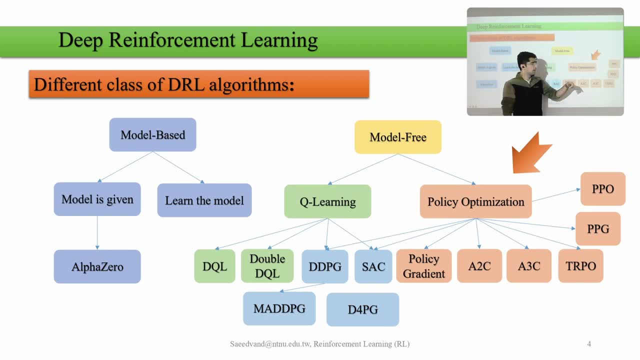 of the important ones: Policy gradient, one technique of actor-critic: We have tripio. That is very similar to PPO But it is very complex to implement And because of that almost no one tries to use it And directly people go to use. 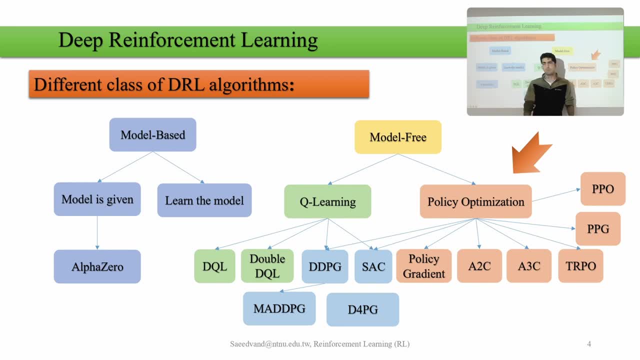 Tripio: the same performance, less complexity. So I also will try to show what is it and what is happening. One note: maybe in future, next semester, after next semester, I will open deep reinforcement learning. that requires one full semester. If you study your book also, it is stated that for reinforcement 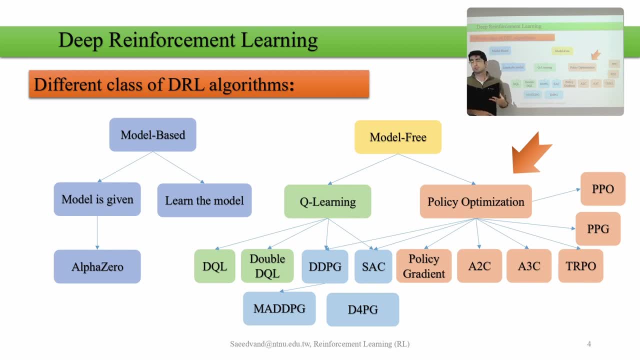 we need two semesters. two semesters to cover all the topics. Because of that, I may open later a semester after next semester to in detail go to the deep reinforcement learning and see how they are exactly working. So is it clear. 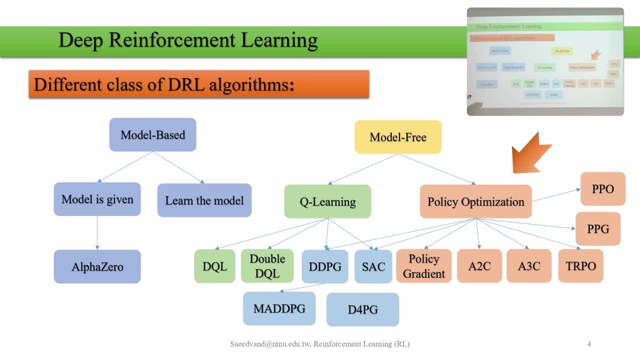 No questions so far. So we've seen this part. We want to see that part And these algorithms over there also. they are variants that they are trying to create And they are trying to create Merge this and this technique together to propose other solutions for. 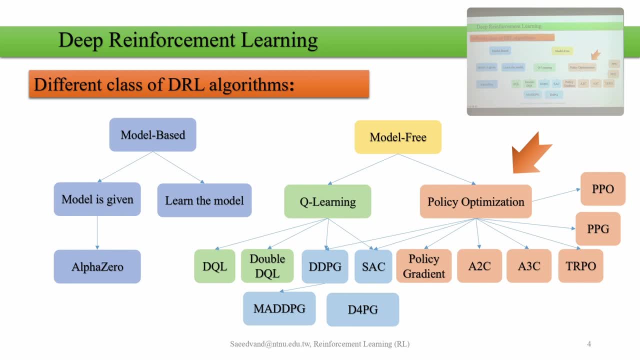 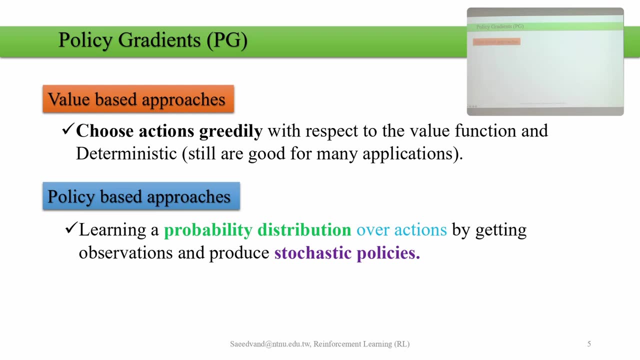 for example, continuous action space- that I will also talk about it today- Or more multi-agent version of the learning based on the deep reinforcement learning. So in policy gradient with value-based approaches, we say we want to what we were doing in value-based approaches. 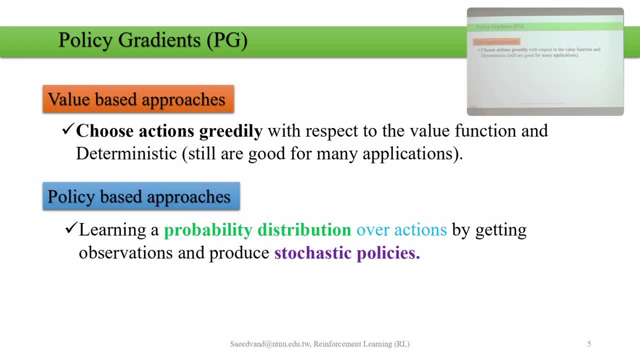 we were choosing actions gradially. So we were calculating values first of all. After calculating values, we were choosing action based on which action can maximize the, can maximize the reward that indirectly, implicitly, also maximize the. we were choosing value maximize. 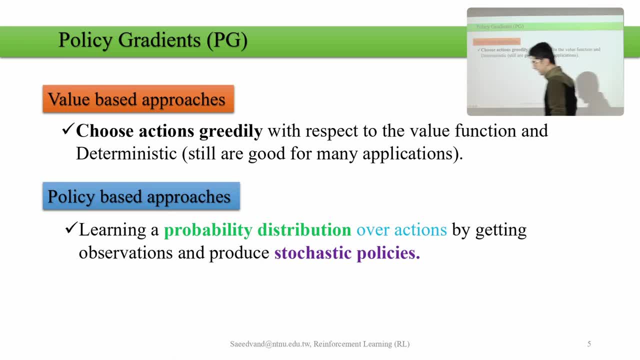 maximum value, that implicitly also max. we're maximizing the reward function that we defined also. So and still they are good for many applications. So with studying policy gradient we're not saying that. so no one should use- no one anymore should use those techniques. 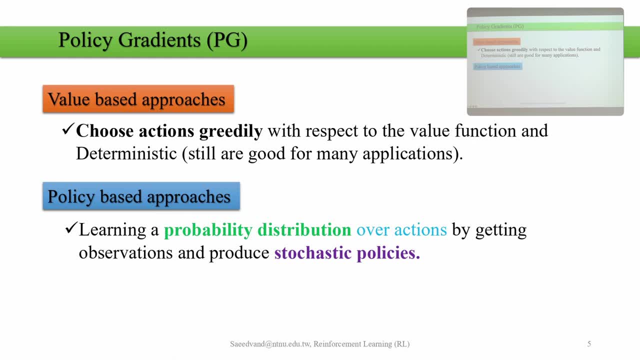 No Policy gradient has lots of benefits, but it's still those techniques that, lastly- if you've seen an example- can work pretty good. On the other hand, now, apart from value-based approaches, in policy-based approaches we are going to learn the probability distribution over actions. 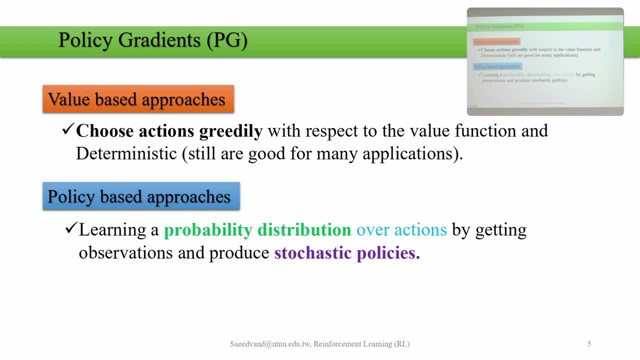 That this can happen by getting the observation produced by the statistic policies. So what does it mean? You should think about this now to understand what is happening. I'll give you some time. Probability distribution over actions. So we have number of actions. 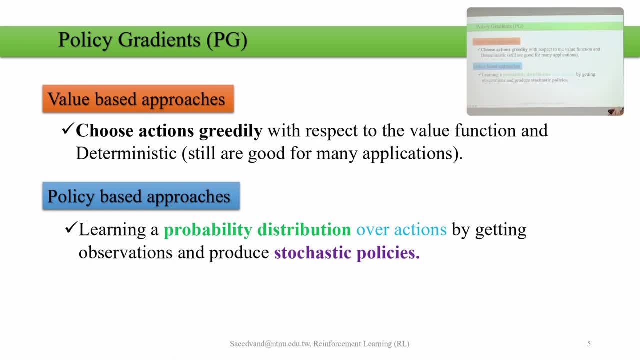 We want to talk about probability distribution over actions. What was happening last, last week in deep reinforcement learning? we were bringing everything to form of probability as output of the neural network. Now we want to always bring everything on the form of probability distribution over actions. 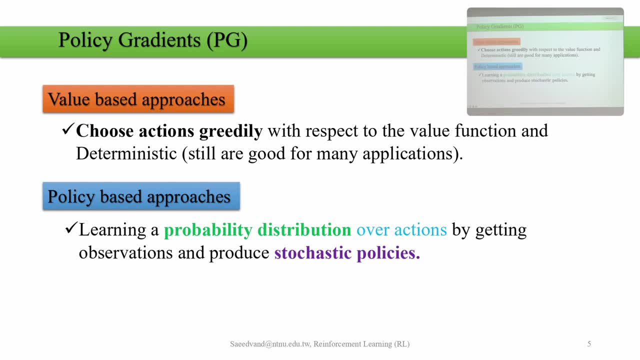 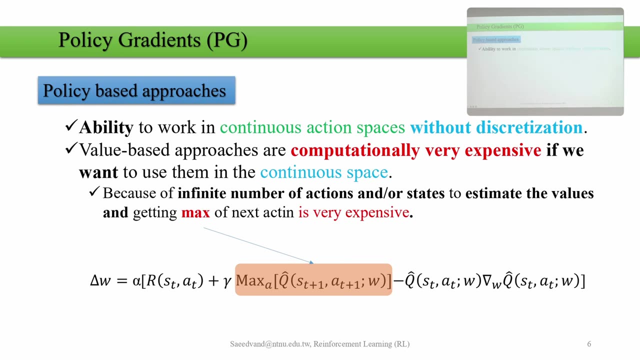 And we are. we are getting observation and produce statistic policies. That that you know now what is the statistic and deterministic means that we discussed at the starting of the course this semester. So by looking at this we can say we have ability to. 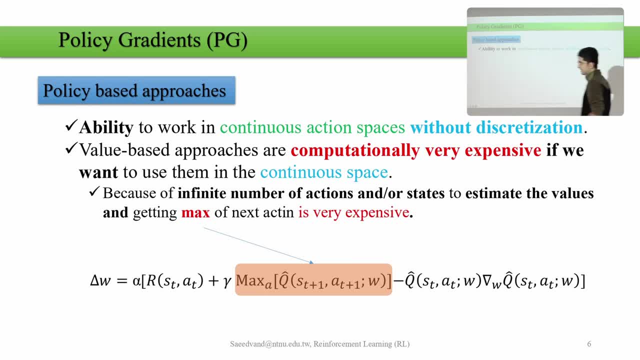 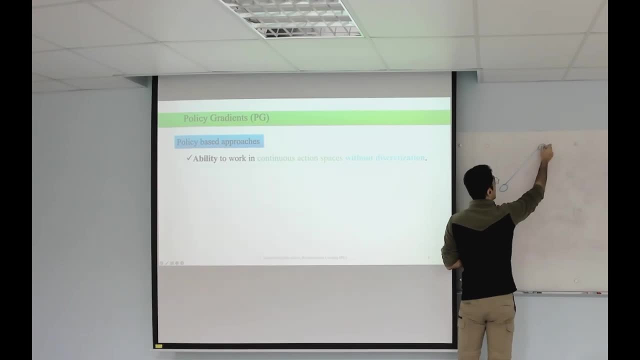 work in continuous action space without this criticisation. So it means that if you have a robot, for example, that this robot has like joints and gripper, in this case, what we were telling? okay, we were saying that this, this revolute joint, can have like 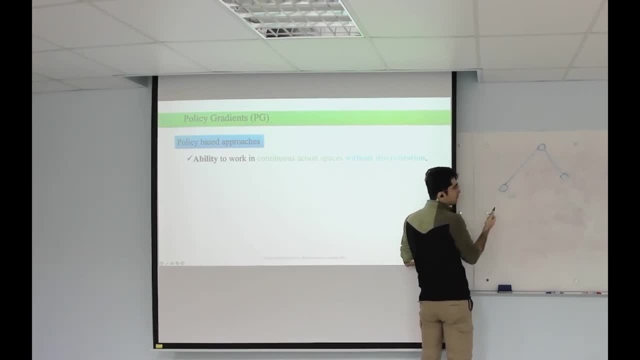 360 degree of rotation, for example, then if I want to discriticise it, I can. I can define the action of this one in range of, for example, zero and 360 degrees, And for only this joint I have. 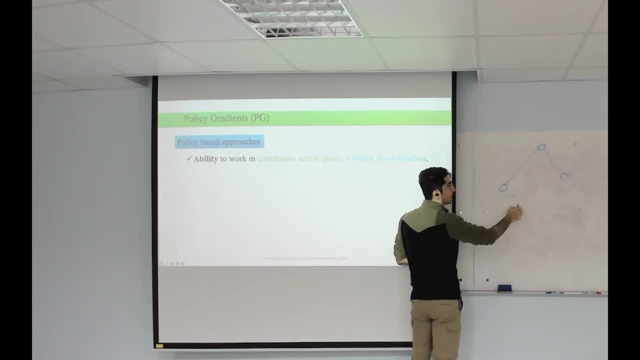 if I also have one one resolution per degree, I have 360. And what if? for this joint, if it's the same, then 360 times 360, if I want to discriticise it times, for example, if I have like something similar here too. 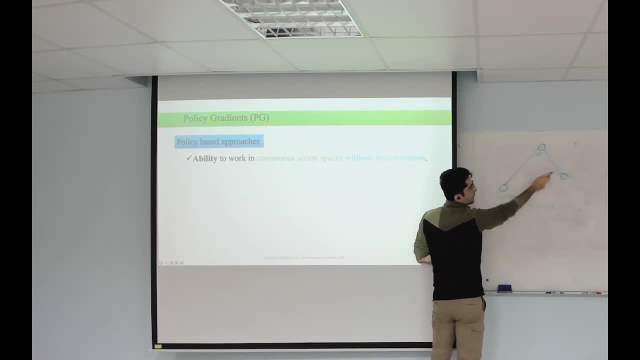 you have the revolute joint that can can be can. we can make it a linear movement by some mechanical components, Like we have again, maybe 360 degrees there too. So you see that the state, the action space can grow exponentially. 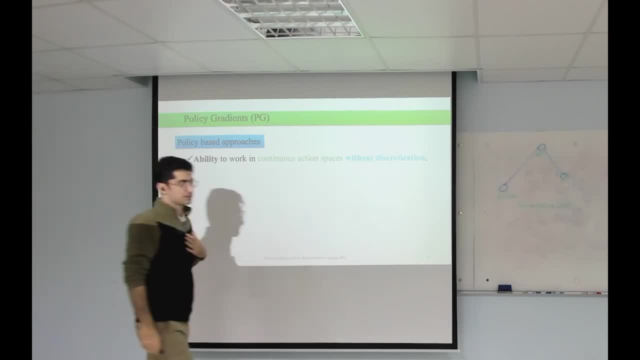 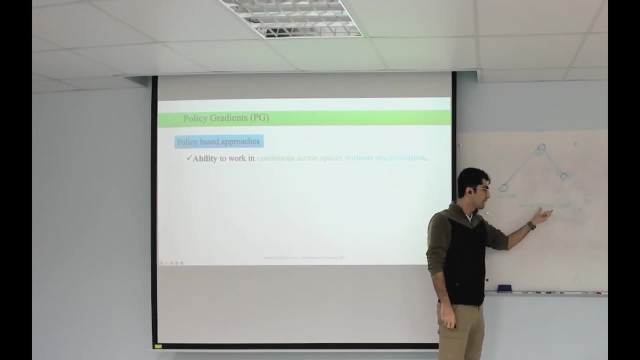 But in continuous form. that also we will discuss it. we will see that. okay, instead of talking about discriti action, discriti actions, we can talk about continuous form of representation of these actions. so that policy gradient is the best option to. 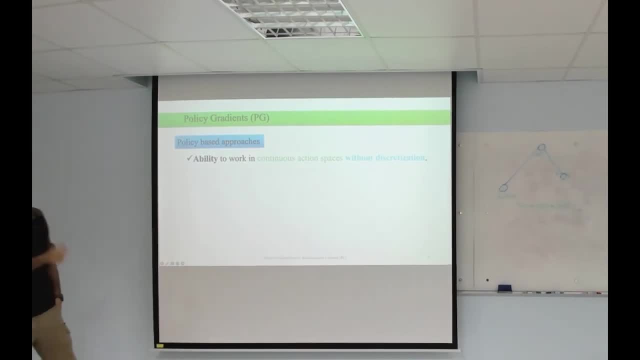 to help us to solve it, That, that that basically the general idea is finding gradient of the change of the policy. That we will see how. So we will try to change the policy from one action to another action. It still can be discriti. 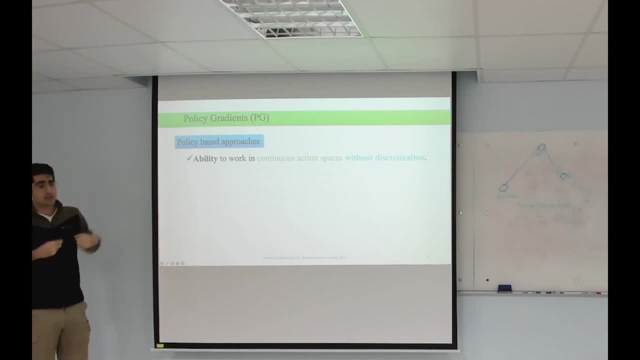 or or continuous form. But. but we will see how we can calculate the gradient and how, in continuous form, we can use it. So we say value-based approaches are computationally very expensive if you want to use them in continuous space. Why. 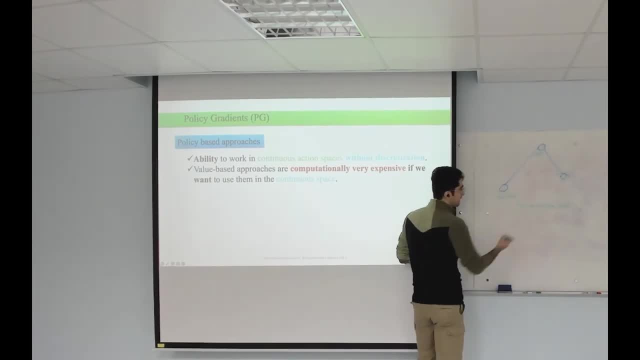 Because now I said I just criticized this. Whatever it is, I can calculate the value function, But what if these are like infinity numbers or continuous form of, for example, 360 times the resolution that I have in, for example? 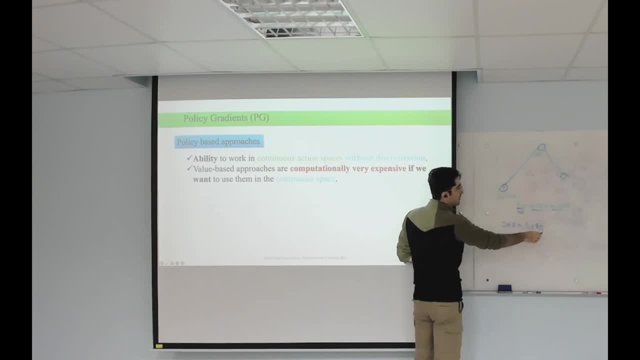 dynamic cell motor 28,. I think Then each one of these will be, will be growing again, even in discriti form or in. if you consider it in continuous form with with continuous calculations, then then if you want to calculate the value base, 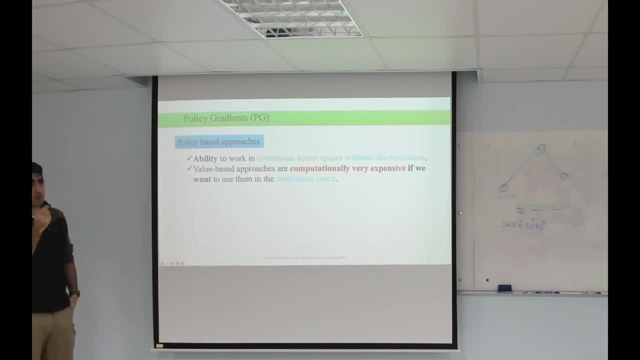 the value function, it will be very computationally expensive. Why? Because of the, the equation that we calculated. If you look at the previous equation that we've learned to calculate with the learning concept, we had a part that in this part 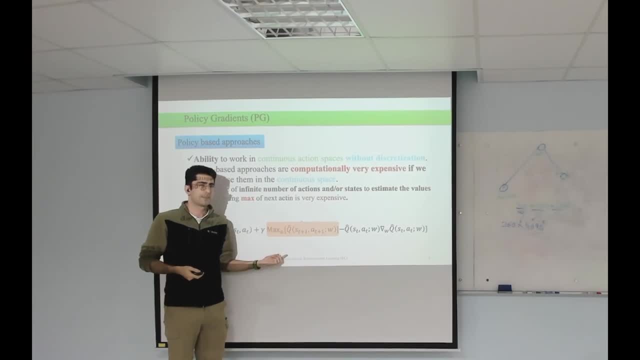 we were getting the max of the next action. And getting of the max of the next action means that I need to know all individual action: next action, possible action, then get the maximum, Although it's coming from neural network. So when you know this, 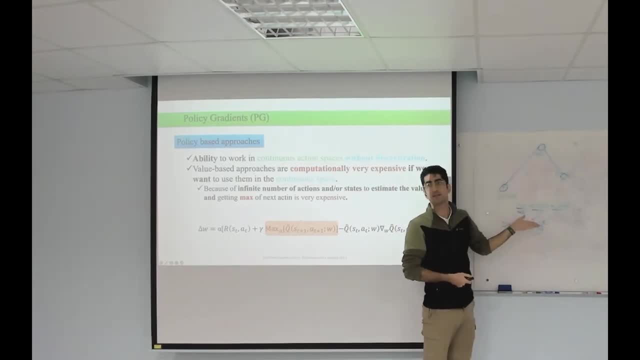 it means that you need to know all these possibilities And just if you want to get the max of all these possibilities, just one iteration is very expensive. If it's continuous also, Then you have something like near to infinity number of the action space. 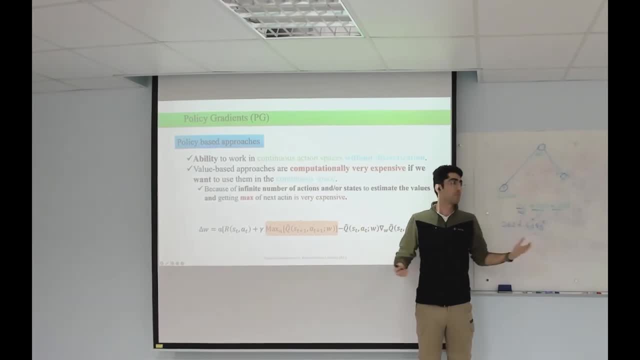 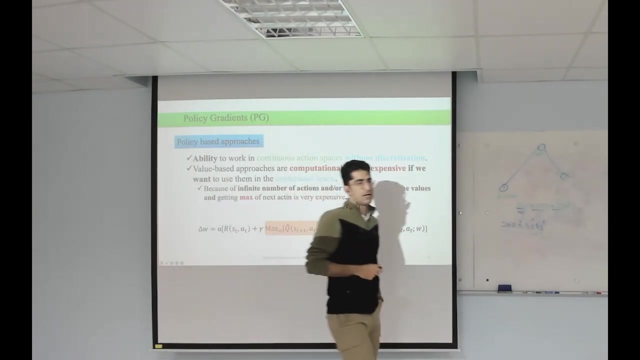 then you want to get the max of that. That's why. that's why we say that. we say that we want to kind of see how, with policy gradients, we can replace this part, get rid of this part, to to update the. 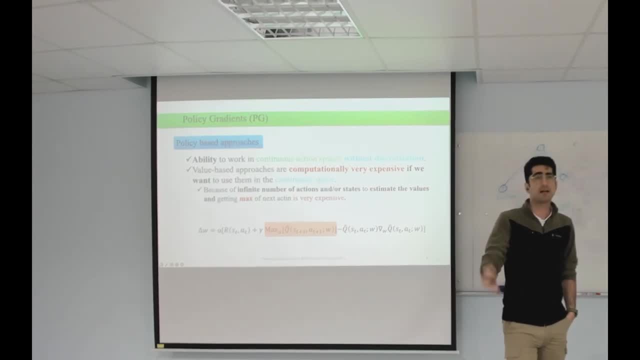 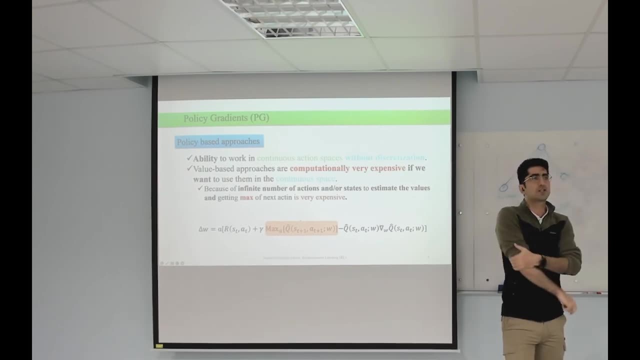 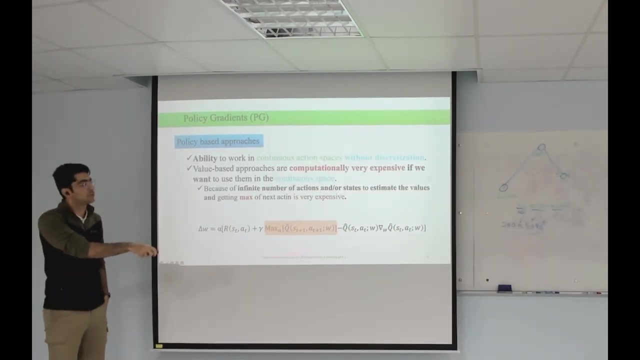 the policy, to update the value. to update the policy by the network, by some parameterized value, directly, not use the value function anymore. So here we have this, the action value. We could have like have the techniques that has directly, just using the value. 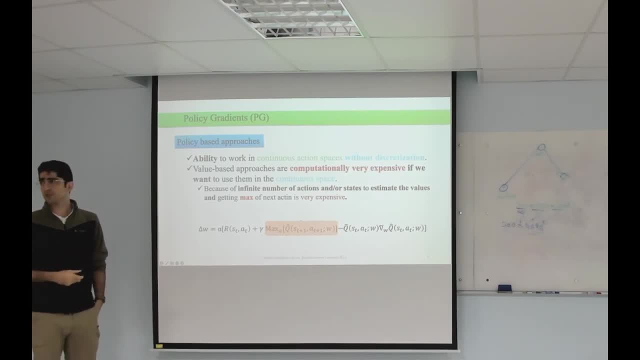 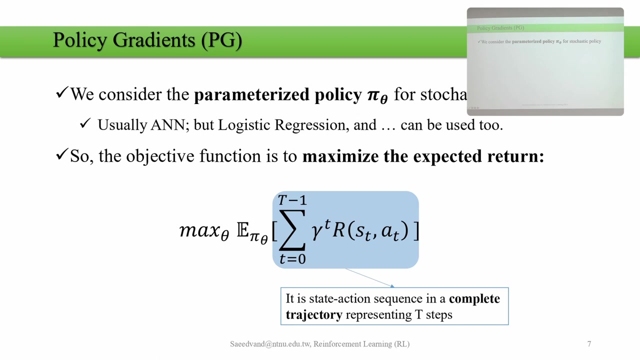 state value. So is it clear so far For everybody. So you need to know what's the problem that we are going to solve. The problem is over here With the value based approaches, especially for continuous action space, or can be continuous observation- to state space. 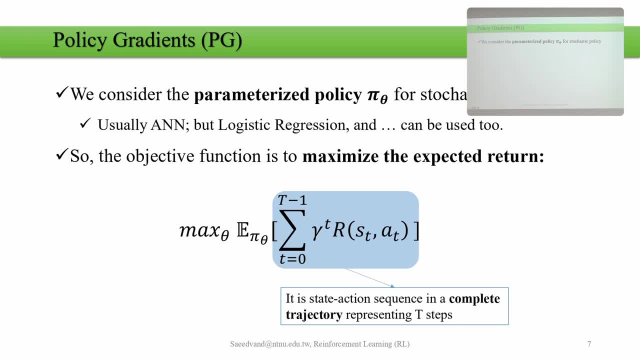 So let's see, start to gradually see what we can do. We say we consider parameterized policy- pi for a statistic policy- as pi theta, that this theta is parameterized value for us, for the network, the same same definition that we already have had for. 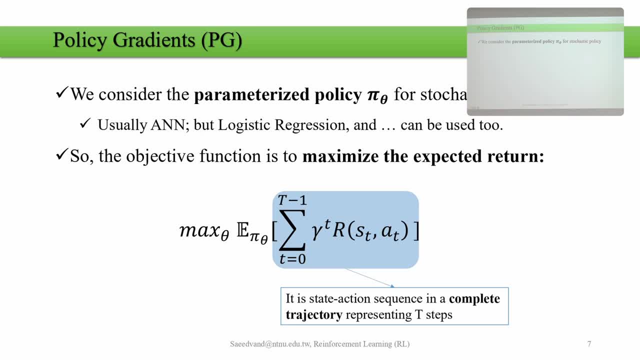 for deep learning Parameters, theta that we want to find, to optimize, to find the best policy that we have. So usually what we use there, we usually use artificial neural network, but we are not limited to that. We can use, for example, 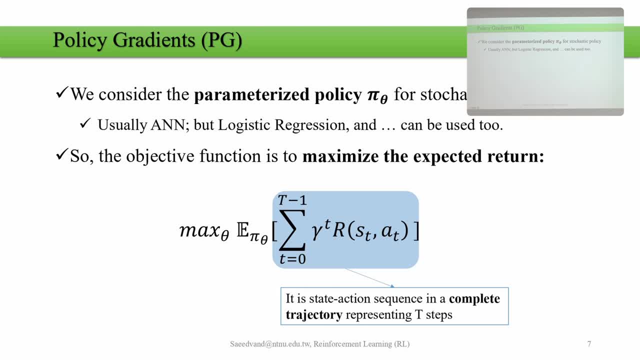 logistic regression. If you are familiar with you can formalize it. write some equations that do something similar to artificial neural network. especially if your problem is small and your action space is small, you can directly use it and you don't need to use a neural network. 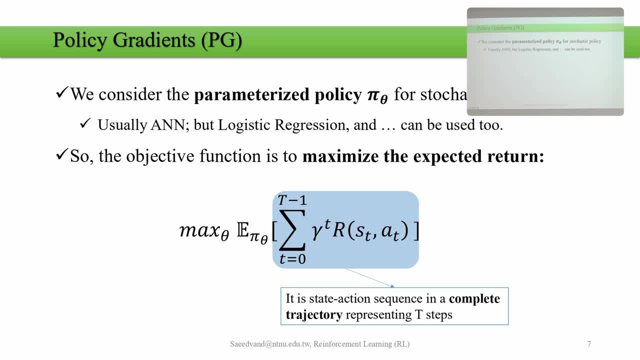 But since now we have libraries, just two lines of code- everybody tries to also use neural network, because here you need to do some math to to do it. So again, the objective function is to maximize expected reward, similar to what we've had already. 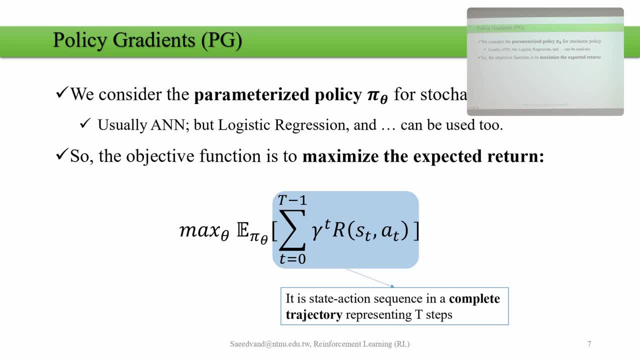 What was the expected reward? We were calculating expectation, So we want to maximize the expectation of the objective function that we have. That if you write the equation it will look like something, something like this equation over here, What we want to do. 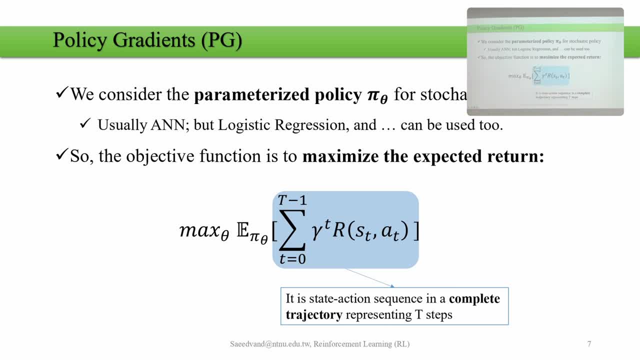 we want to maximize the theta parameters of the expected policy that has the parameters of the neural network that we have, parameters of the value, function, approximation or network that we have. So we want to maximize theta expected policy that contains discounted reward, some of the discounted reward over all trajectory. 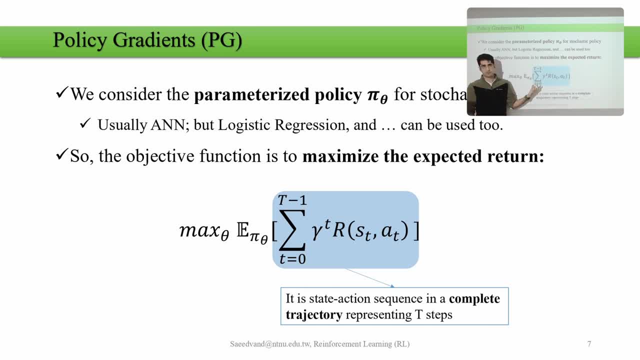 So trajectory means whole episode of one environment. We generate from time zero to time t minus one. We generate a trajectory, for example, robot moves in the environment. Then what we do, we gain some rewards And our objective in policy gradient is maximize theta parameters by expected maximizing this. 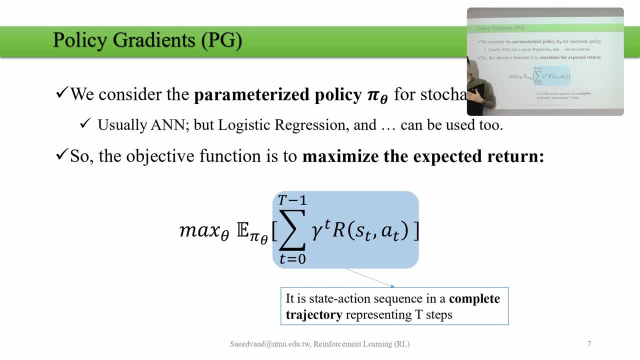 But the problem is, we cannot of course use this equation directly, because we said we want to. we want to work with policy directly and we want to maximize the policy and calculate the policy. We will see how we can convert this equation somehow to bring the policy calculation. 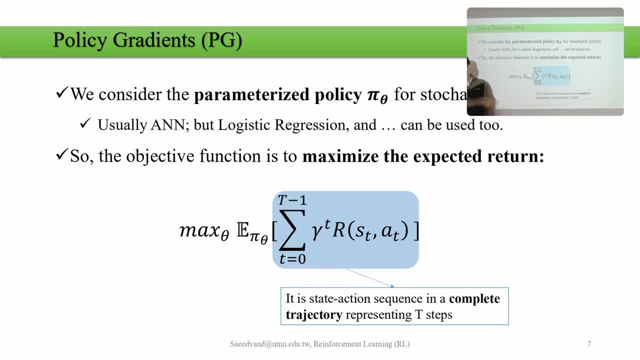 inside calculation of the expectation over here. Is it clear? Any question? If you missed so far, then it will get harder to understand the rest. Make sure that you get the point. So I've written some notes here. It is the state action sequence in complete trajectory. 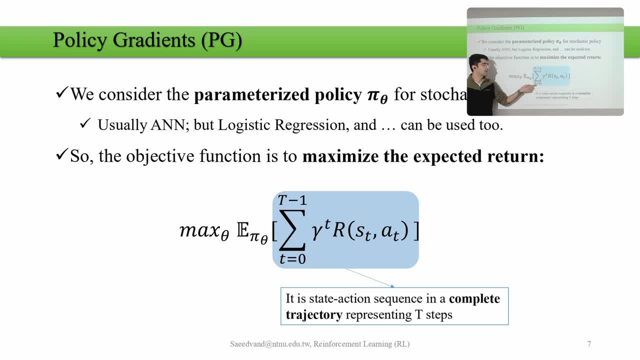 That is represented by t steps. So we have a trajectory. same discounted factor: that we were discounting the reward Already have seen it. We want to calculate the discounted rewards- Some of them are expectation of policy- and maximize the theta parameters on the network. 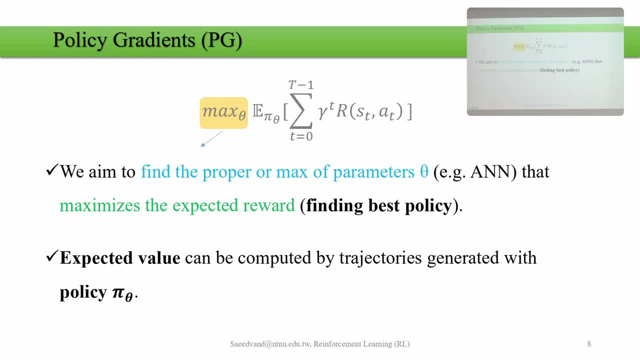 Now this max over? here we are aiming to find the proper maximum parameters. I mentioned to you, For example, our network can do this for us And, as I explained, this maximum expectation should finally result in maximizing the reward that we are collecting. 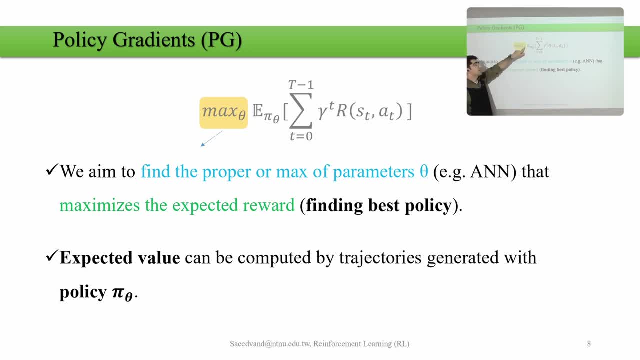 That also, if we do this, if we maximize the policy parameters that maximize reward, we kind of doing improving the policy indirectly, Because if you do this, if you collect more reward, we are optimizing the policy directly- there too right- And finding best parameters to do that. 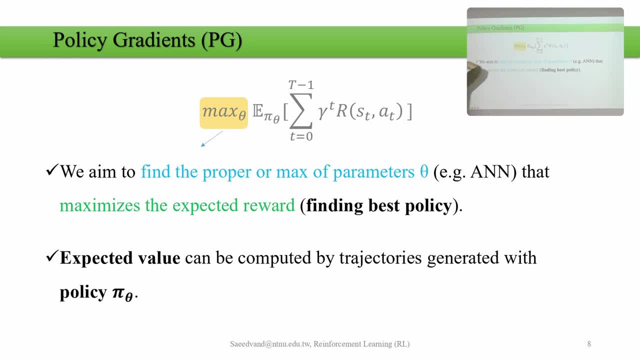 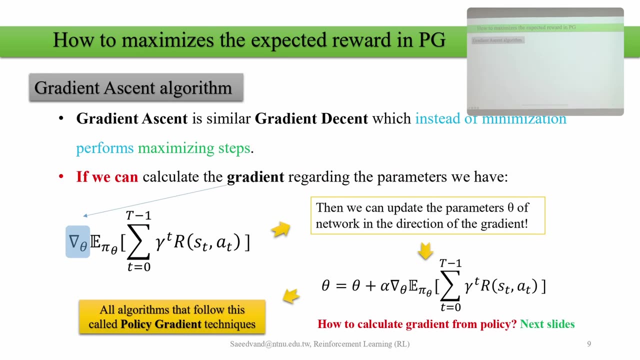 Finding best parameters to collect the rewards that finally give us the policy that we want. So we can say: this expected value can be computed by trajectories generated by policy part that I explained already. Now, before moving forward, we need to have a look at the gradient ascent algorithm. 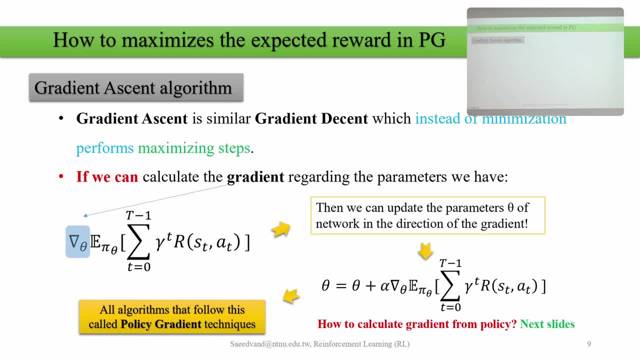 I already explained gradient descent in deep neural network part. You know what is it. now I'm not going to explain it again. But what we are doing in gradient ascent algorithm, we are doing the same, exactly same, but we replace the. 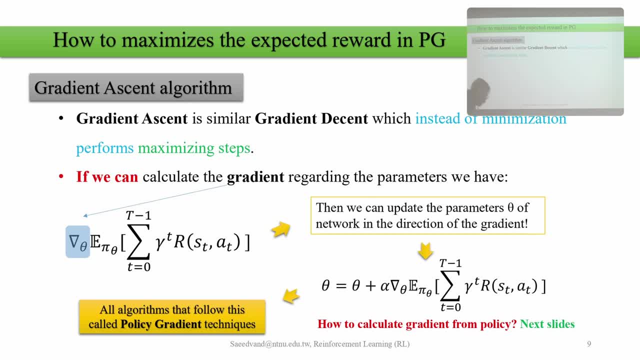 instead of moving downside up to here, we want to move outside up to here. The same scenario. we just want to ascend it. We want to increase the objective that we have. So it is called gradient ascent And policy gradient is using gradient ascent. 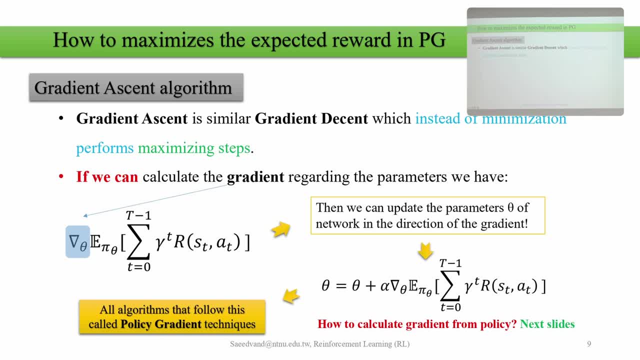 because we want to maximize, not minimize. So now what we want to do, we say, okay, this term over here is the gradient Gradient of the parameters of the expected reward, This gradient ascent. if you remember, we were calculating gradient. 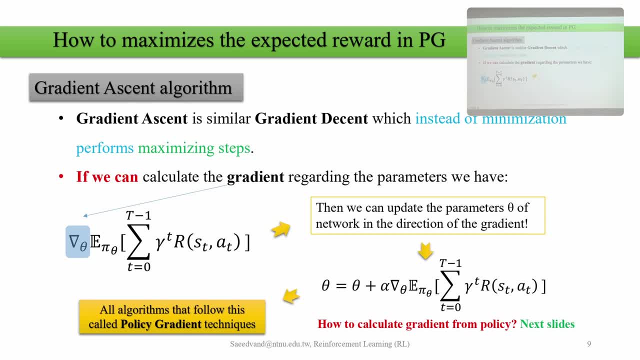 amount of change gradient on the, for example, one function, And we were minimizing Here, we want to maximize it. So if we can calculate the gradient of the expectation of this trajectory, so that we are kind of solving the problem. 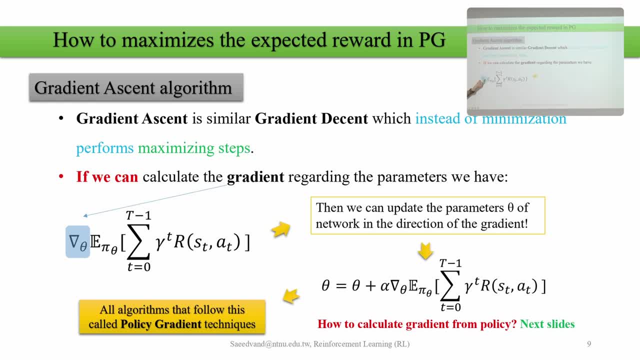 With this gradient, what we can do with this gradient, we can update the weights themselves. So in neural network, in deep learning, what we were doing, we had some weights, We were calculating loss function by calculating some gradient and updating that. 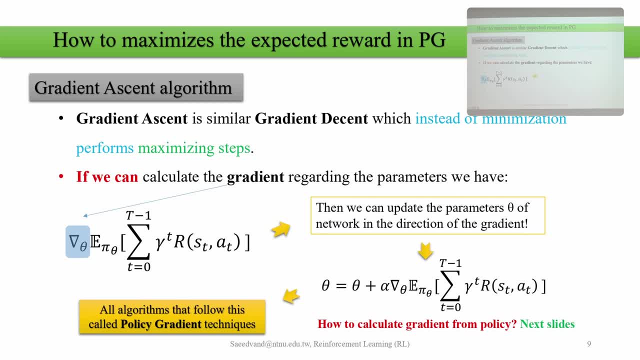 that loss function again. So the idea comes from there that if we can calculate the gradient of this term over here, then we can update the weights of the network that we have. So it kind of improves itself. So I've written the same thing there. 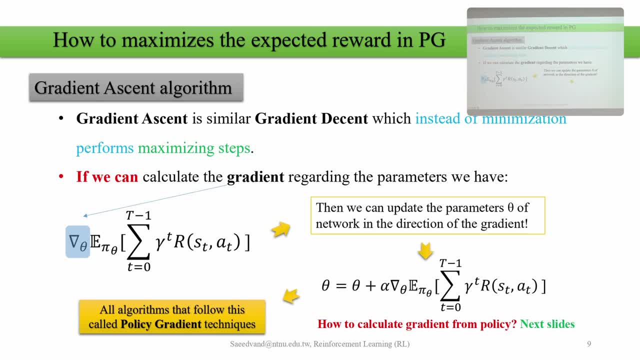 Then we can update the parameters of theta of network in direction of the gradient that we have. And what we can do. we can write theta equal to theta, Since we have gradient ascent added by learning rate, alpha gradient of the expectation of this term over here. 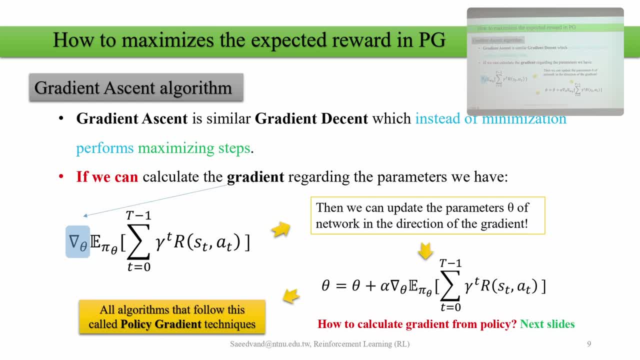 So any questions. so far We haven't talked about the policy calculation and gradient of the policy calculation. We will see that part yet. But here we see that if we can calculate the gradient of this term, we can plug it to this term over here at some learning rate of gradient. 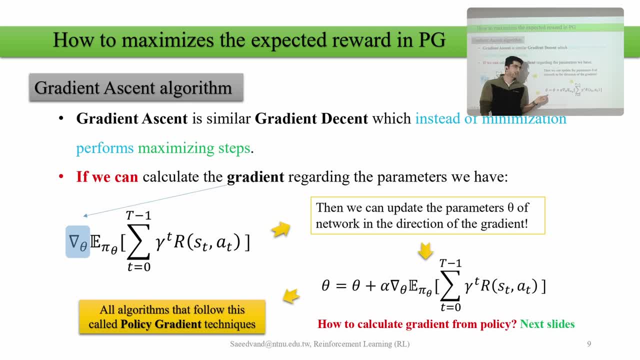 and update our network. weights itself based on gradient and learning rate. So we have neural network. It needs the calculation of the weights. These weights can be calculated by adding each time the learning rate- how much I want to improve it- and the gradient of the trajectories. expected reward. 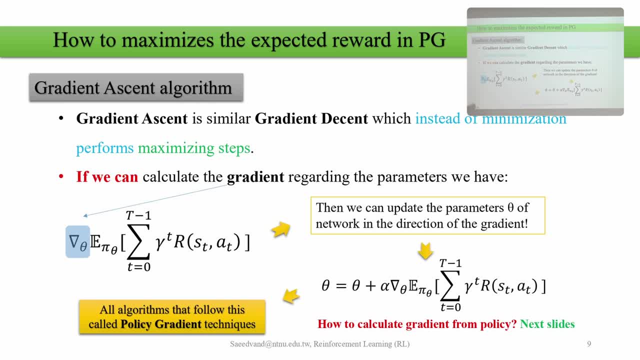 We will see that also, we can change this part a lot. We can. instead of having trajectory, we can use, for example, TD. We can use advantage. We can use different techniques over there That can be replaceable. We will get to that. 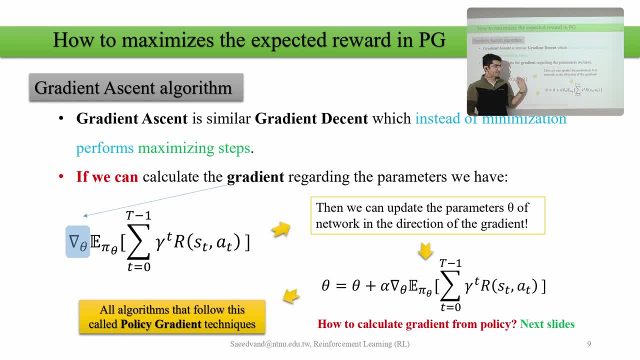 We will get to that part soon, But the whole gradient descent idea should be following this part: Gradient ascent, not descent. Gradient ascent and policy gradient. So I have an important golden point here that all the algorithms that follow this update rule are called policy gradient techniques. 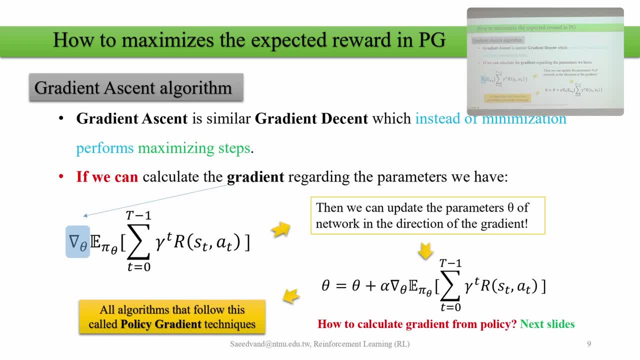 All the family in the graph on the tree that I showed you, All those family that are trying to do this scenario will call policy gradient. But the major difference is over here and how we can update and how we can like kind of apply limitations or control the speed of convergence there. 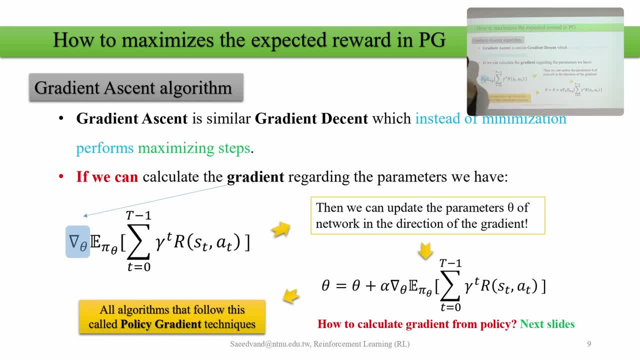 or whatever you're playing. mostly is over that part, But because of that, understanding this part to these slides, to this slide, is crucial. Clear Question. Okay, Now the question is how to calculate gradient from policy. So this is not easy at all. 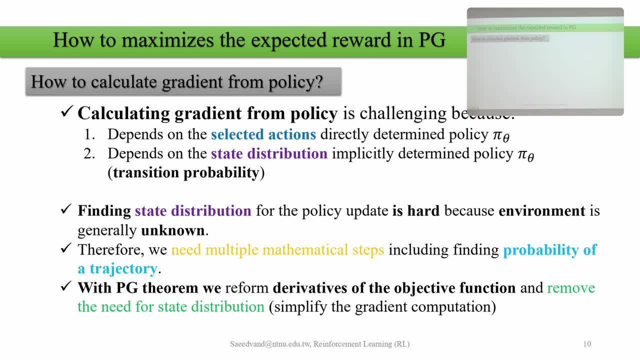 And If you want to answer that, we say we need to calculating gradient. gradient policy. that is challenging. It depends on the selected actions directly determine the policy pi. So this policy pi with parameters theta is actually is a network, neural network or deep network. 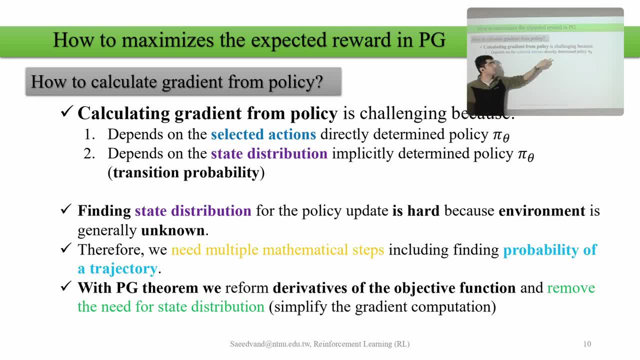 that generates one policy for me, right, And this, this, this policy- pi Is kind of- depends on the selected actions that I have, And also not only that one, but also it depends on the state distribution or transition probability that I have. 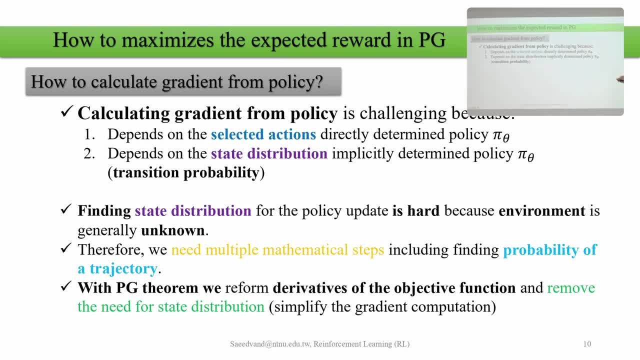 That that these two together, that also transition probability or state distribution, comes from the policy pi that the same network is trying to give me. what is the policy At the beginning? of course terrible policy, something random. But we want to kind of adjust those parameters to. 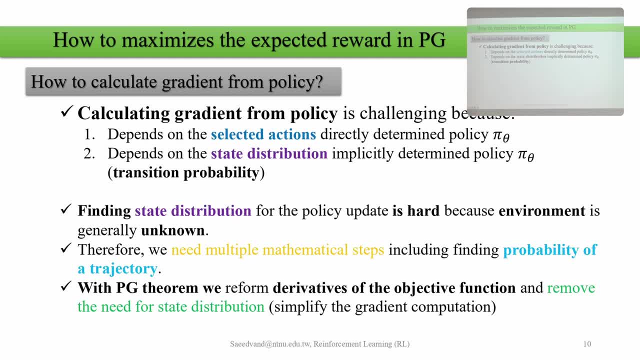 to take up parameters in order to maximize the reward, in order to learn what to do- Agents learn what to do- So that these two elements are important parameters that we want to see how to deal with it and how policy gradient can solve our problem. 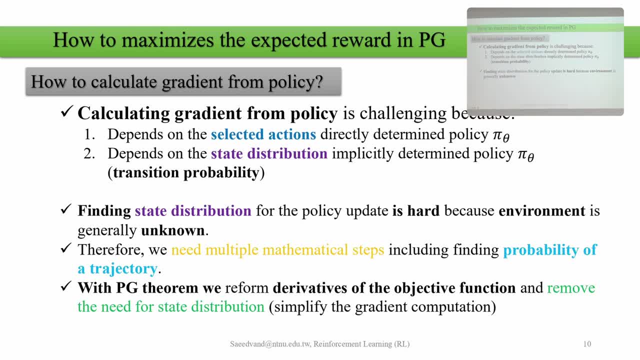 Therefore we say: finding state distribution for the, for the policy, is very hard If, if environment is unknown. first of all, what does it mean? It means that for the selected action part: okay, we can, we can say we are trying to select actions by the policy that we have. 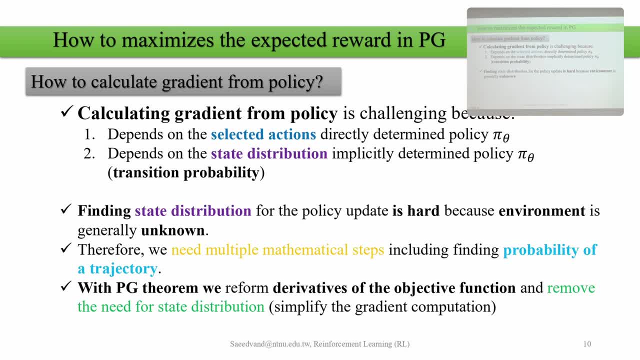 We, we can figure it out, But what about the state distribution? We don't know. In some techniques we discussed together, I gave you, for example, in the example, this is 0.7,. this is 0.3,. 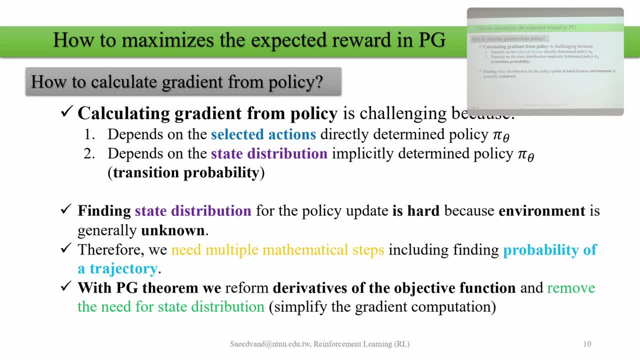 probability of the actions that can happen in the environment. Do we know that? We don't know that. Since we don't know that, we want to see, okay, actually, how policy gradient is working and how trying to play with these values. 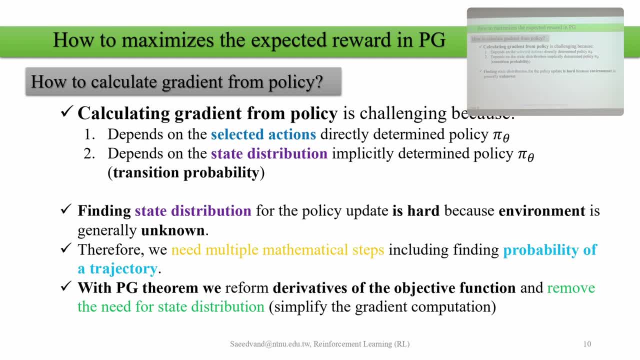 with the state distribution in order to state probability distribution, in order to solve the problem. So now we need to apply some mathematical calculations in order to bring the probability of the trajectory and the policy inside the game. And and since, since we want to calculate the differences of the two policies, 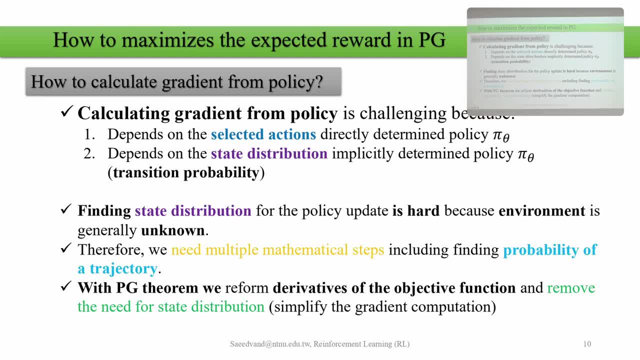 and find the gradient. we need to use some policy gradient theorems that drives the objective, functions and and and kind of. we have to remove this state distribution from from directly calculating the objective, since we don't have it. So 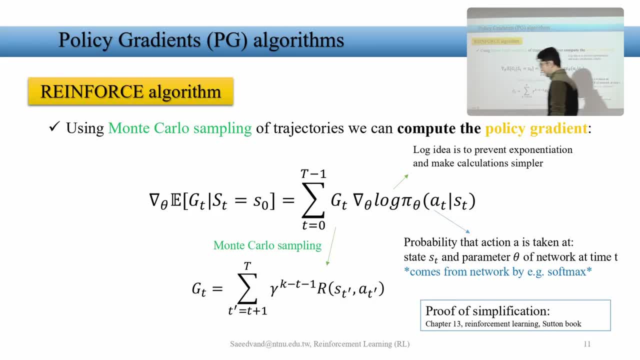 how this can happen. I'm going directly to the slide. So this term over here comes from the equation, from policy gradient that I showed you: The sum of the expected sum of the discounted reward that we've seen From there to come here. 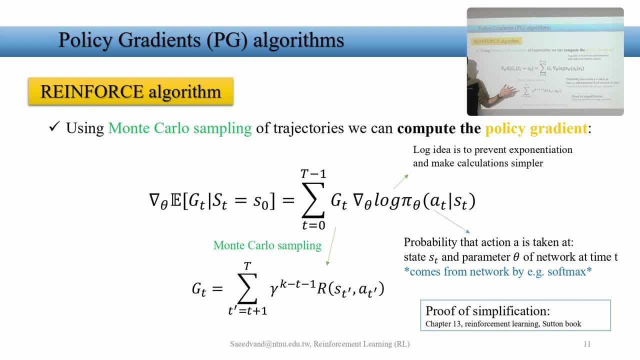 we have like two, three pages of math. I'm ignoring that, I'm letting for you to study it yourself. But finally, after doing all calculations, I I think it's not necessary to know how that's happening, but you can have a look. 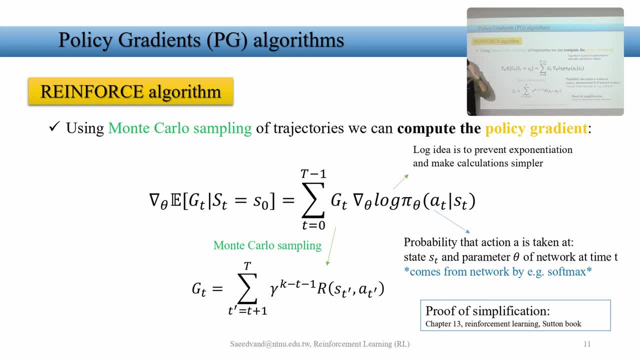 I put the reference that you can have a look at chapter 13 of the book, how the drive derivatives comes, how we can remove that transition probability. Lots of mathematical knowledge requires, But finally we are. we are this this term over here. 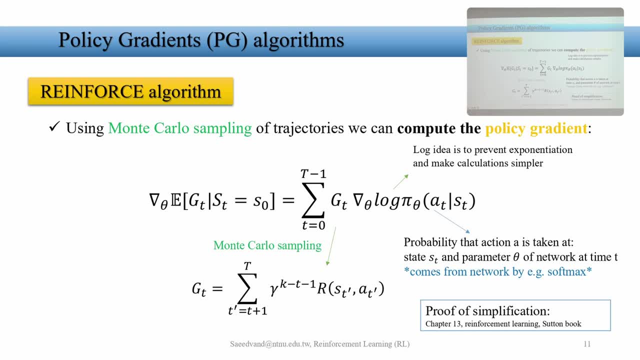 but let's see how it looked like and what is it doing. We say, okay, we are using similarly as previous set that we have, we have the trajectory And if you have using that trajectory in one episode we are actually using Monte Carlo, sampling that. 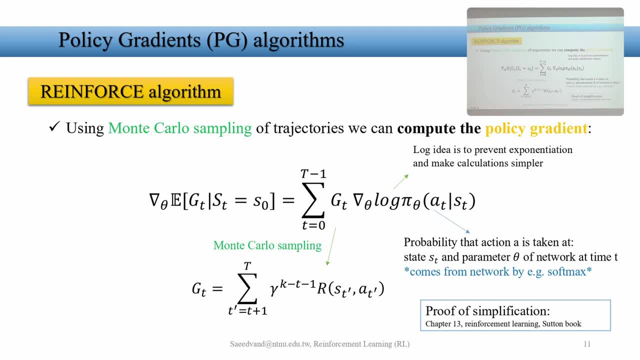 that we were in Monte Carlo sampling what we were doing. If you remember, we were creating trajectory in the environment at the beginning. random, because policy is random Then then try to compute the policy gradient, like this equation, How that is happening. 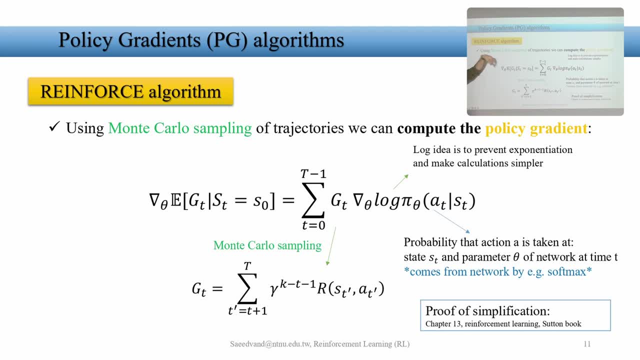 If we use the equation in this form, we call the algorithm as reinforced algorithm. And let's see what is happening. We are calculating the gradient of the parameters that are on the network. Again, that is expected. GT. GT was returned, If you remember. 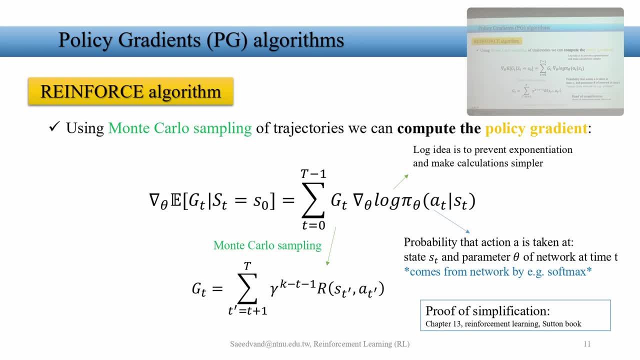 we've seen how to calculate the return. but GT also, I stated over here, GT is equal to some of the, some of the, the trajectory, the trajectory that we have by discounted reward of the next state and actions. So this was the return that we always 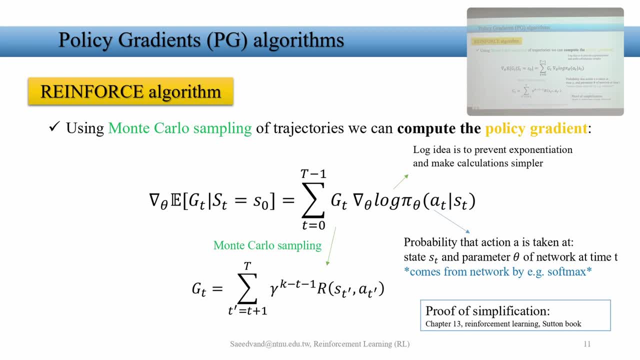 a couple of times in different algorithms we defined as GT. Then what we do? GT given by state T. state T, for example, starting point, is equal to some of the this return GT times gradient of the logarithm of the policy pi that represent state and action. 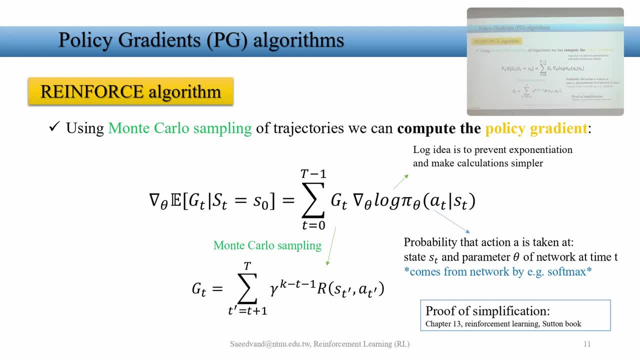 So what does it mean? First of all, the logarithm over here. where is it coming? We didn't have it over there. The idea is just preventing exponential calculations, that the numbers are growing, just taking it, taking them down. Nothing very complex. 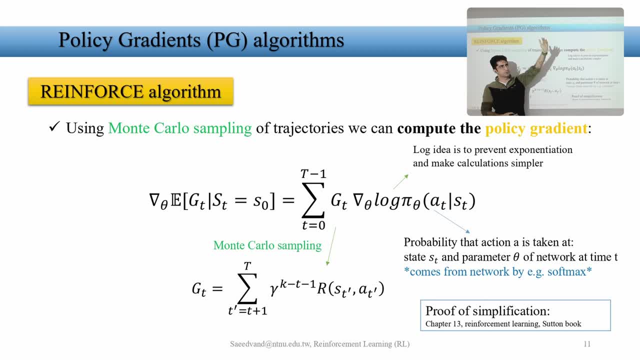 We just want to bring the value down. Bring the values. If you get the logarithm, the values are bigger. We bring the scaling and making them as a smaller values. But here we have the probability that action A taken at state S with the parameter theta of the network. 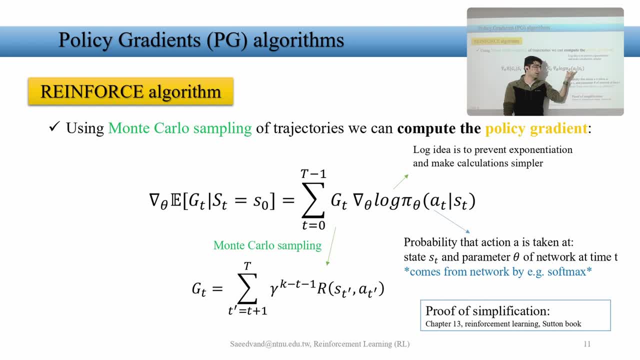 That actually this policy pi I mentioned to you, we have a probability distribution, So that, so that our network, our network output should be something right, That something shows the probability distribution, that, for example, can be softmax, So that the policy parameters theta. 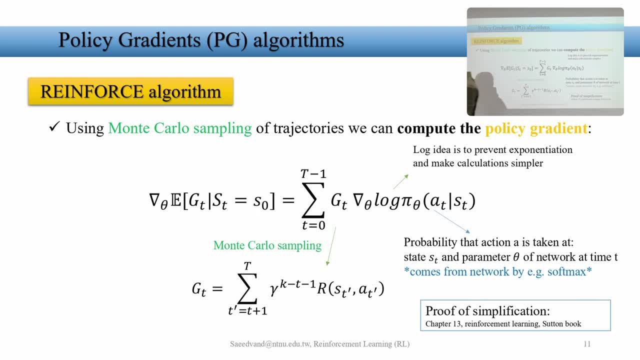 action given by state gives us the probability of the occurring occurring that that action in one particular state. So maybe it looks a little bit complex, but but actually it is not, because here we have the probability of the one action that is occurring, based on the softmax output. 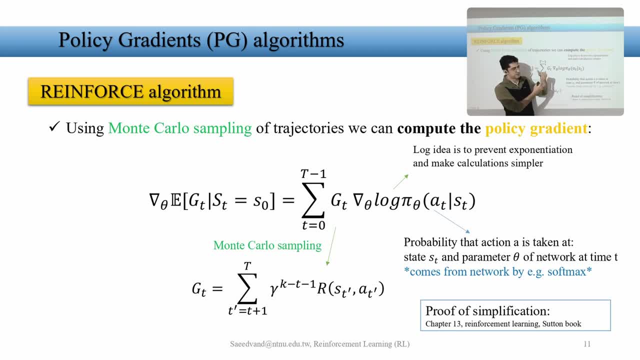 What we were doing. what was doing softmax? softmax, we're converting output of the data network to probability forms, That's saying what is the probability of each one. And we consider that probability as output of softmax, in form of probability of each action occurring in. 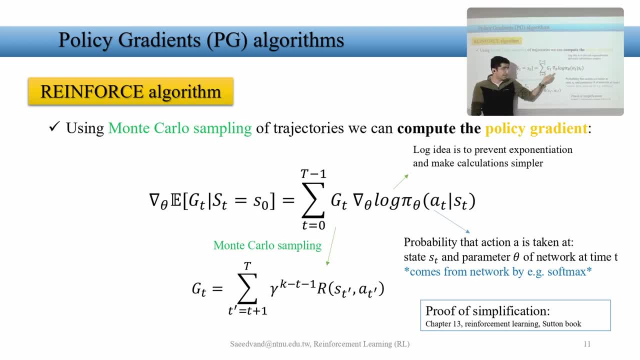 in one state, Then calculate the, calculate the gradient of the logarithm of that probability, Then multiply that by GT discounted reward, Then we can calculate the expected reward of gradient descent algorithm that we have. Question, any question. So I'm using all the terms that we studied during course. 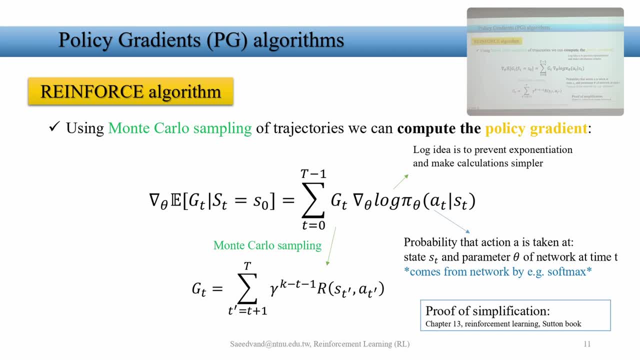 If you forget some, then you're missing some, some, some parts. We have to, So all the terms that we've used like, like return, the probability, distribution of the actions and and all the things we have to use it here. 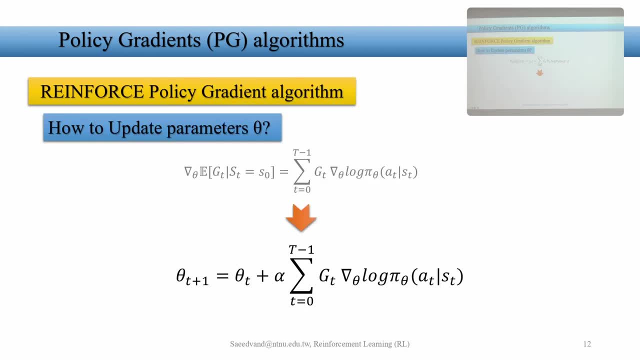 Okay, Then what we need to do? simply look at. look at what's happening. We've got objective function. I can now update the same This: this policy pi comes from network in the left side. This policy pi, the parameter theta, can be updated by this term. 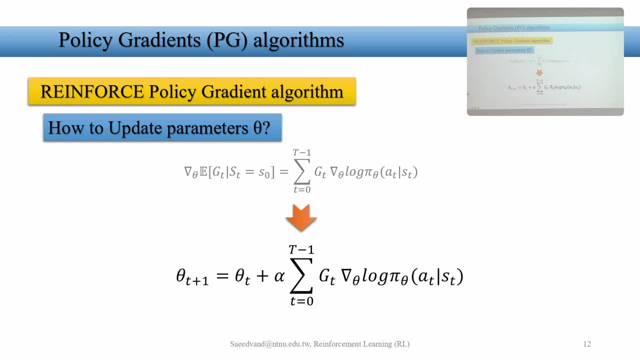 The theta key added by one update of weights of the network is equal to uh current rates of the network added by learning rate of the whatever. whatever learning rate should be times some of the discounted reward added by the same term gradient of the logarithm of the probabilities that is coming from network. 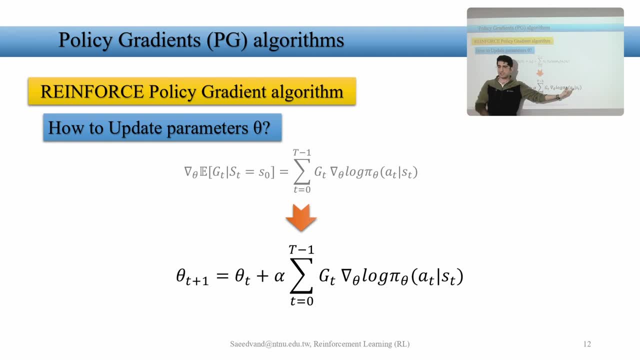 So we ask: network, what is the probability of this action that is occurring? Then times it to the return. to sum up the return in this reinforced algorithm, then apply the learning rate and update our weights. I think this is the most clear thing that we can understand policy gradients. 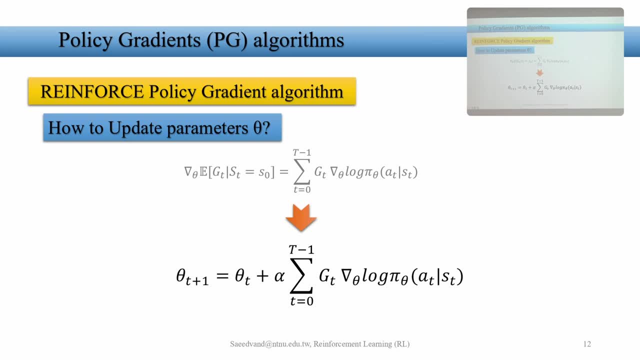 The network output in the form of probability, calculate the gradient, then adding learning rate, then adding by updating our uh weights of the network. It's kind of asking network and updating itself And why? why we can update itself correctly because of this GT. 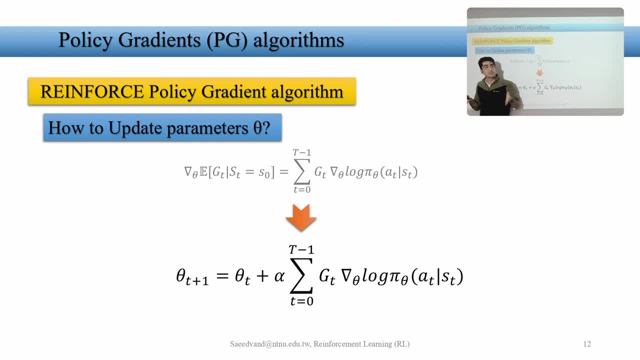 that GT is calculating discounted return, discounted reward for us, And this part over here is kind of feedback from environment. that this feedback from environment times the, the probability and the output from the network with some gradient can help us to update the parameters. 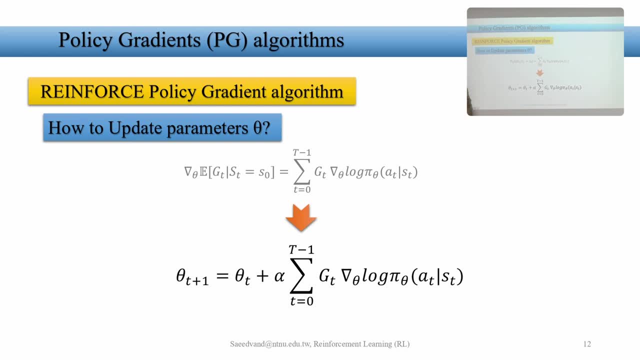 Of network itself, Kind of we are up, we have the policy gradient brings the benefits of the updating neural network That was updating theta into the game directly, into the equation directly. So merge the neural network update of the parameter theta into the 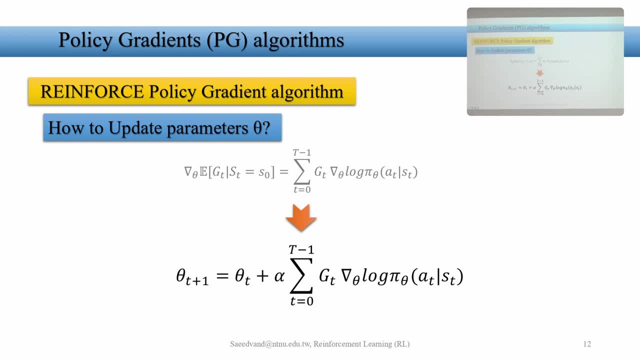 also uh, the uh, the calculating the uh and the policy and bring it uh to to understand what's happening. Okay, This, this equation, has different representation in the different resources. You may, uh, you may need to a little bit study. 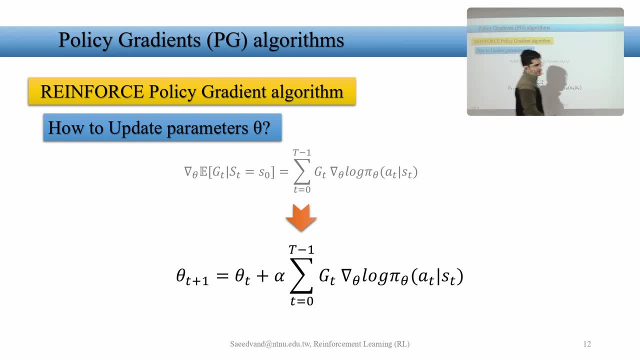 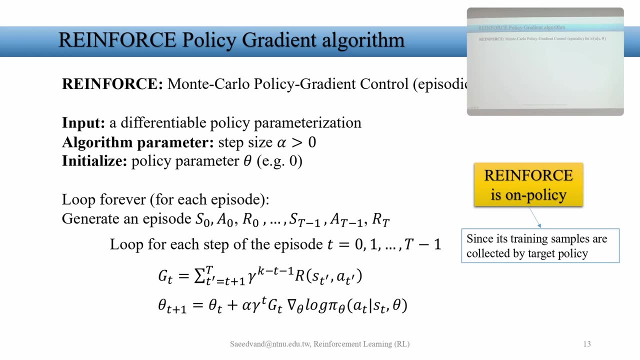 You may. you may need to be careful to see uh, because I see more than 10 different uh. uh form of representation of the uh reinforce algorithm. Now let's see step by step. Oh, okay, First of all, 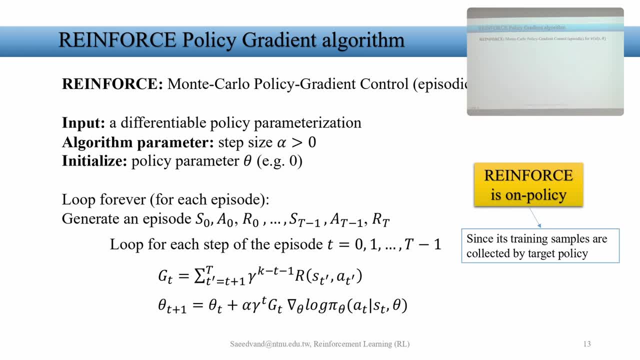 we have Monte Carlo policy gradient control. That is the episodic for policy or policy pies, action given by state and parameter. So here the theta parameters inside here. it could have been here too, It doesn't matter, is the same Representation. 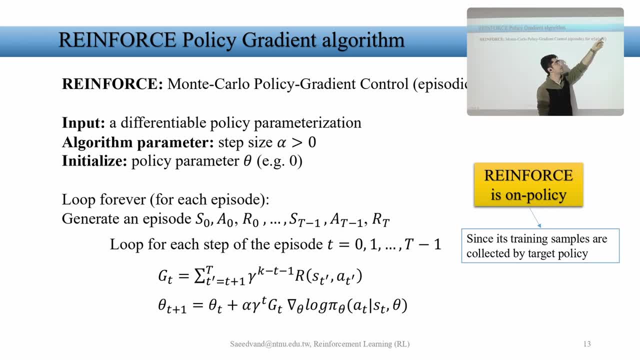 The objective is kind of finding the tetas that maximize action for state Okay. So let's take a look. So first of all, input is a differentiable policy parameters. we need to be careful also that the policy parameters are kind of defined somehow that is differentiable and that. 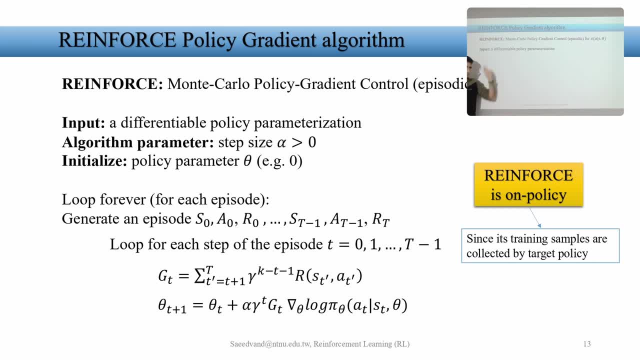 we can calculate the gradient, Mostly we can. but if you define it somehow that you cannot calculate the gradient, or gradient is not existing in some cases, you should reform it, define it somehow. that is always calculatable, Be careful about that. So what is happening there? another parameter: we have algorithm parameters like step size. 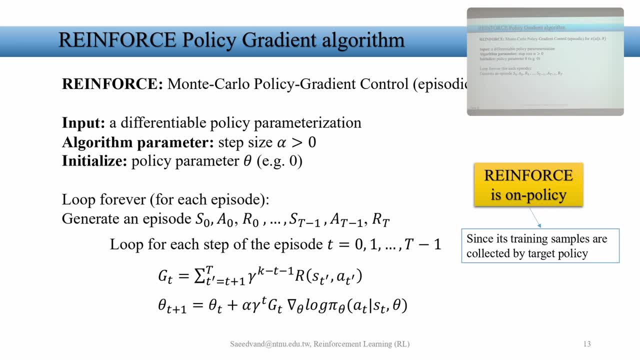 learning rate. alpha, of course, should be greater than zero, otherwise our network won't learn. We have the initialization of the policy parameter, theta, that we have initial weights of network. we have different approaches. for example can be zero or some random weights over there. 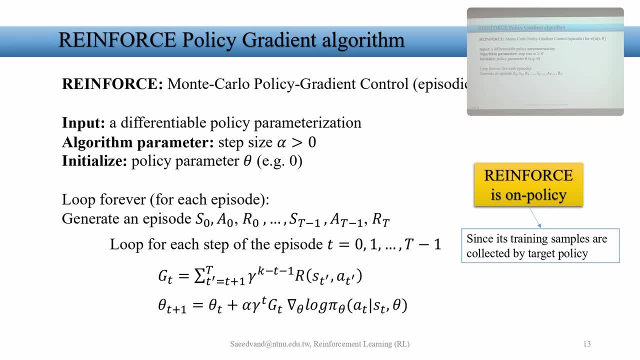 whatever it is, We calculate, we randomize, we initialize, We initialize the parameters, theta over there. And what we do next? first of all, in reinforced algorithm. first of all, we loop forever, or for each episode. So forever means that, like, of course, it's sometimes in some case finish here because 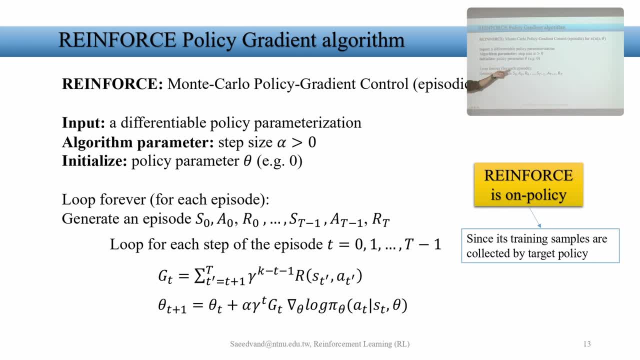 we have control So that when episode ends, that terminates. I mean the episode should end up, It should end up in terminal state somewhere. So we generate episode for that one from state. the pairs of state action. State action- that goes to also reward. 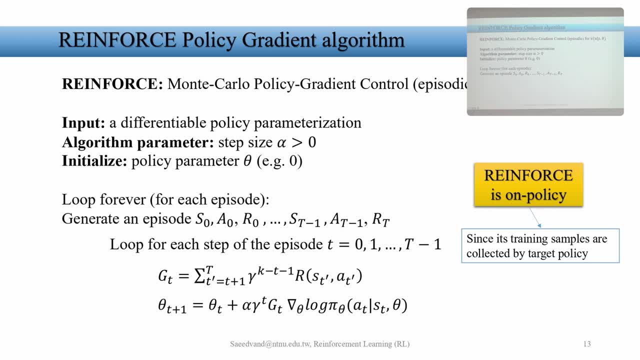 State action reward And finally we have the state action reward. So these three is a pair And these three is the end part, that of course, we have state t minus one, because if its next state is terminal, We already finish it. 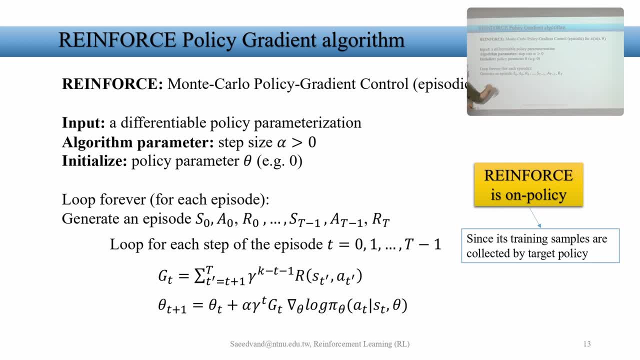 Because of that, we don't need to calculate it again. As you've seen in the examples that we were in the Monte Carlo approaches, we were generating and we were not calculating the end state- Something similar, But reward of t is including that part of this. 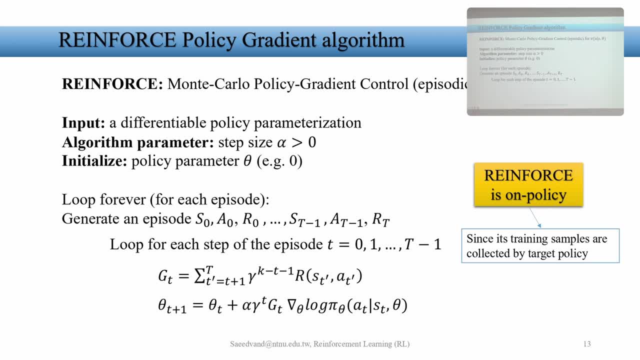 Then after that, after we generate this episode for reinforced algorithm, we loop for each step in the episode that comes from zero to t minus one. We want to, actually we want to- move into the trajectory. That's it, That's we have. 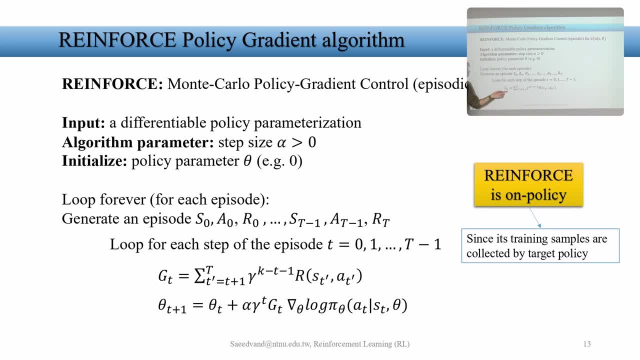 Then what we do? First of all, we calculate the return. GT is discounted. Some of the discounted rewards, The same term that I showed you, Exactly the same thing. On the other hand, we have the up data parameters: Theta, added by one. 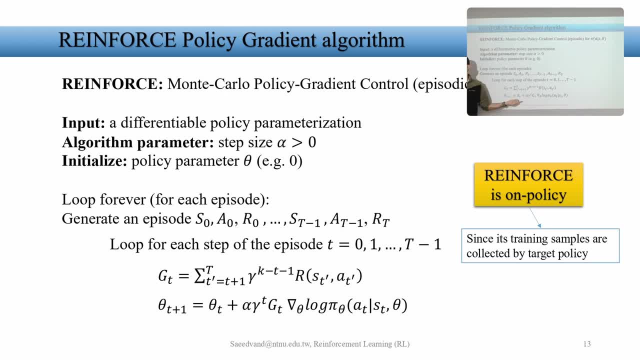 Equal to same parameter again to update the data parameter. So after understanding the mass, the background, you see it. also. the algorithm is pretty simple, That the zd A each time, for each, for each episode and for each step at the episode, we update the. 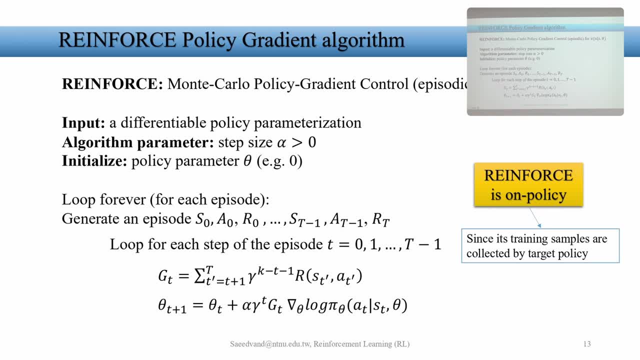 theta parameter, we update the uh weights of our network and how that's coming from that, coming from the calculate on the return. that is sum of the discounted reward based on how, how, based on the trajectory, what you generated. if the trajectory is good, we could get, we, we, we get good return. 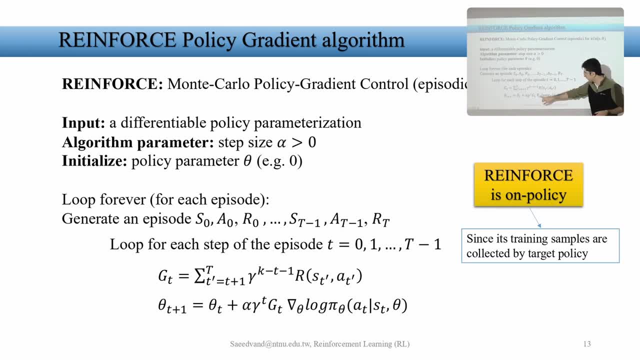 if we get good return, then the gradient of the differences of that, that, that that calculations show that the gradient shows higher amount of change and the change of data, of this data not only by learning rate is, is defined, but also the gradient of the change that they between. 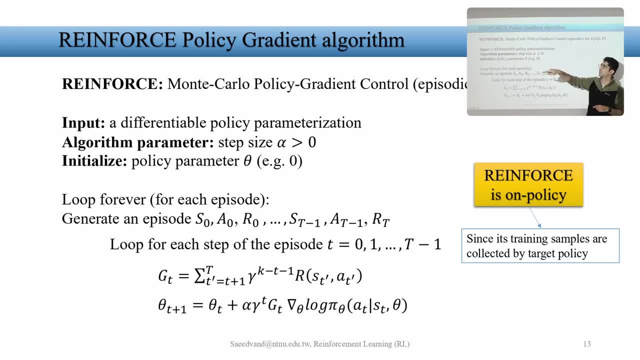 policies and the policy you know. when we calculating the gradient, in certain point we can say how the slope is and if the slope is higher, based on this return, then the theta will be updated faster and our network will move toward learning the collecting more returned by gt that agent is doing in the environment. 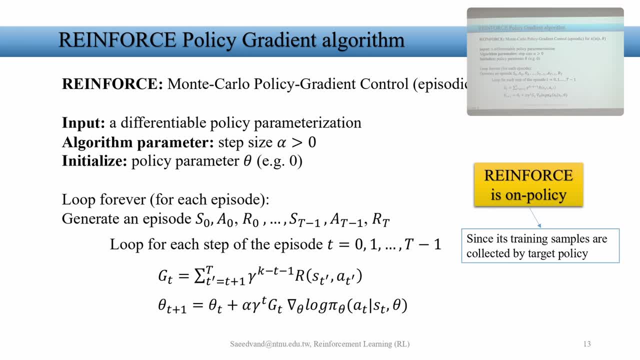 clear. so this is kind of the base of the gradient algorithms. the whatever algorithm we have are kind of trying to follow this concept over here. but but changing this part over there that i will introduce something here. we have a note. we say, uh, reinforces on policy, so why it is on policy? 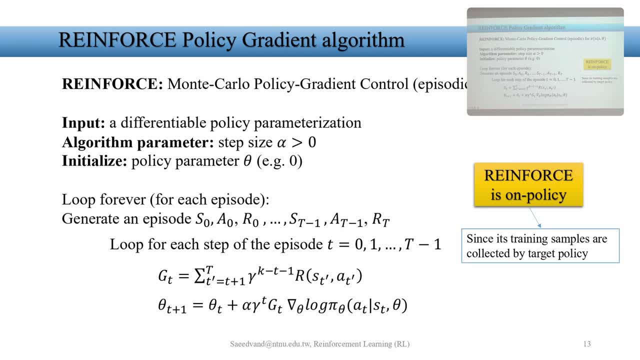 why it is not on policy? because i- i will state it over there- the answer the- the training samples are collected by target policy itself, by the policy that we have same network. so whatever is generated by the policy also has been used to update the data. and if the update step with the action generation step is same, 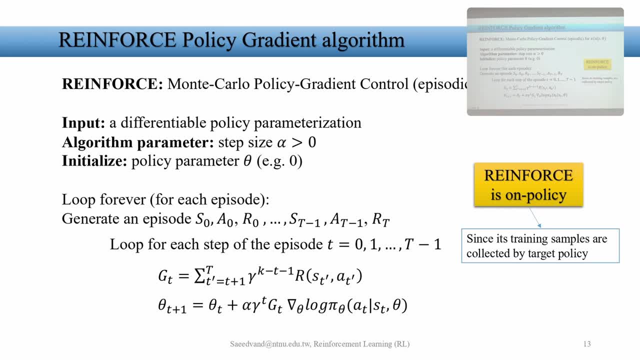 then. then we said this is on policy. if they are different, there are policy, but we are kind of maybe are more interested in if we have the same analysis. i like data very much more similar than the concept. i like to work more closely J manner here here. if we 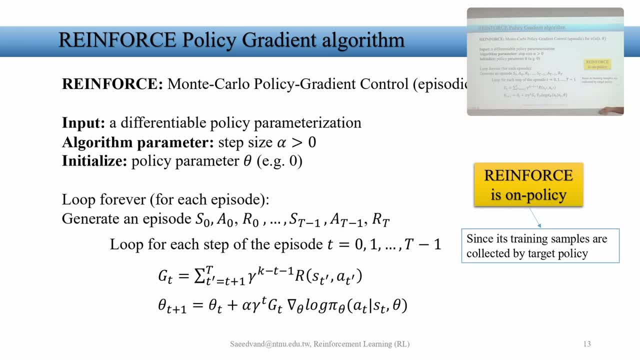 trial, for來說, trying to hear from j as say, unidentified results of as gold. the growth of data will be of principal reduction, as seen while we are collecting window meta samples as scattered pages needed for negotiation, And we will see in the next slide that we have another techniques that are of policy. 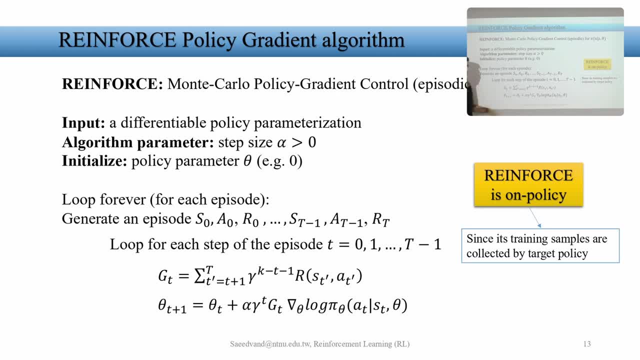 and they are not using same network to do this. because when we are doing like asking same network what to do and updating the weights of same network but what he's saying to do, then these can make on a stability update of the parameters. He's like I'm asking this student over here: Hugo, how are you performing? 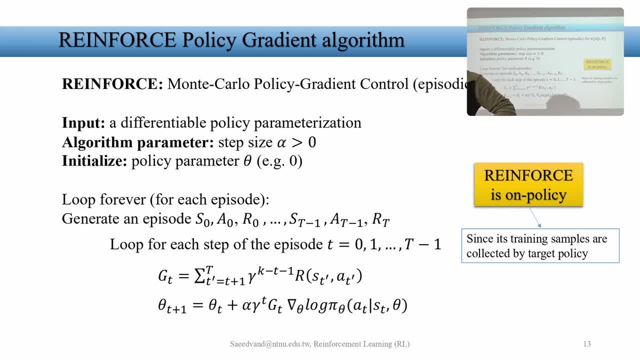 He says: good, good, I'm good. Again, how are you performing? Good, good, I'm good, But we will see that it's not good. I should ask this guy how this guy is performing. Then you see they are fighting against each other. 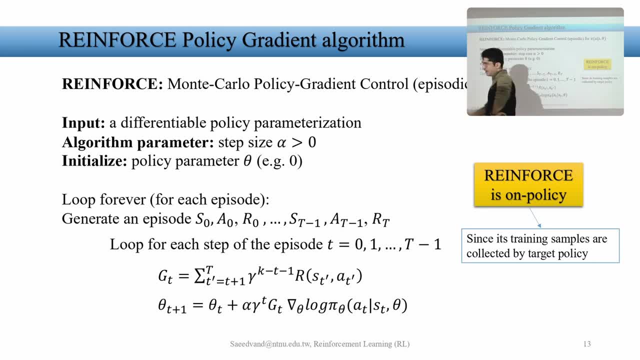 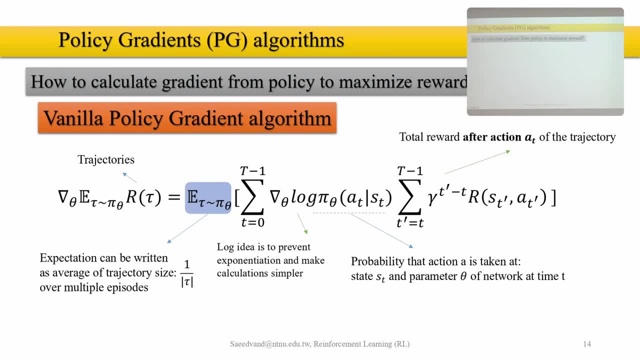 If you say bad, I'll be angry. Yeah, that's the actor critic That we will see, Okay, Okay. So we have a question that we say: now also, let's have a look at how we can calculate the gradient from policy to maximize the reward if we have vanilla policy gradient algorithm. 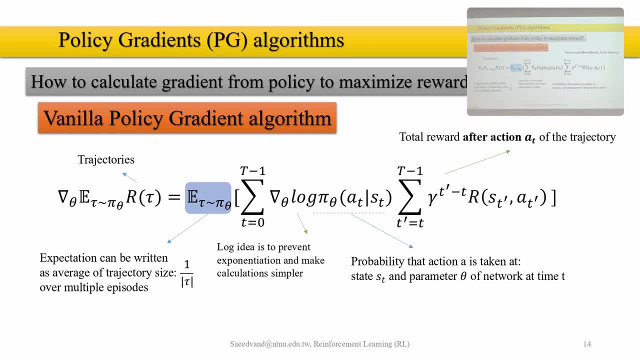 So vanilla policy gradient algorithm is very similar to reinforce, but some slight changes over here. Let's have a look at the term, Let's see what that looks like. So the G, the return that we had there, he replaced by this term over here. that says: 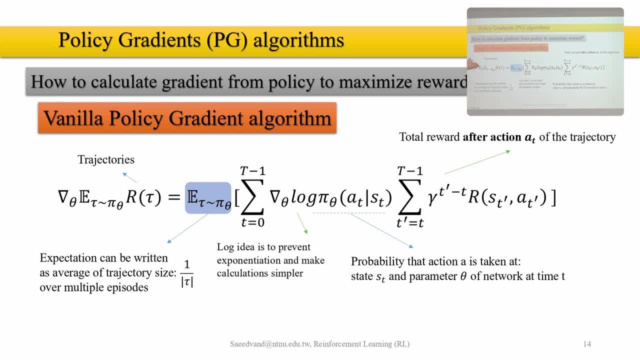 let me come from beginning. So we have gradient, We want to calculate gradient of the expected return on the trajectory. This, this tau here is trajectory that is generated by policy. pi again, one network, And this is like the rewards of the trajectory that we have talked. 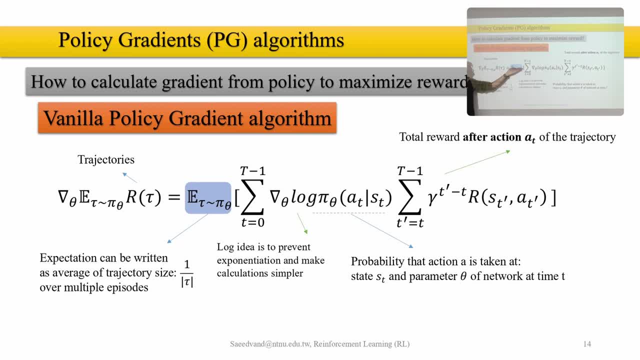 So this is equal. Okay, So two calculation of the expected expected trajectory from policy pi. that in vanilla, in the state of a previous algorithm, we usually want to do. we usually calculate the one over size of the trajectory to get kind of the average of multiple episodes. 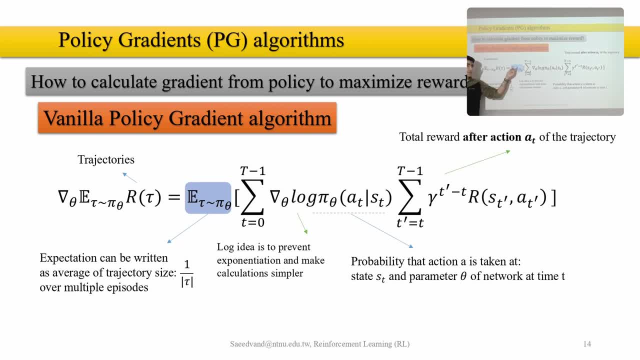 Difference number one. So here we want to get average. If you remember, in policy in Monte Carlo- Okay, In Monte Carlo techniques, I was mentioning that the expectation usually is average. So it's the same thing. The expectation here of this policy is the average one over size of the trajectory. that 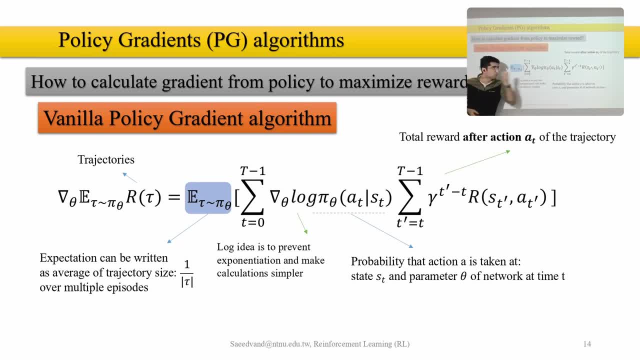 I have times. So the average of this term over here, that says the same calculation that we had, the sum of the T from zero to three, minus one gradient of the logarithm of the uh, the policy, pi, Okay, And the same definition that we've had then here, instead of GT, we want to put this statement: 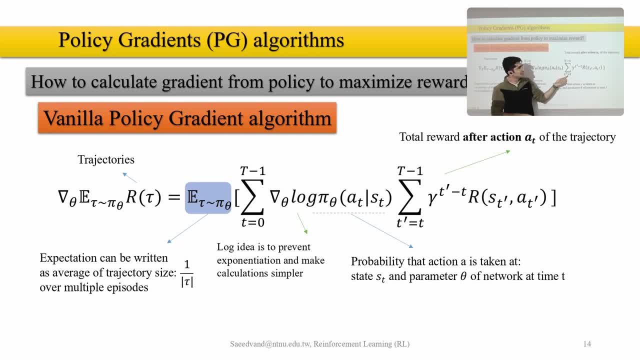 over here that this statement in the state says: uh, get total reward of the actions after, after uh, the action that is happening. It means that instead of calculating from scratch, from zero, we we always calculate the discounted Three. 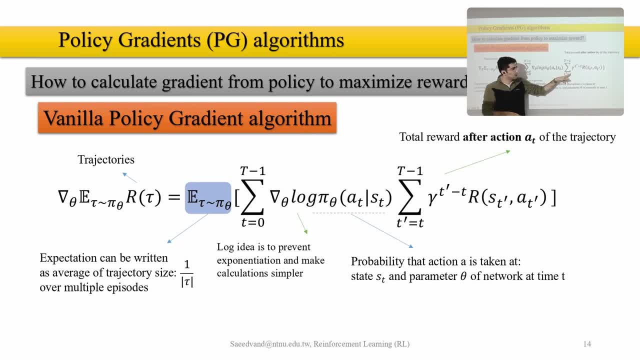 Uh. T equal T, prime equal to T. It means that when T is increasing, this is starting from next uh to to forward view of the trajectory is not coming from the beginning, that we have different techniques of Monte Carlo. We've already familiar with it. 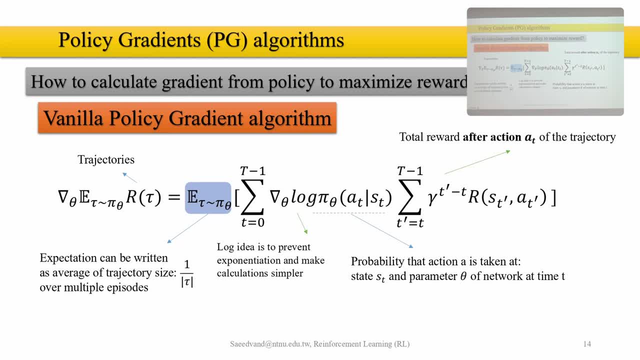 So in the force we did calculate the based on the return, But here we calculate based on the return, Okay, Okay. So how do you do this? So, first of all, we get the, the incoming, oncoming actions in the trajectory, just. 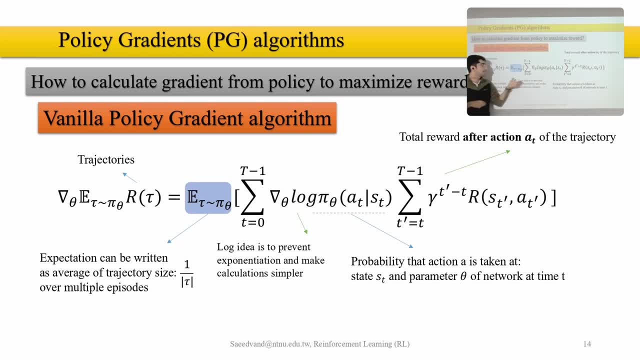 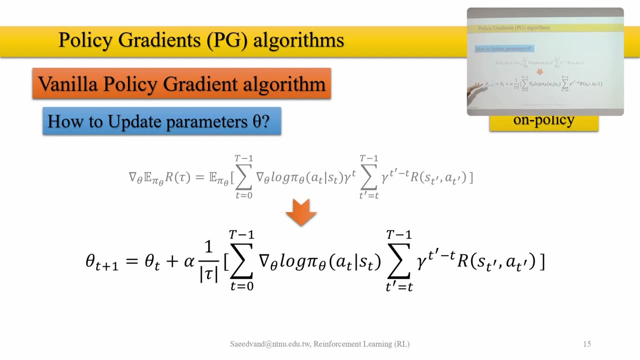 looking forward After trajectory first Second we get our reach. So this is called factors, the one algorithm in the state of being forced on what we do. Again, we cannot take the parameters off the toth network by the same process. 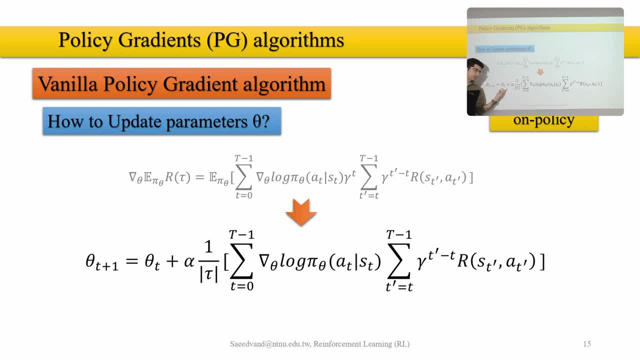 It's all off, But he added five on- is equal to current weights of the network. Learning rate times The average. the calculation gradient of the logarithm of the probability that can come from different techniques. One is softmax of the network, then times the discounted reward of ongoing actions. 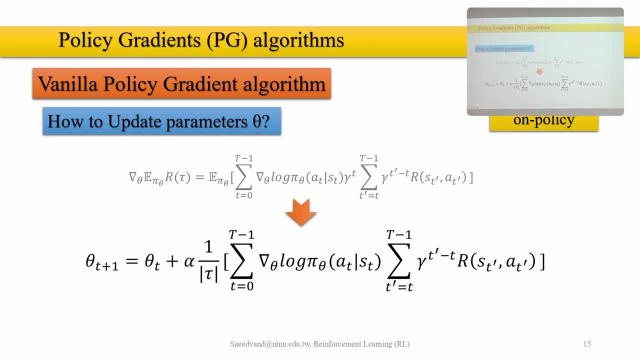 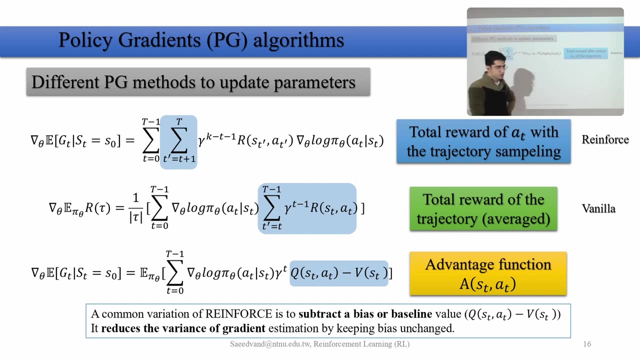 oncoming actions of the trajectory. So again, vanilla is on policy, same as the reinforce, And now, as I mentioned to you, let's have a look what else we can do over there. The policy gradient technique of the update of the network weights is the same. 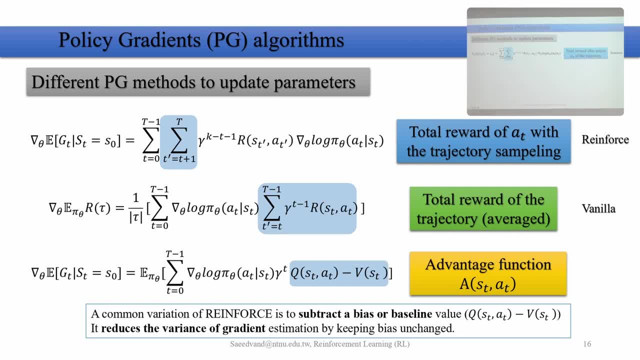 But have a look what we can do. First of all, we've seen this as reinforce, Total reward of the trajectory, Total reward of actions. Then here we have the vanilla algorithm. So here, just I put the return inside instead of gt. 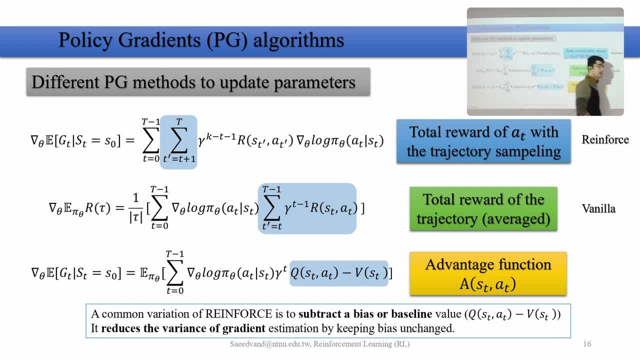 Then what else we have? We have very nice definition here as advantage function. Advantage function is one of the elements of also some advanced policy gradient techniques That PPO is also using, Some techniques also are using. So what does it says? It says that let's use benefits of both value and policy gradient. 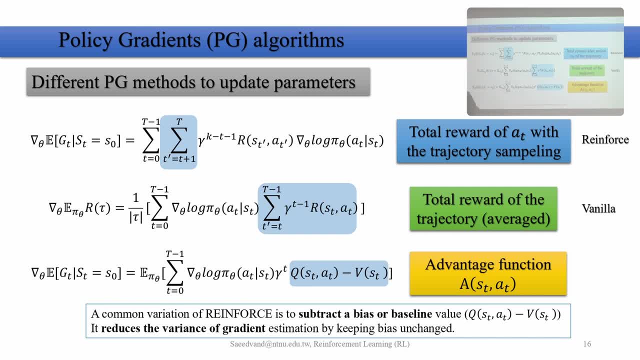 Use benefits of both kind of What to do. let's say the same term, similar term that we have expected: return of the policy pi And some of the gradient of the logarithm of the policy pi based on the network and discounted. 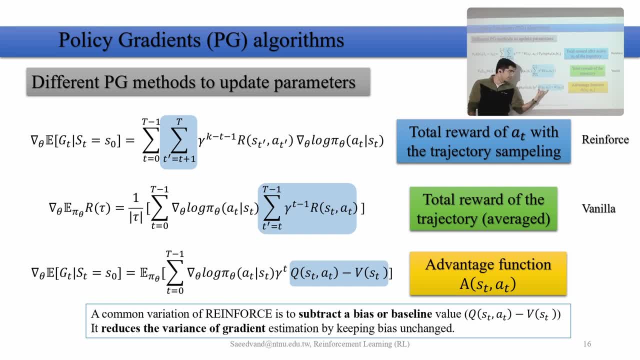 But here we have a new term that says calculate the Q of the SMT and subtract it by value of the ST. So here we have the value of the state, Here we have the each value for each action and subtract it from the value. 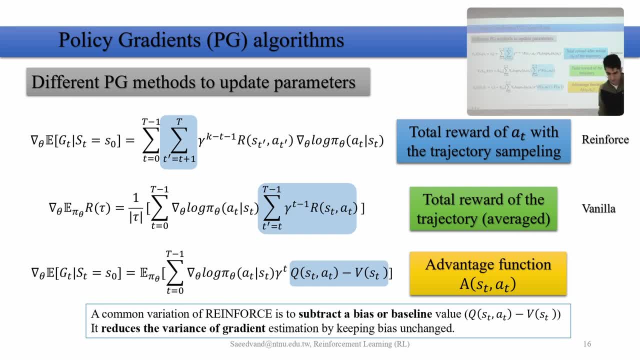 That also is called this part over, called also baseline. What does it mean? I mean this state: we've seen that we can calculate Q and Q can state different values for each action, possible action. which one is better or which one is good? 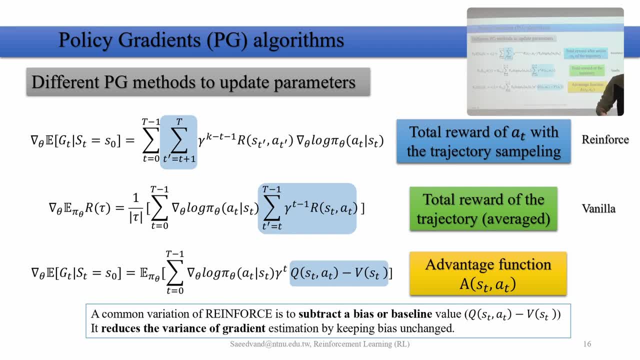 The idea is here: Not only use that one, but also calculate the value and subtract the Q of the action that we are taking in that state by the value. So what does it say? What does it says to us? It says we're getting some advantage. 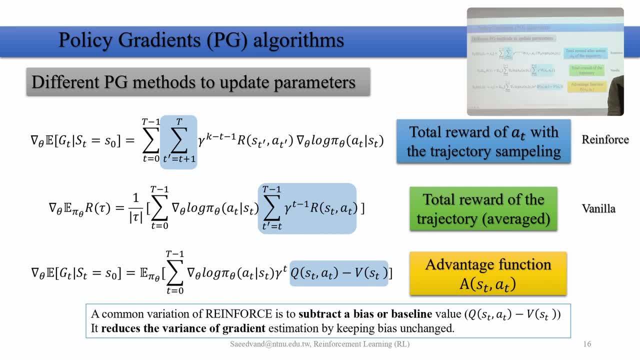 And what is the advantage of If I know that being at this state has like 100 value? what is the advantage or differences of that action with this value? forward action, left action, back action, Kind of comparing the each values by that base value or baseline. 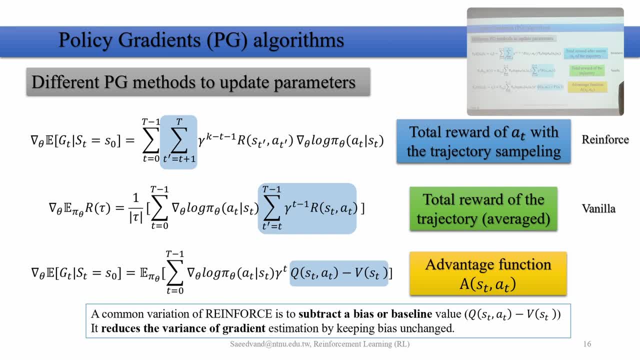 So two times calculations: One time, One time for the state, the value, and one time calculating each one of the maximum of the not maximum, each one of the values for action that are possible. Then we are kind of finding the difference. 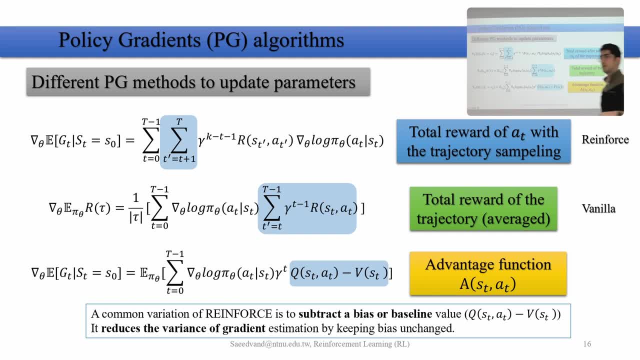 And that difference called advantage. Why? Because this is more stable. Okay, Any question? Okay, Okay, So by looking at this, if you want to rewrite the equation to update the parameters, theta will be similar to previous ones. I didn't do that. 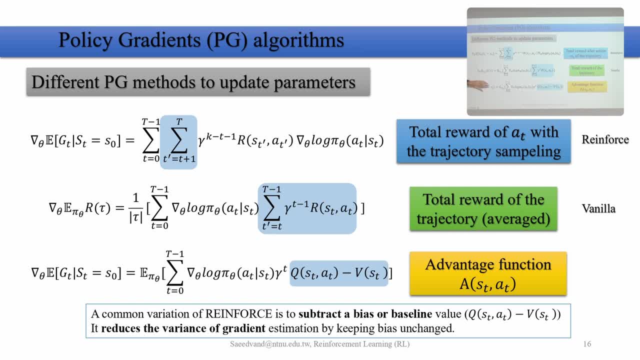 Theta t added by one equal to theta added by learning rate. And after this, expect it this term, So that now, instead of, instead of creating like trajectory, like here or here, we say calculate the advantage, Okay, And then we update the weights based on that advantage. 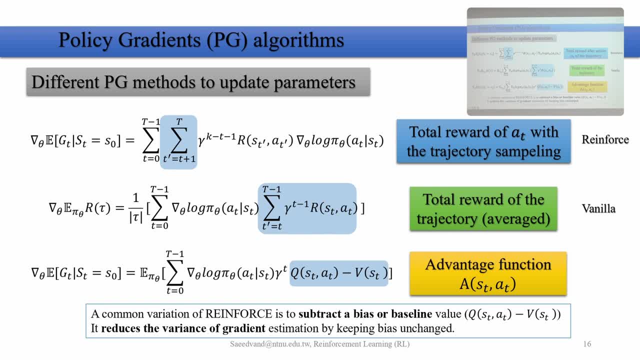 So I have a note here. Let me see a common variant of the reinforce. It's subtracting bias or baseline that I mentioned to you. This can be baseline Also. we can. there are many different techniques that this value can be replaced with anything. 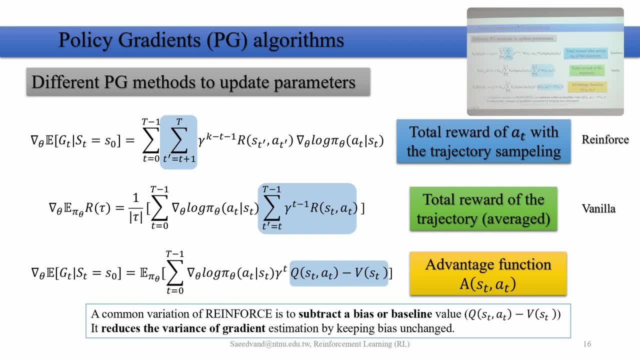 else but that's called baseline Value, for example. advantage that it reduces This value is called baseline Okay, Okay, reduces, kind of formally we can say variance of the gradient, estimation will be more stable. So it means that you know the variance can represent the error. 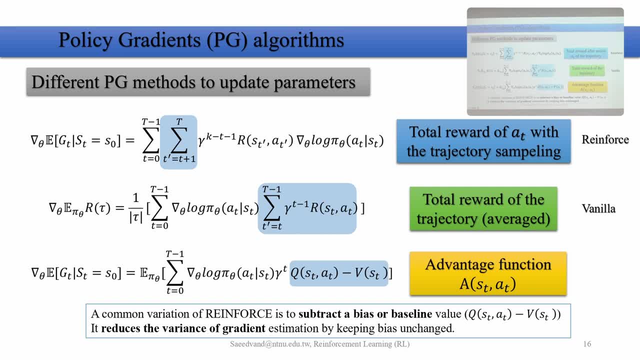 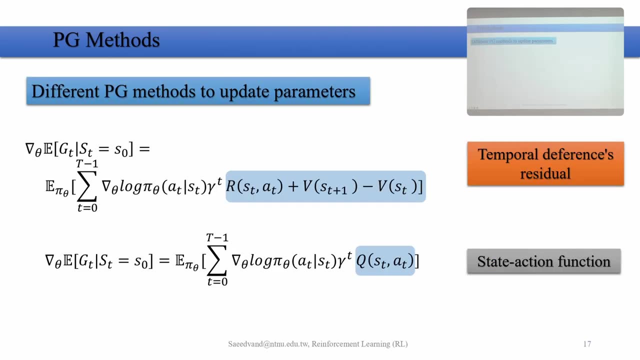 If you consider the distribution, the variance is wider. then our error is higher. So it kind of tries to make it more stable or reduce it. reduce the variance of the gradient so that it will be a useful advantage function. But also we will have a point over there too that we should be careful with. 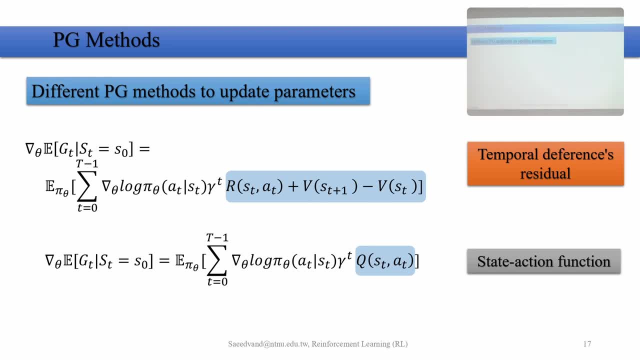 In the next slides I will discuss about it. What, if? what else we can do? One of the techniques also is temporal difference. We can say, okay, let's calculate the residual temporal difference instead of Monte Carlo Bayes-Crayton trajectory. that we see that. what was the reason we bring the? 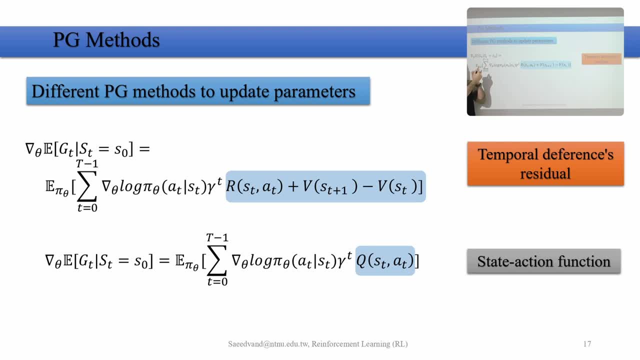 temporal differences into game instead of Monte Carlo approach. that. we see that. what was the reason we bring the temporal differences into game? if you remember, in Monte Carlo approaches we had to generate whole tasks, then do whatever we want. But we said, okay, that's not good, Let's introduce TD. And we see: TD zero, TD lambda. 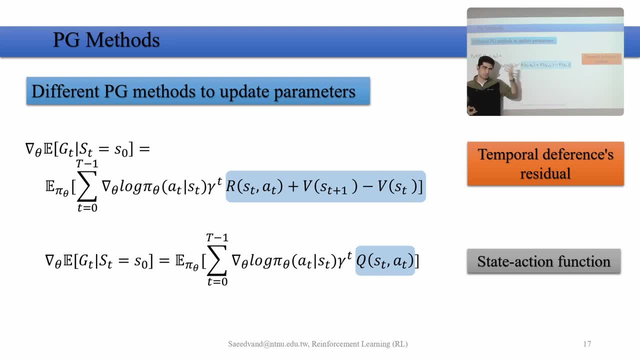 different techniques of TD. So the same scenario, the same motivation idea can come here. We can replace it with TD temporal differences, the temporal differences of the value of the SD added by one, or value of the SD. So what is the difference between this state and next state? 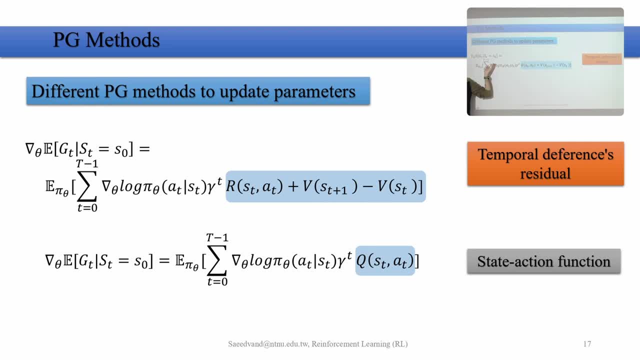 In order to update the weights, in order to find out how good it is. this is not only limited to value. it can be key value, but we need to then modify modifications over there. So the first part is same gradient of the expectation, expectation policy. 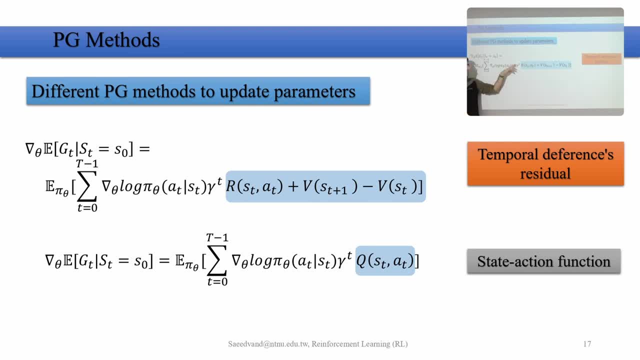 some of the again gradient of the logarithm of the probability times, discounted factor and temporal differences that the updates of the network is based on, the how much each step the state is. the value of each state is improving by temporal difference, so can we do something else can be used instead of: 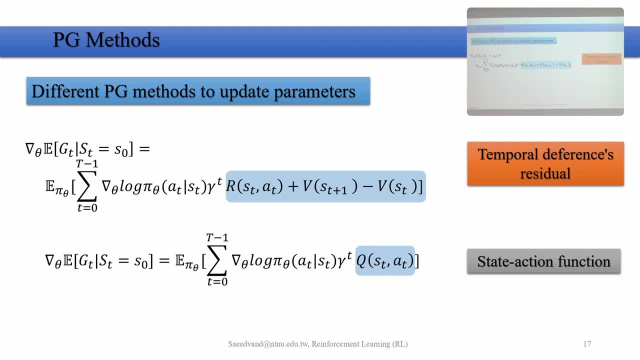 TD. this is TD 0. right, this is TD 0. can we use another TD algorithms here? yeah, you can do. you can replace any TD algorithm that we studied in specific chapter for that. over here inside policy gradient, for example, we can have state action function. that here we can say: okay, let's. let's say after, after doing. 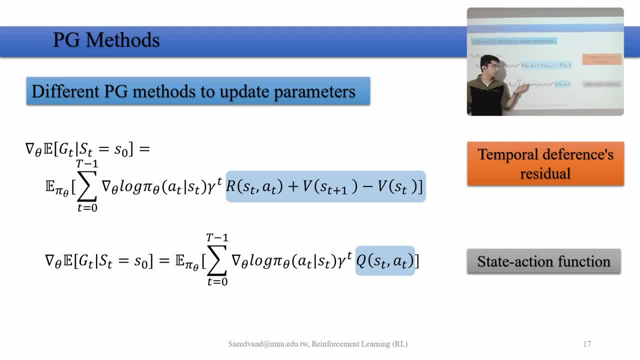 the same calculation expected sum of this term over here. finally, we can say q of the state of action instead of value or temporal difference. We can directly also put the q over there or td of the q over there in order to update the parameters. 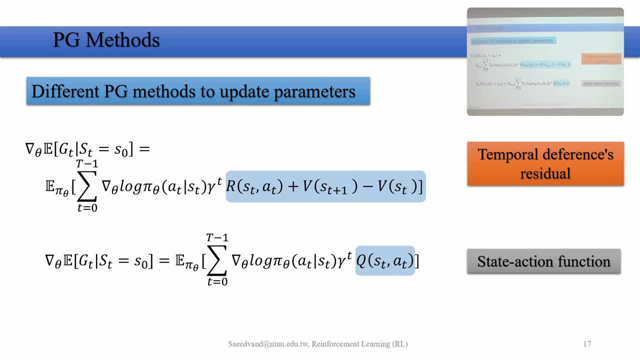 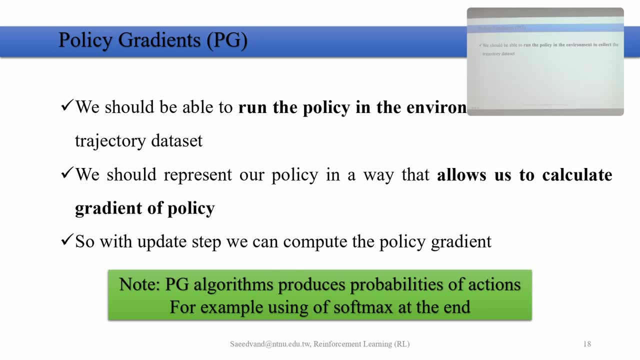 Clear Questions. OK, Now we say we should be able to run the policy in the environment. So we have some points. We should be able, first of all, to run the policy on the environment in order to calculate it or in the simulation. 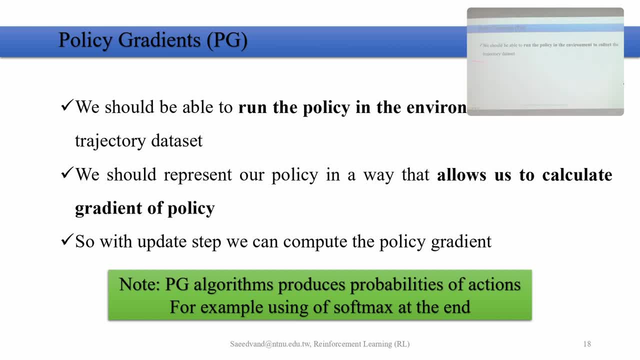 That's, of course, obvious. It means that you need to define your algorithm, kind of, to be able to generate the action and run it over there, But also, in addition, we should represent the action, As I mentioned somehow that we can calculate the gradient. 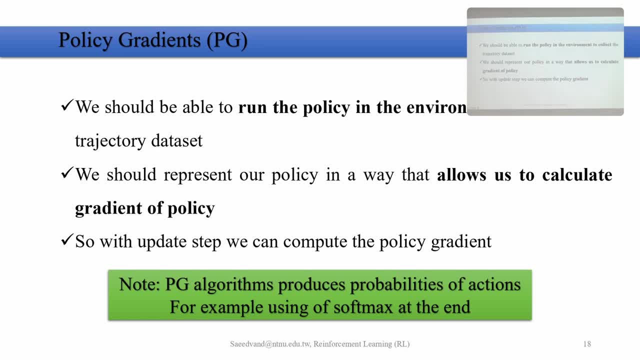 of the policy over there. So update state, then we can calculate the policy gradient. But important point is that the policy gradient algorithm produce probabilities of actions, for example using softmax at the end. But also we needed to know it in advance. 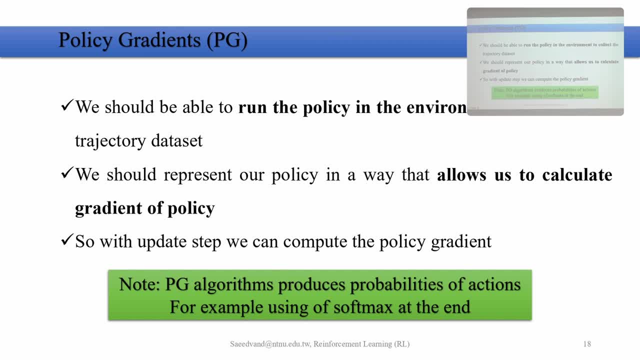 I mentioned it before. come to this point. One is softmax. We can do it, But bring it the transition probability in any form that we can have. It's actually saying that what is the probability of happening the action as output with softmax? So by given, by state. 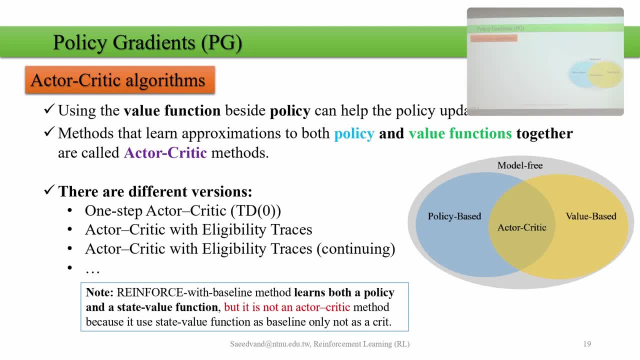 OK. So by knowing that background from policy gradient, by knowing two algorithms of the reinforced and vanilla, and seeing that how we can update the parameters, now we can have a look at one of the also famous algorithms of policy gradient. that the idea is OK, we already. 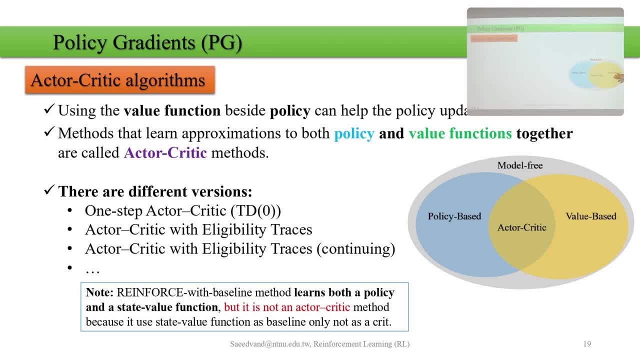 knew policy-based techniques before today. OK, So we can use the value-based techniques. We knew value-based techniques, But today we also have seen some techniques that is policy-based. Now the question is: can we use both together? Can we use somehow the value and the policy? 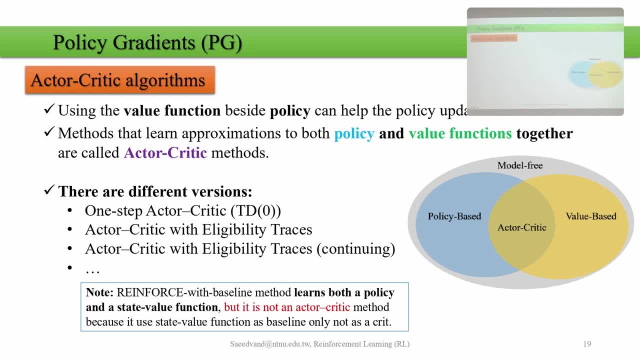 to do the same procedure to use benefits of both. Yes, we can do, And that's a reason algorithm are called act or crit, So we say using value function besides policy, we can update the policy updates better And that method is approximating both policy and value function. 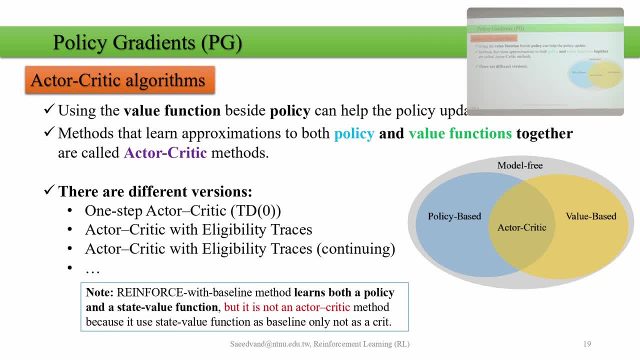 that called act or crit. I already explained And there are different versions of act or crit, Too many different versions actually. I can say One of the basic and starting point of for example policy gradient is one-step act or crit. 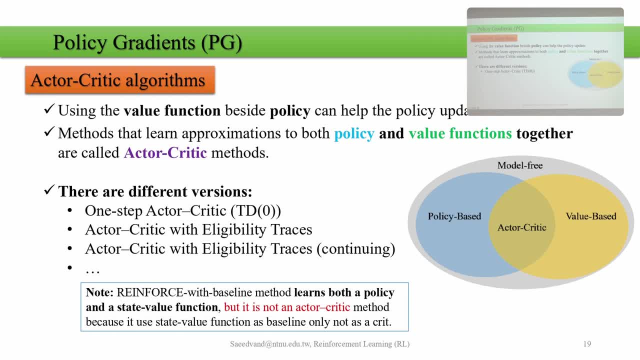 That is based on td0, again, temporal differences 0.. We have, like we already studied, for example, act or crit with the eligibility trace. You know what is the eligibility trace To update based on the trace of the backward or forward view. 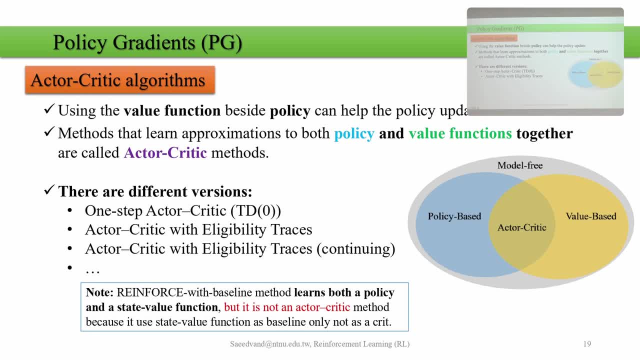 of the value function. So that can be also part of act or crit policy algorithm. You can bring it inside here We can have like act or crit. We can have act or crit with eligibility trace. that is continuing. It's not like here we have finite horizon. 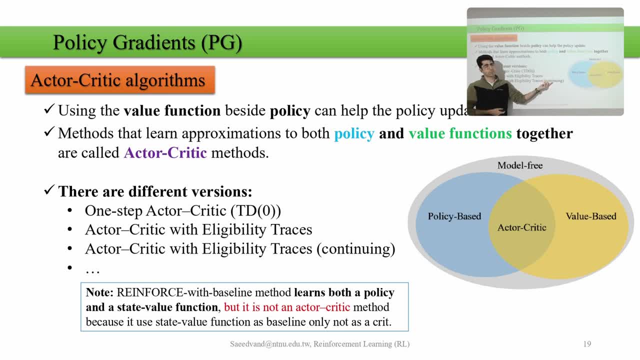 that episode ends somewhere. But in kind of tasks like prediction, your agent needs to do trading And forever it's like trading. every episode finished, The weather prediction. weather is not shutting down like after some episode, It's continuing. 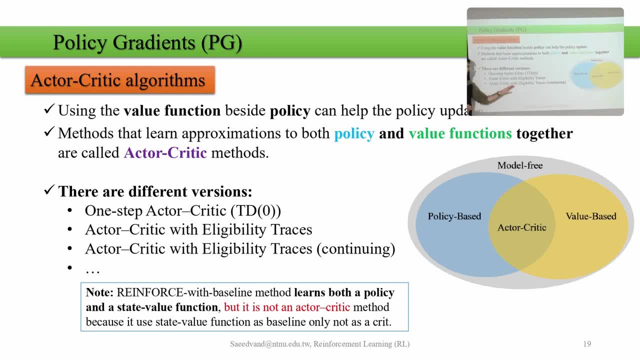 So in those kind of algorithms also we can use eligibility trace of the activity. OK, Thank you, You're so welcome, Thank you, Thank you. Thank you for listening. another class of DISCITES in proximal space and other Vaticans today. 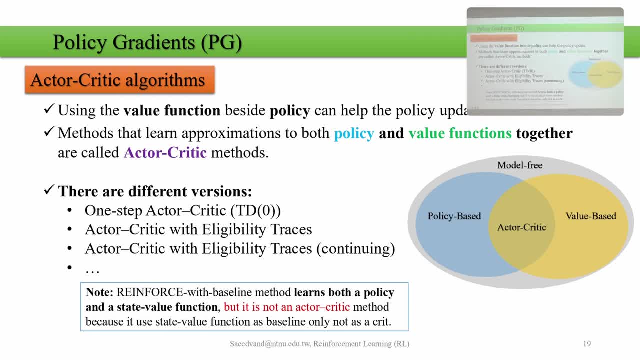 And pointed out extremely useful. So let's go on to the next part. Thank you, value function together. so it was using, it was using the uh uh. it was using the uh, the the uh- both terms together. but we should not be confused that it is not actor critic, that's. those are. 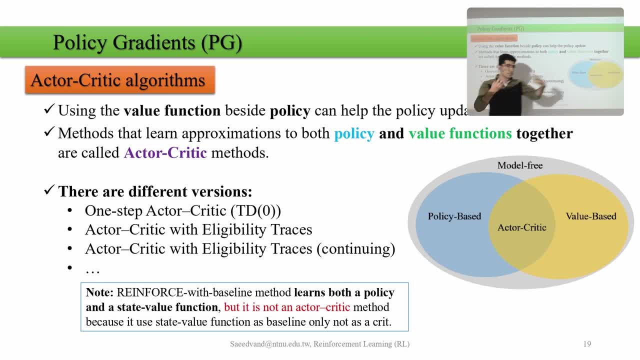 different. what's the reason? because we want to kind of create a criticization of the actor, that this criticization tries to improve the actors, not only calculating in one identical iteration, something like baseline, because baseline has different versions. actor crit, the advantage function is is looking similar to, but baseline techniques are much more. 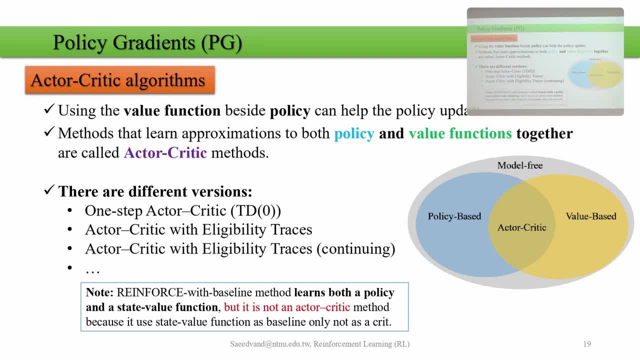 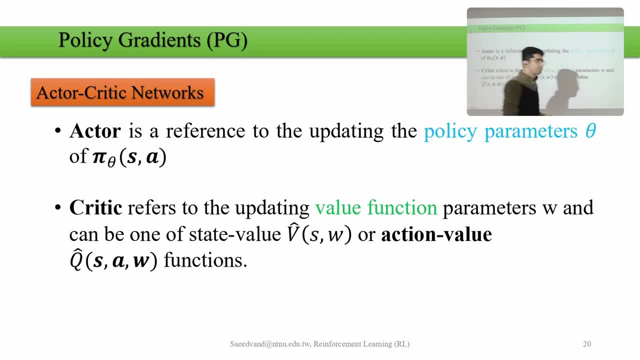 a better example for this one that we should not, uh, mix them up. so so what we have? we have two networks in actor critic. one network is called actor, another network is called critic. what is the actor? actor is the policy updating policy parameters, theta that is represented as policy, pi, state action, and critic is the value function. 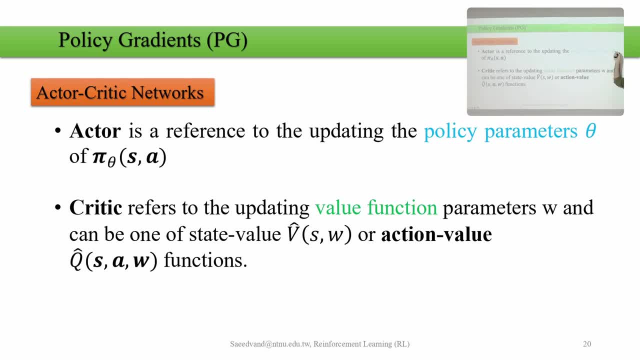 so here we have policy parameters of the state, and then you have new parameters of the state, and then how could you say the dataaltung in this way嗯, value function instead of Q. then we have this one. So one network is for critic and calculating value function. 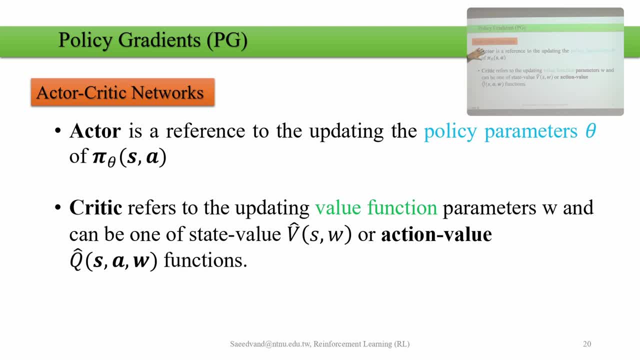 Another network is calculating the policy parameters: Today's course as actor and the value function approximation as critic network. OK, clear. Now we need to see how these guys can work together. That's it: Merge them together in order to update it. 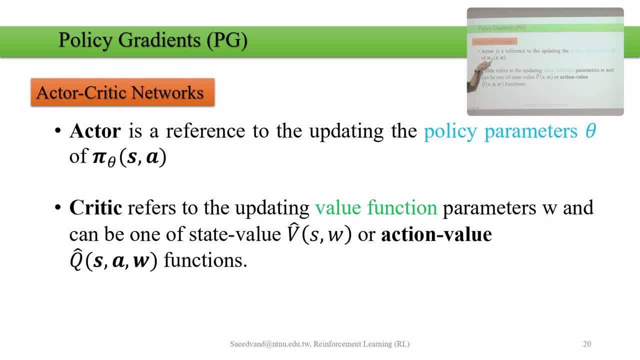 But keep this in your mind Whenever after you see theta- that before today's course we were talking about the policy pi theta. this theta parameter is referring to actor And this W are again network parameters, but this is referring to critic parameters. 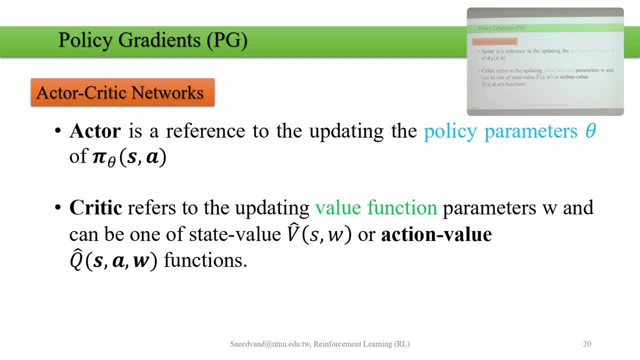 So because they are different network and, of course, their parameters and updates will be different too. OK, So keep this in your mind, Try to keep it in your mind. Keep it in your mind. We are moving forward. So we want to see now: OK, using that actor-critic directly. 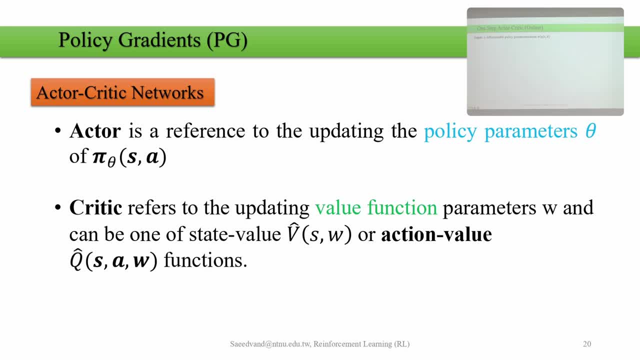 how we can write the algorithm and how the equations looking like in order to have two networks of actor-critic in order to update the weights of the balls, But by the name. before I continue, also have a look here. Critic is criticisation. 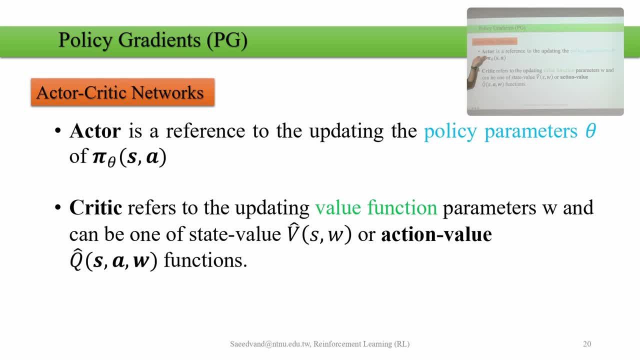 Kind of saying what to do, what not to do, to actor. Keep this in your mind: that actor is generating the policy parameters. that policy, finally, is running in the environment, But critic uses some values in order to improve, in order to kind of advise the actor network. 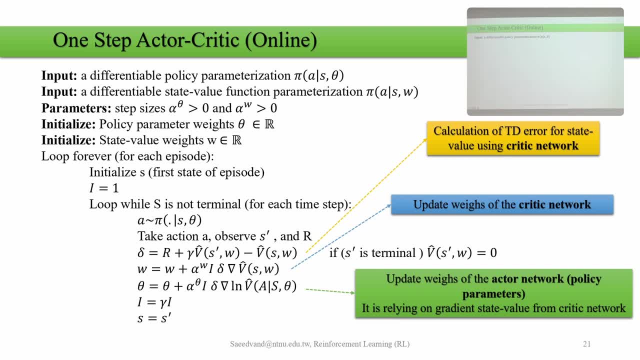 So, based on that, let's have a look what is happening. Input is a differentiable Policy, parameters, policy, pi, action, state and theta. One input And second one is differentiable: The state value function parameterisation that is stated as pi of action given by state and w. 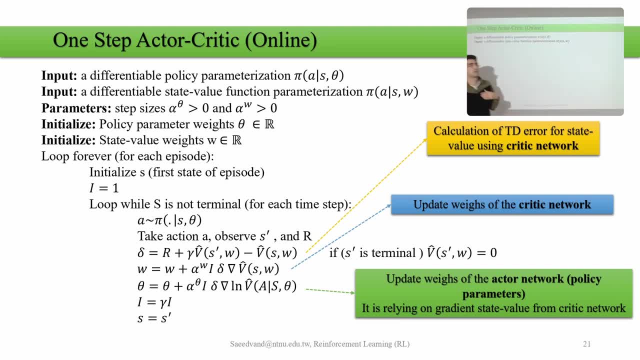 So actor, critic, as initial values And of course, we will have learning rate And learning rate for both of the networks. we will have alpha Learning rate: alpha for network of actor And the alpha for network of critic. Both must be greater than zero because we 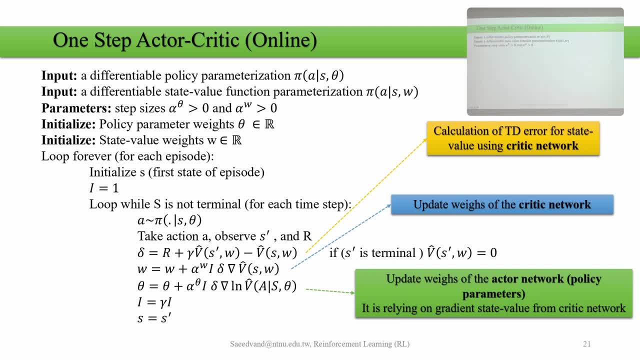 want to learn. both networks must learn from the environment Also. keep this in your mind. We have two pure random networks at the beginning. Both of them are trying to be learned, Both Right policy network, both actor network and critic network. 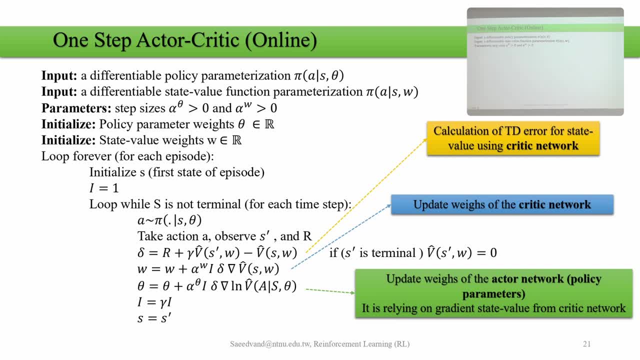 At the beginning they are zero, nothing knowing How they are learning. They are learning by getting some rewards from the environment and updating themselves, but trying to improve each other too. So what we do? first of all, we initialize the weights. 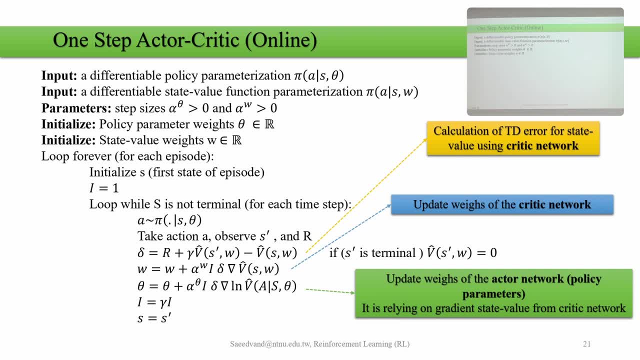 of the first network and initialize the second network. Parameters theta and w can be zero again or random values Initialize again. We create a loop forever similar to previous one for each episode And we initialize the state of the episode first state. 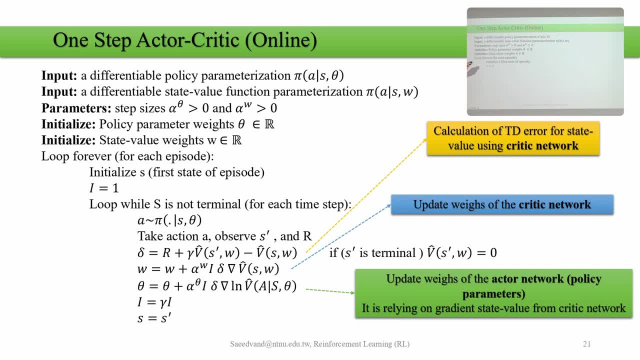 Keep this in your mind: This algorithm is online And, since it is online, we are not generating like Monte Carlo trajectory at the beginning. We're trying to update it in online way because this technique also can be implemented, similarly, Similar to Monte Carlo. 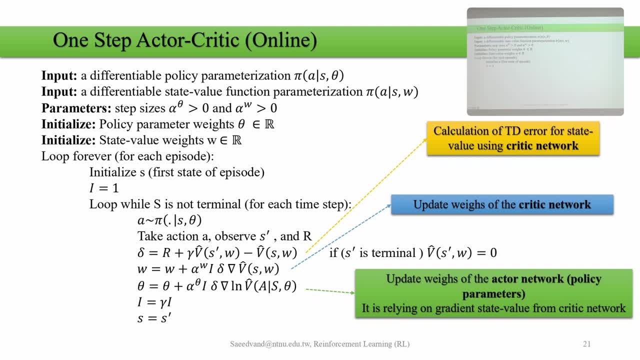 We create a variable i that is showing these steps, Iteration kind of as one. Then we are creating a loop of the create, of the loop of each step in the episode. So, episode, each step, we want to, one by one. 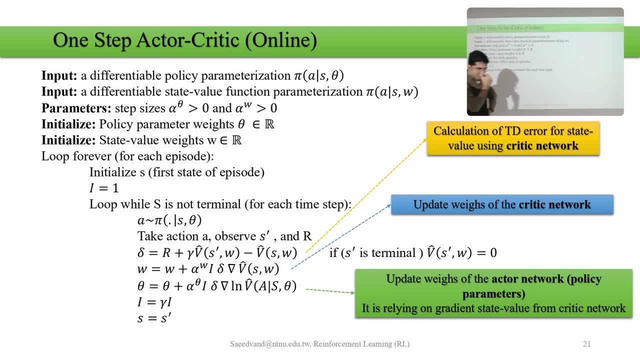 see what's happening, First of all, one, two, two, two, two. we need to Ah, Thank you. And then we can see the action. Action from where? From policy network. What is the policy network? Actor network. 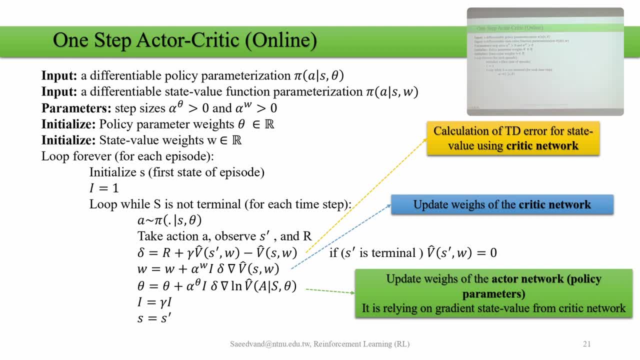 How can I say, Because these parameters are over there, Ketan, And when I ask the network of the actor what to do, then it gives me action, Then I can run it, I can run action. observe next state of the environment. 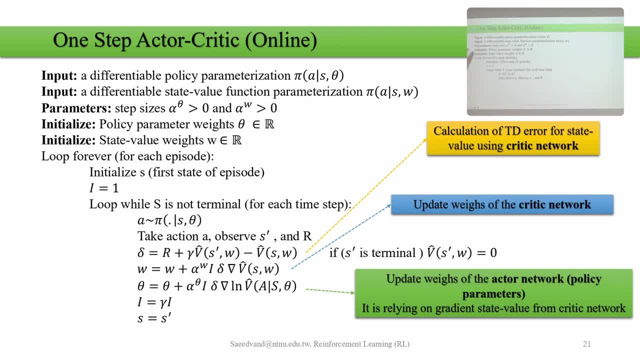 and get the reward. So far, very simple. Nothing. nothing special happened. Two networks and I take the actions. I ask the act what to do, then I take and see the next state. Now we want to see what's happening. 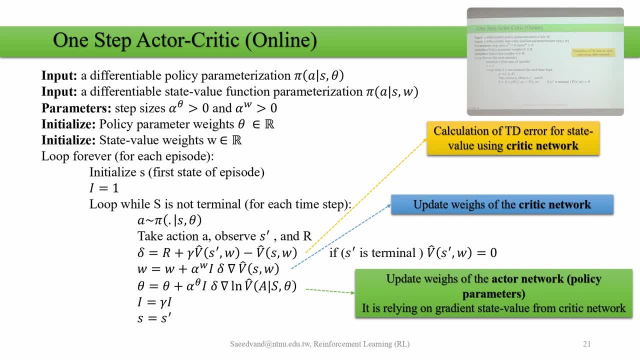 All the actual critical update is happening over here. First of all, we calculate the temporal differences error because the algorithm is online, OK. OK, If it's something else, we can calculate it differently, based on return or whatever Here, since it is temporal difference. 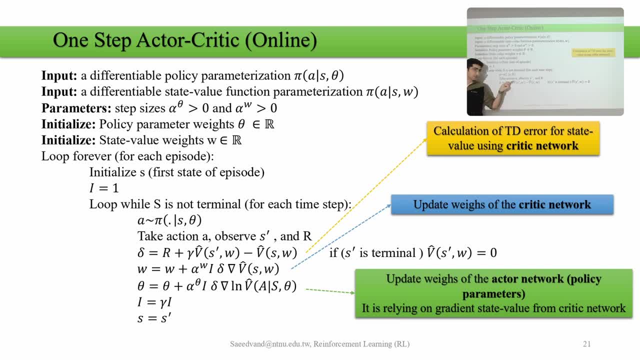 what was the temporal difference? Predicted value. Why predicted value? Because it's network. I told you, when we have network, we put hat here. Predicted network predicted S prime and W subtracted by value of the S and W. 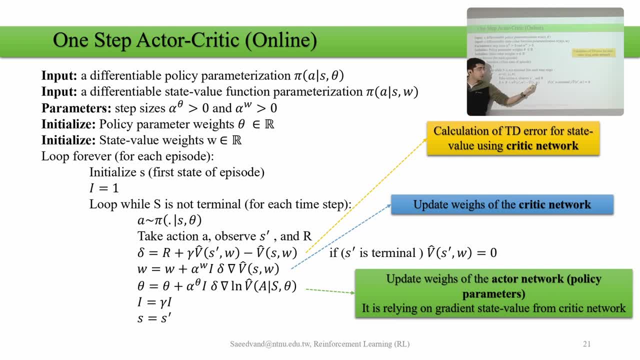 So when we have W here, I'm asking critic network From critic network that is in charge of Answering me the value. I'm getting the values and calculating the differences of those values by giving this state And next state. I'm saying what's the value? 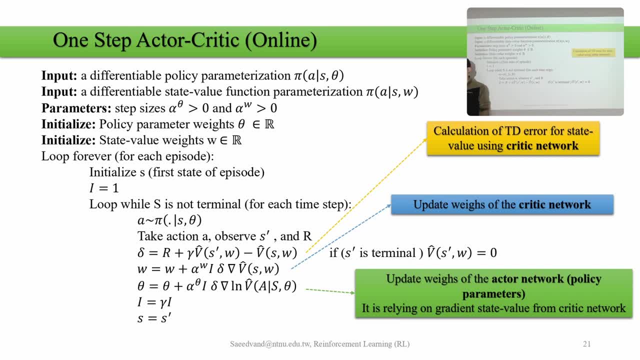 Calculate it, discount it, add it by reward and put it in another variable like delta Clear. I calculated the TD error by value. Just have a point here that if If next state is terminal, it means that it is finishing, then the value of this S prime. 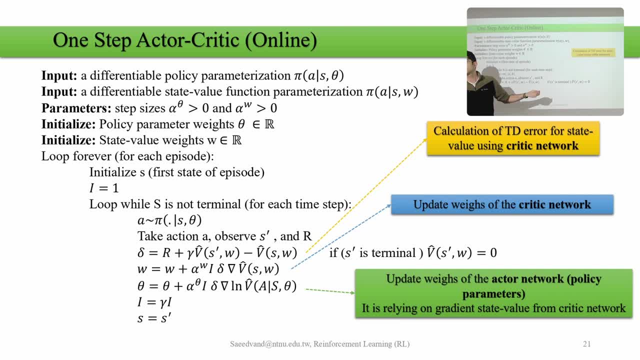 will be 0, because we don't have it. We cannot ask the network right That's not existing. You cannot ask non-existing thing. Then we say: put it 0 over there, Replace 0.. Clear, We calculate the TD error first. 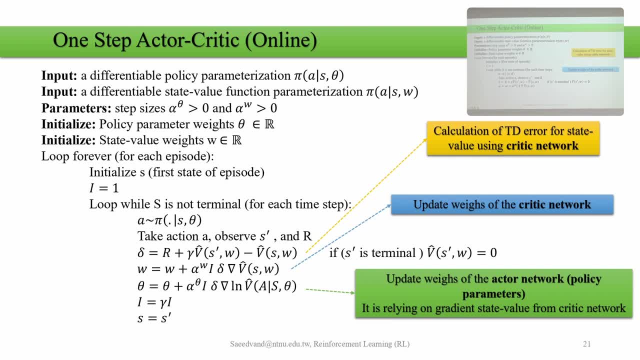 Then we just have two steps: Update of the parameters of the weights, simply What we do. The weights of the critic network w is equal to. It would be better to show it as wt added by 1, but consider that new w's by previous w's. 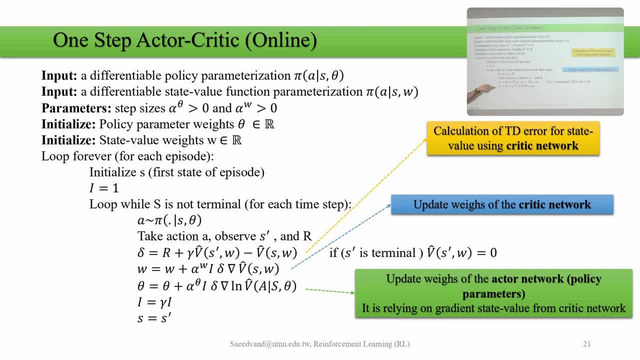 It is based on the presentation of, I think, the book that you have. As I remember, I brought it from them. So w next weights is equal to current weight added by learning rate of the. w learning rate of the critic network. 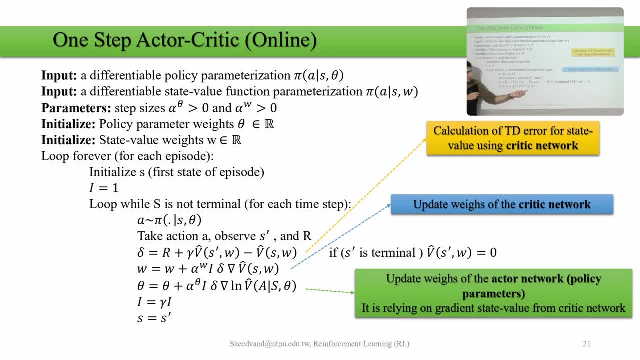 that I defined here, whatever it is Times, the term that we discussed already, The i is representing the step size, the comps that we are moving by, some that we will see how to update it, The TD error that we calculated there, the delta, so TD error. 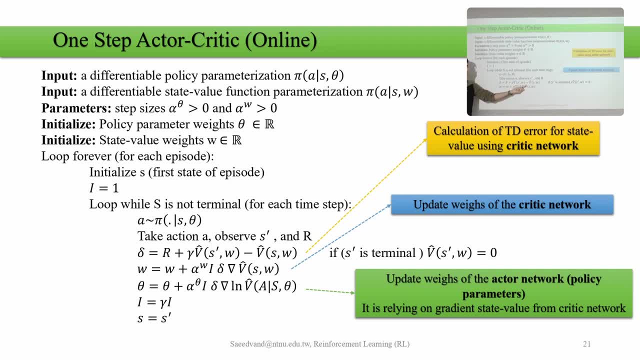 times gradient of the Predicted value, that this predicted value, gradient times the TD, error times, the learning rate and some value of i that we will calculate down there can help us to update our critic weights. critic network weights. 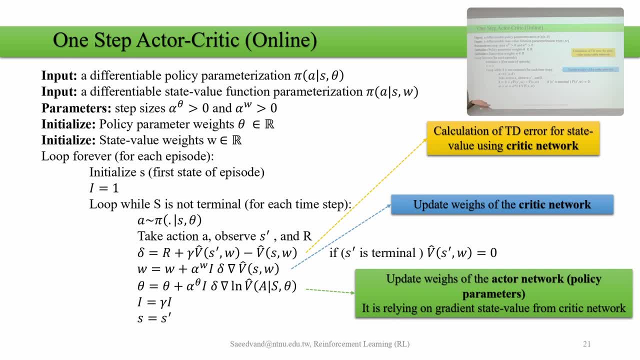 So that's also clear in understanding. The idea is very clear. I'm calculating by the reward and the error by TD. that we've seen, for example, in many algorithms how it's working TD. When I'm calculating that I'm merging. 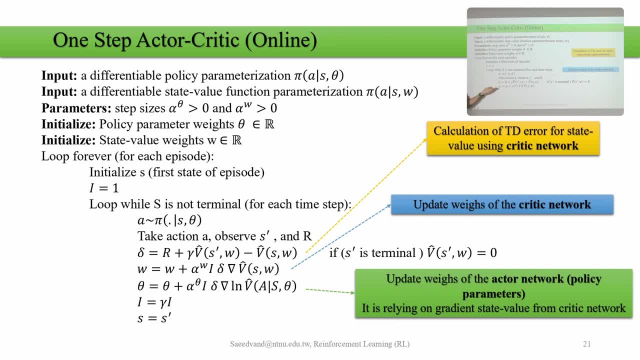 I'm putting it into form of updating the weights that I have for network of critic. What about network of actor? We can do the same thing. Update of the parameters. theta is equal to new theta, previous theta added by learning rate of Actor network. this time times completely similar. 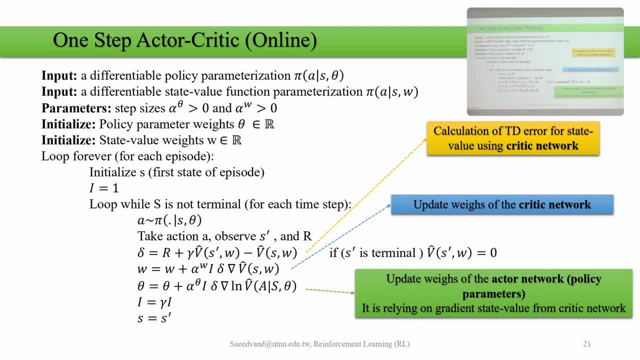 But here we have logarithm of the value because we discussed in policy gradient. Here we have the. we are talking about the value, But here we are talking about the policy. So because of that logarithm of the value of the action, 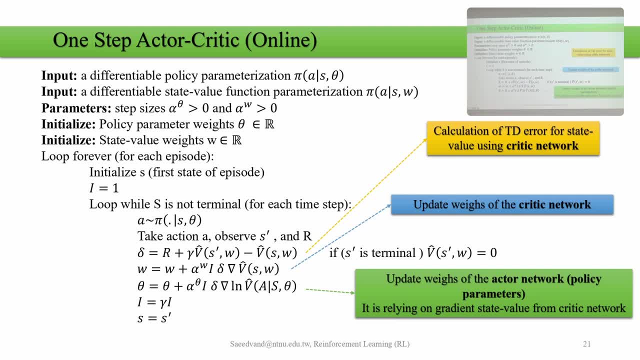 given by state and theta and the parameters that we have. I also have written there a point for you that we are updating weight of actor network policy parameters and it is relying on the gradient of the state from the critic network. why the state of the critic network? because this value comes from critic network, right? but we are 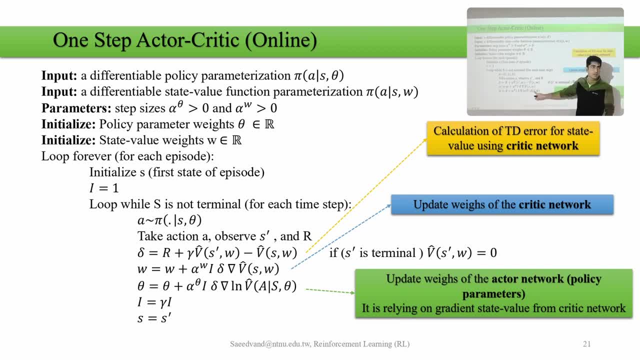 updating actor network. so this is the kind of connection between those two networks. this part over here since comes from: uh, critic, critic, criticize. actor over here sounds like, says like old grandpa, like if i get old grandpa, maybe i'll be talkative, don't do that, don't do this, like that, that grand old grandpa is critic over there. 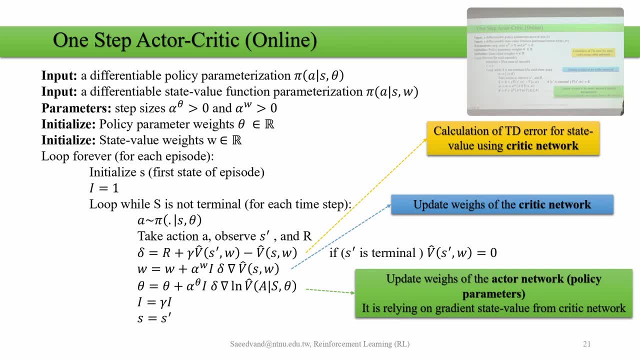 that criticize the network of the theta to update the weights. so one more step: the i equal to discounted i. so this is discounted iteration that i have to in order to update the uh like, say the the future rewards and future updates, because the weights of the like future and now should be differently applied on the weights of 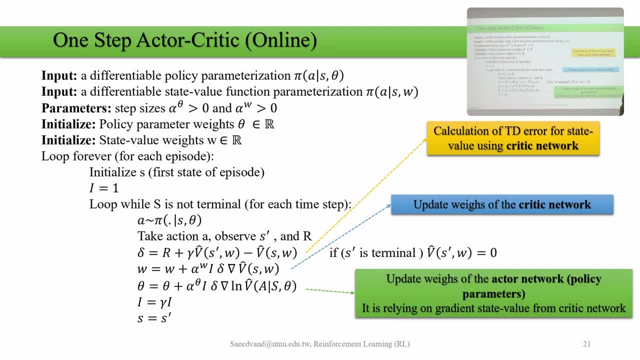 the network. that's why is because of that, something similar what we do for the reward over here- discounted td or discounted reward or discounted- what we do, we are doing something similar on the each one of the weights. any question. if this is clear, this is also based off the many advanced techniques also. it is also advanced. 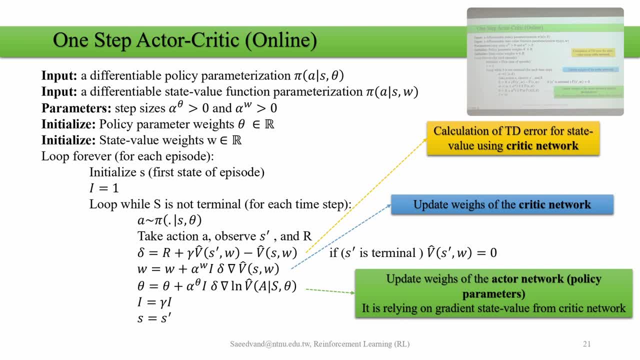 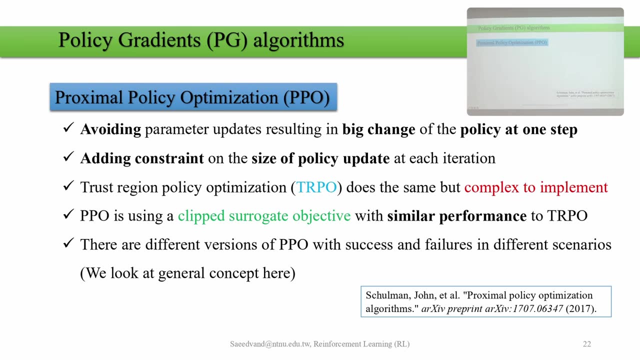 technique, but also based on the many uh recent uh state of the art techniques and because of conservation of this nature, so that we can to Issue the state rising steady state at all. so because, if we look at the process of starting movieuse, all these data from this method and we, Most importantly, all of them we've thought are necessarily 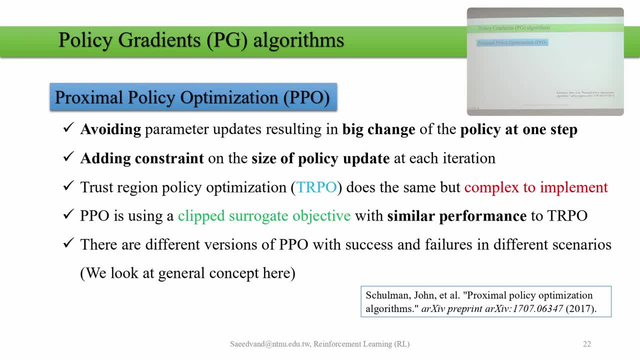 consumed to reduce our state. we don't need to do something extraordinary, we just need to have a look at the flow. and what is the idea? What is the idea? Let's see. First of all, the paper- original paper- is over there. 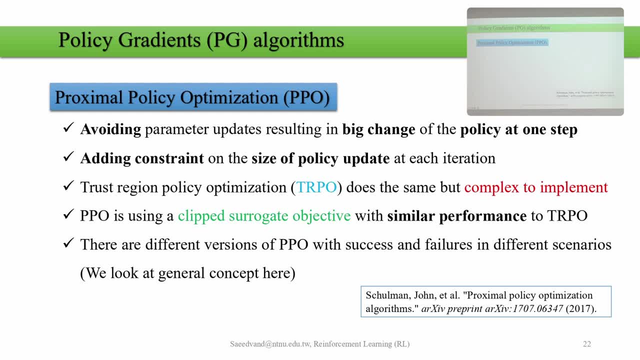 presented 2017, and we call it as Proximal Policy Optimization, one of the famous networks that we have. So what is the idea? The whole general idea says that in actor-critic, the parameter updates can be resulting in very big changes. The idea is that update of the tetas, the weights of the 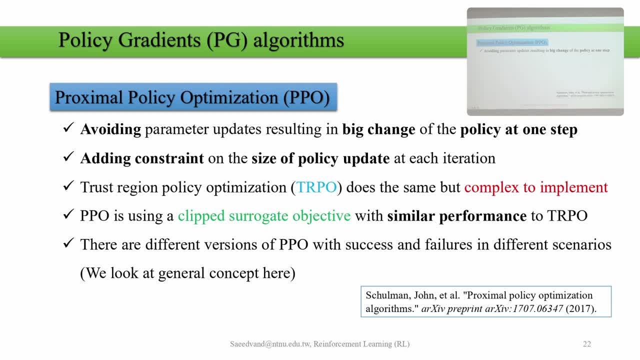 values of the network. suddenly, it's like if you give a candy to a kid to, a kid will be very happy. forget even his mom or dad, right? Something similar can happen in those networks: If agents suddenly see something good and gets big reward, forget. 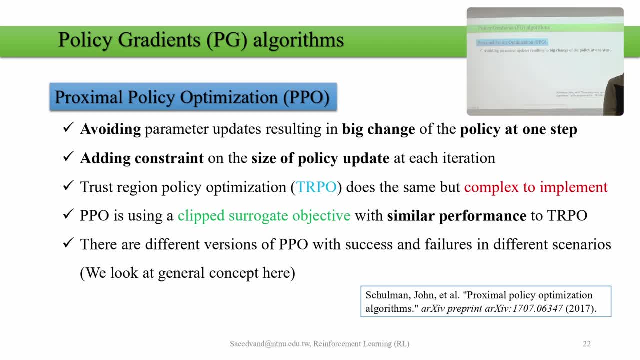 everything but they will melt, and says, okay, you are my god. The TPO basically says, okay, don't do that, let's limit it. The whole idea is this: underline: So: we want to add constraints to the size of policy update at each iteration And what we do. if you look at the 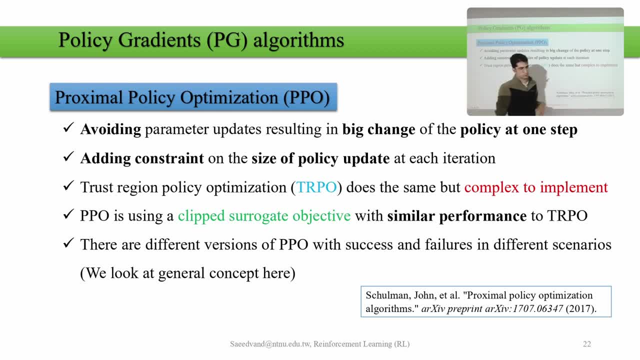 TPO like Transition Policy: Optimization that's also doing the same thing. The motivation is same: limiting the update of the teta parameters or alpha parameters of the networks. But here TPO is very complex to implement, very complex to understand. The procedure is like brutal TPO: just simplifies. 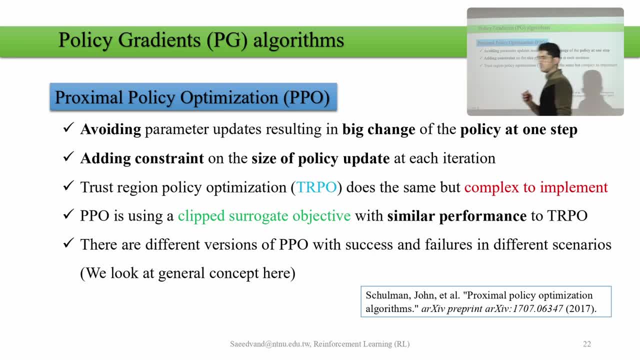 simplifies it and gives it like very, very short understanding of what's happening and implementation. So it is using the technique that does the limitations is named as Clipped Surrogate Objectives. That is similar to in the performance, similar to TRIPIO, as I mentioned. 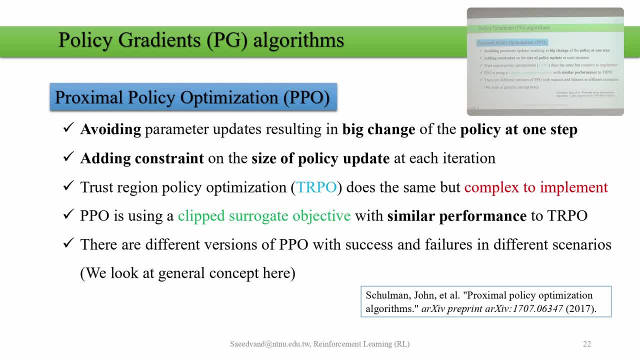 And there are different versions of the TPO and in different scenarios they can be failed or success, depending on what we are doing and the application that we have. But here today I'm going to just have a look at the general presentation of TPO And, as you are interested in, or if you want to do, some research projects. 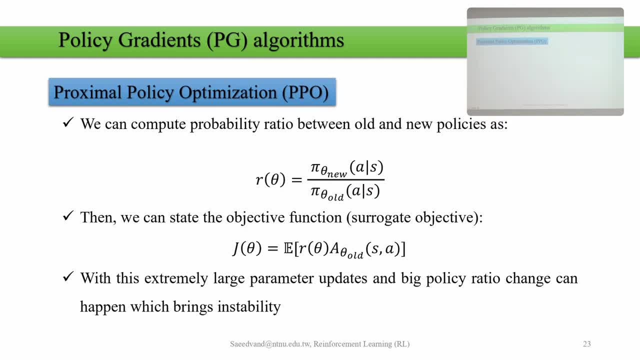 you need to go to different versions of TPO and have a look which ones, in the state of the artworks, are more successful. So we say we can compute the probability ratio between old and new policies. So one step is kind of say, okay, let's calculate the probability of the old and new and calculate the ratio And the 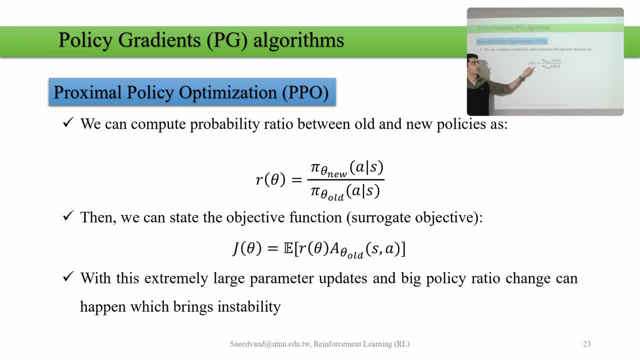 ratio can be shown as this one over here. Simply, we can say ratio of the parameter teta, update of the weights of the teta. This is not reversed, This is ratio. That is the policy, the new parameters values for the policy that I have. 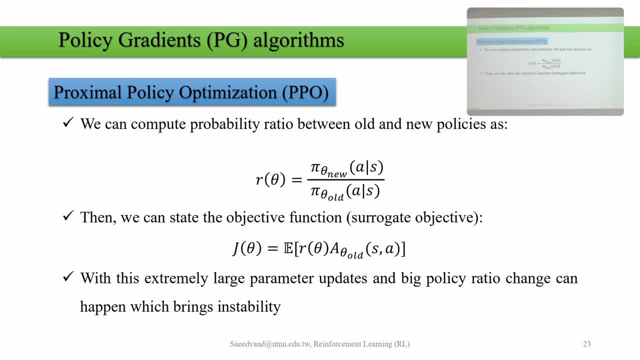 And the old one. if I can calculate the ratio based on that, we can say: then we can write the objective function And objective function can be like the error of the teta that later also we can write again: teta is equal to teta added by this term over here. 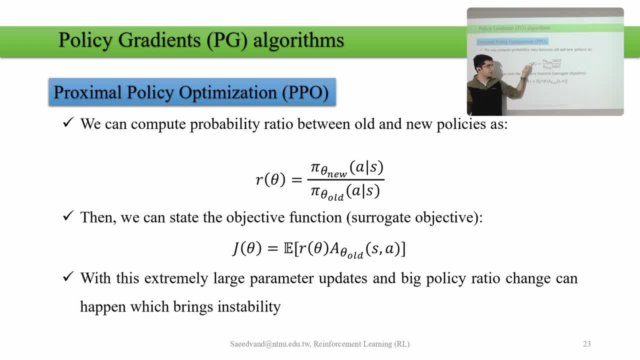 Equal to expected ratio, that I calculate times the advantage of the state and action, An advantage we defined already. So now, but the problem is the idea. the main problem, the main challenge is that this teta can be updated dramatically. That, as I mentioned to you the important part of the algorithm. 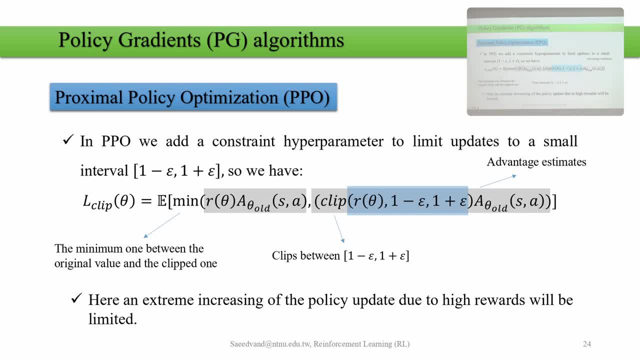 is doing this calculation. So what we do? we are trying to flip the amount of update on the teta. We say, okay, the same term if you don't look up the whole equation. the same term over here of the ratio advantage function of this state and action. That advantage is equal to value. subtracted by the Q, Q, Q subtracted by the Q, It's always the same thing. So the advantage of this function, that advantage function, is equal to value subtracted by the Q or Q, Q subtracted by the Q. 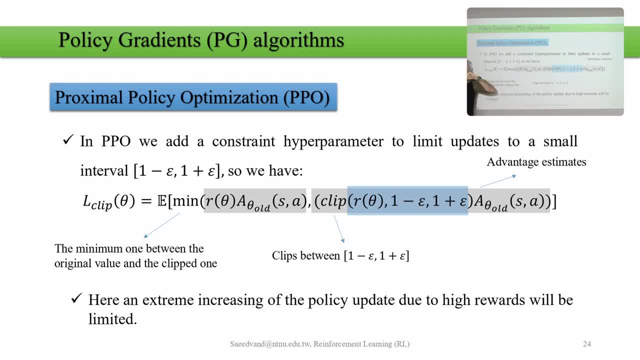 subtracted by value. so what we want to do, we want to get the minimum of this term and this term, left side and right side. that left side is what we've done in the previous slide, but right side says: okay, if that is big, let's define some thresholding by by writing one subtracted by. 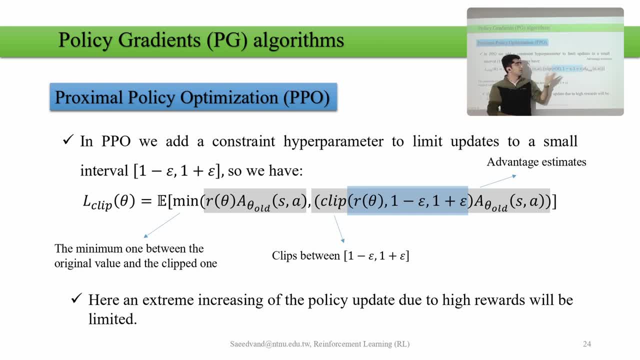 epsilon and one added by epsilon. that this- this- this is kind of limiting our update of the weights- that that, first of all, in this stage we clip the term that we are calculating as original term. this term is original term of calculation. here we clip it between minus one, minus epsilon, and 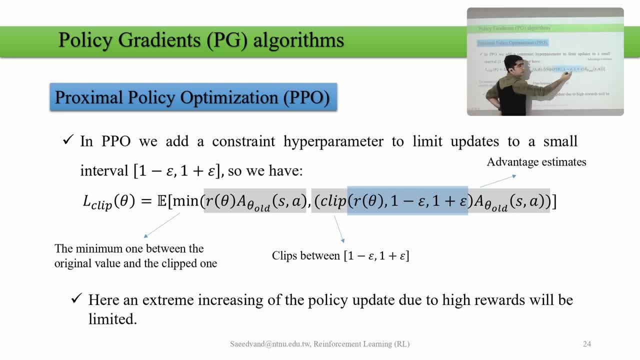 one added by epsilon usually is like 0.2. we clip it and even this clipped version is it smaller than the original one? because we want to limit it? we get the minimum. if this is okay, then use it, otherwise clip it. so if we clip it, then we are limiting our. 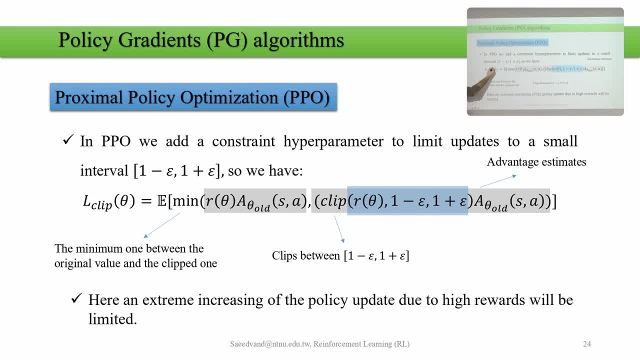 update of the network. then we can write the l clipped. the loss of the clip is equal to theta. then we can write theta is equal to theta added by the this term question. so with policy gradient we saw, we clearly saw how we are updating the parameters, weights, and here just we want to a little bit change on the how calculating. but after 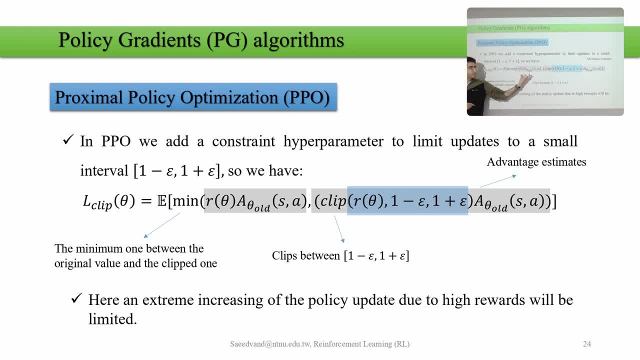 calculating. the most important part is clipping if it is two, and then we are updating the parameters that are in the same place. so one of the most important things we want to do is to kind of creating trust region that how much update of the weight should be. if it's suddenly c candy, say no, no. 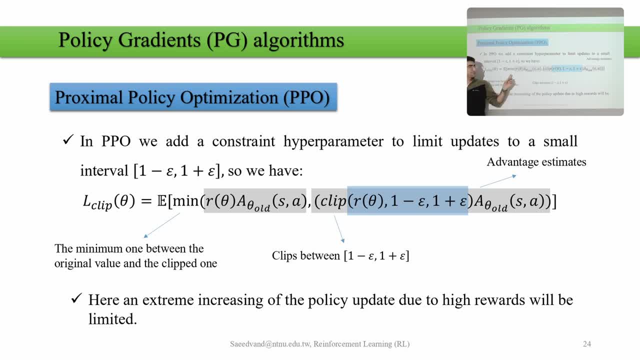 i love my dad and mom. still, i don't want to change all my beliefs with this clip. we will cut it. we put some rules. okay, somebody gives you one million dollars, don't forget your mother and dad. see these guys saying: no, we are gonna forget it. even we're going to forget you. 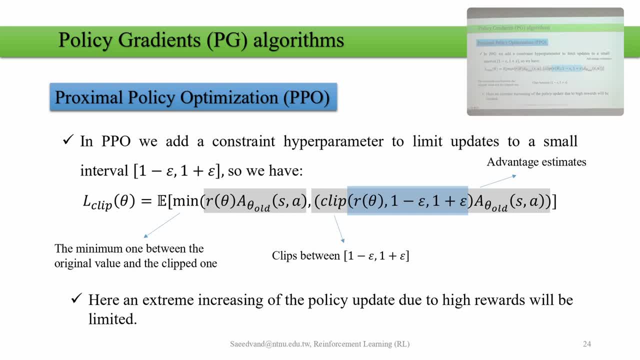 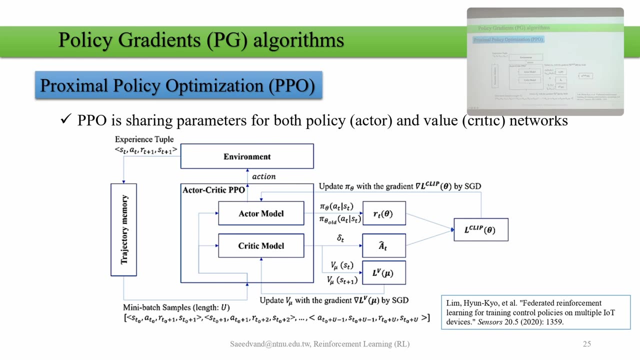 If there is one million dollars, Okay, Nothing is specific. after doing that, Let's have a look at the diagram. all that is looking like. as I told you, it should be based on the actor critic And and we have the environment over there. We have actor network, critic network. 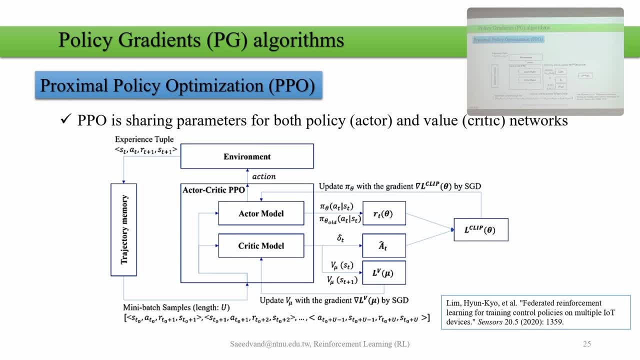 We have trajectory memories over here but they have the point that we have over. there is the clip, so that actor and Critic critic was generating value, an actor Generating the policy right and we calculating the ratio of policy or of the top with the equation That's we said, we calculate the advantage. advantage comes from value function, because advantages 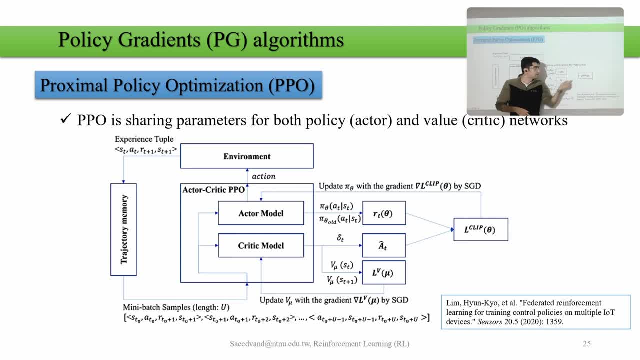 differences of the values over there, then We clip it with the equation of the previous slide. Then, after we click, click, click it, what we do- we update our actor model over there. So So This is the whole general idea. I Hope I don't miss anything. We have mini back sampling over here. 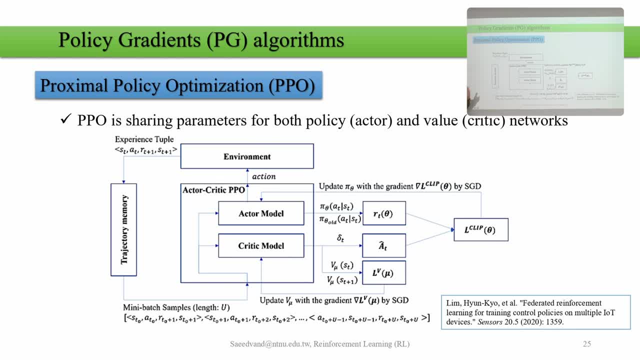 So with mini back sampling, of course We already have seen it in the killer network that we have. We have memory, memory of trajectories, we sample it and the motivation is: don't lose, don't forget the previous dates, Don't don't just only update by current observation, update also by by previous trajectories that agent has seen, post actor and critic models. 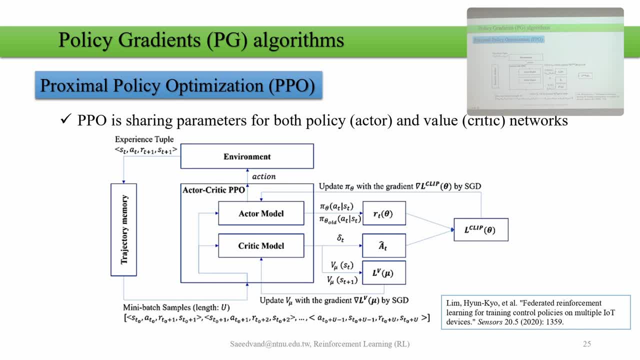 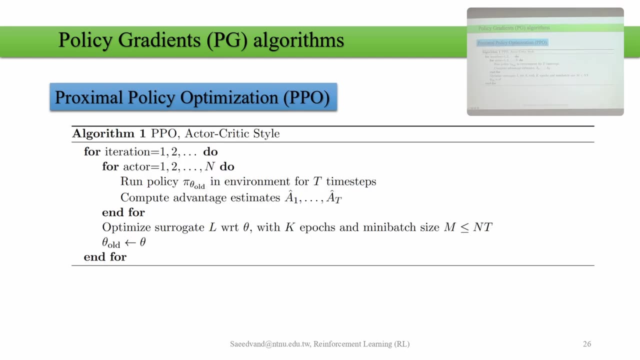 I'm running and this is the paper. I think this paper represents this presentation of the actual critique model that you, if you are interested in, you can have a look in more explanation how those are Happening in more details. Then the general Algorithm looks like. this algorithm looks very simple for iteration one, two. 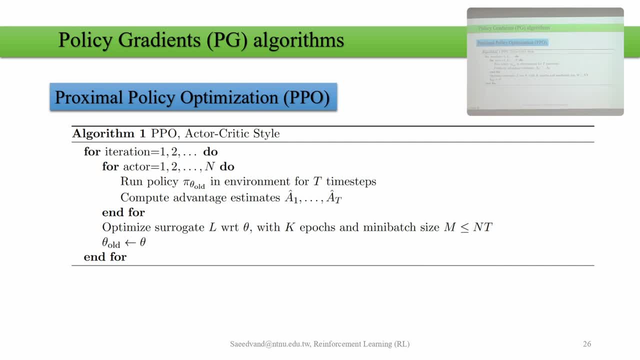 one, two, unlimited here. then for for actor network, one, two, n. Run the policy in the environment at each one of the time steps, compute the advantage estimation and, after calculating the whole Advantage in the in the loop, then optimize the surrogate L by cutting it, By limiting it, and update the parameters that we have for the network and then bring the new, new parameters to the end. 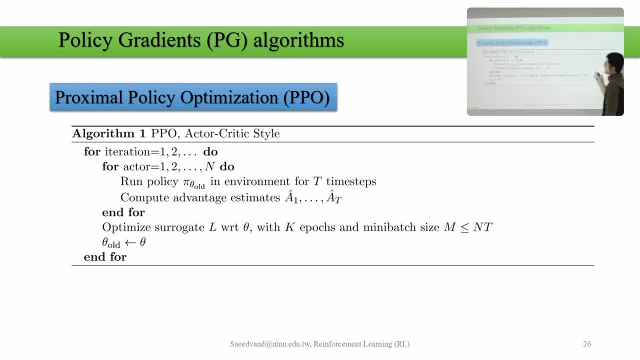 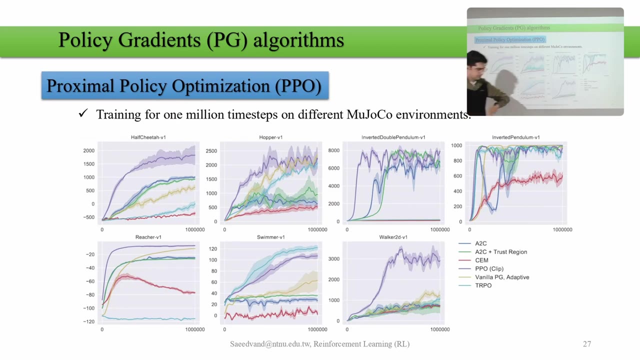 And and then loop it. but this is the. this is the basic algorithm. This can, based on the different algorithms can be, grow, change a little bit. I told you we have different kinds of people that they try to improve it and change some. some equations and follows here. 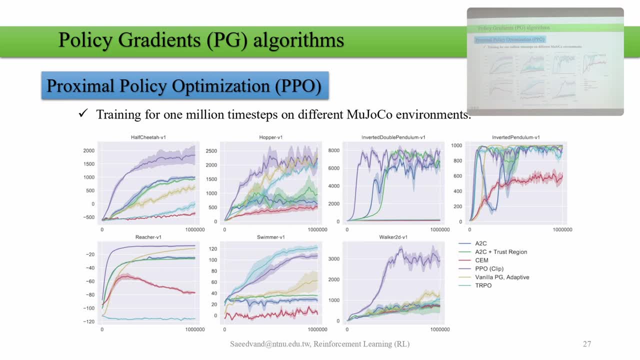 Let's have a look at the comparison of the PPO with other algorithms. here, A to C is the version of the actor critic. We have A to C added by trust region and trust region is also trying to limit with something like tripio and But, but it's based on trust region. It's another technique. We have cm, We have PPO clip agent that today we studied. 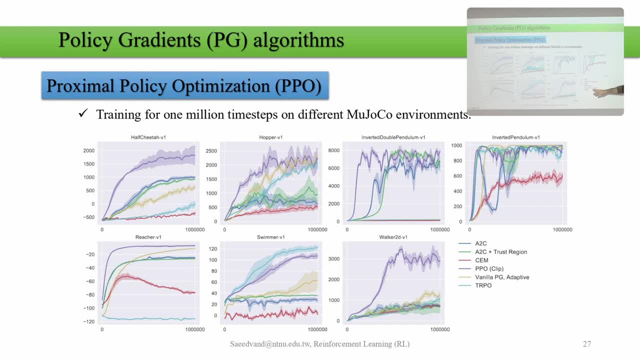 We have vanilla policy gradient. that also today. we studied TPO itself and let's have a look at the performance. I think this- this is, yeah, based on the more juco environment and 1 million time step of running the technique. so by looking at PPO, that is purple here at the first example, here PPO is performing pretty. 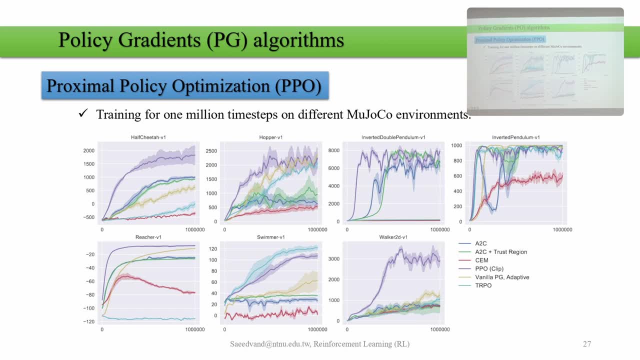 Better than the other one. next place is the actor critic. then PPO is down here. I don't know why. what happened to? usually towards good? But I think that's because it's very complex and, and you see, it's like it's still trying to converge if we continue. 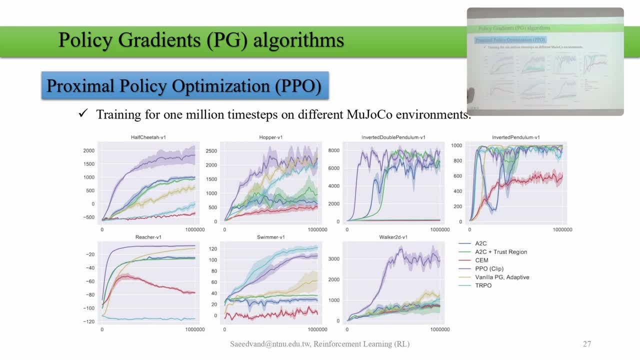 Maybe 10 millions, Maybe this guy comes up there, but this is low. Then in second environment you can see that hopper, another algorithm, again PPO- is working better. The second one is vanilla, that today we study Just just. let's have a look at two best ones in the third example. 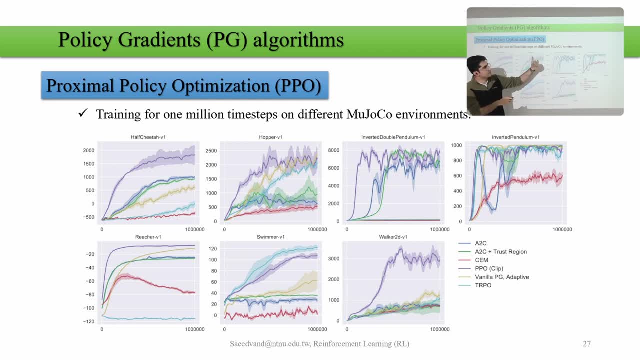 PPO is better. an actor critic with trust region is best Here, almost. they are doing well in inverted pandal. you From more juco, you have in, you have it in Isaac, not, not Isaac. open AIG simulations. We have richer problem here. that again PPO is doing better. 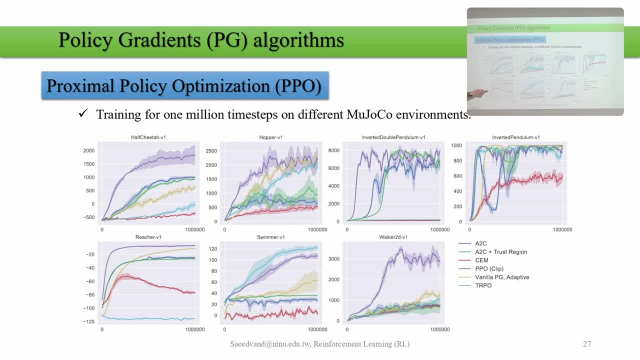 vanilla, second Vanilla policy gradient second: here PPO is not doing well. Which one is trip you is doing well in swimmer problem. You see, you have a problem that PPO is doing terrible, almost not terrible in comparison to. In comparison to trip you is worse. But here in Walker, again, trip you 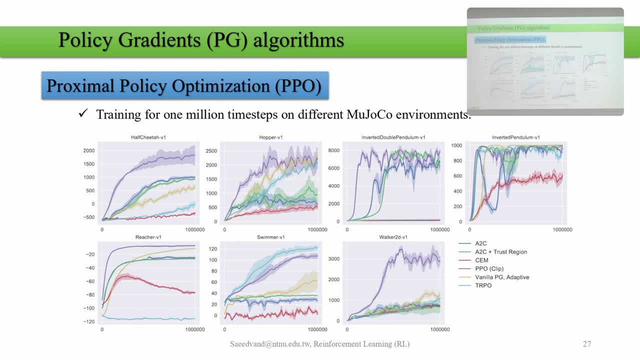 Again, PPO is beating all others If it's with large, large value, large, large amount of improve. And now you know, I don't know. I should think: what's? what's the reason that is very different with the other techniques? Because I think in these problems the reward functions. 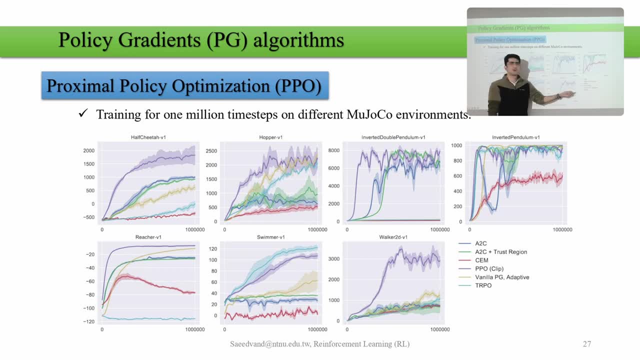 Is like giving too many counties to keep, and they all are forgetting the weights of the of the updates. But, trip, you is doing the same And, and this one day, the, the trust region, is also doing the same. trust region also, creating a region of trust that only you can. 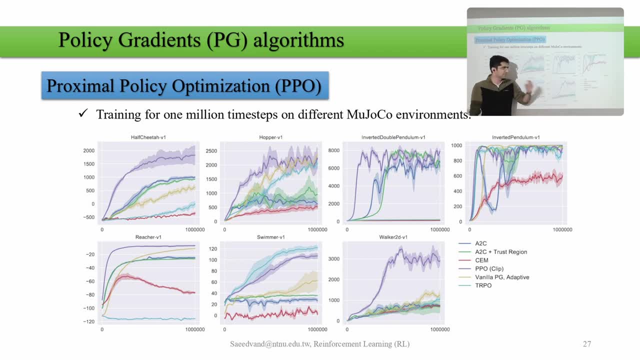 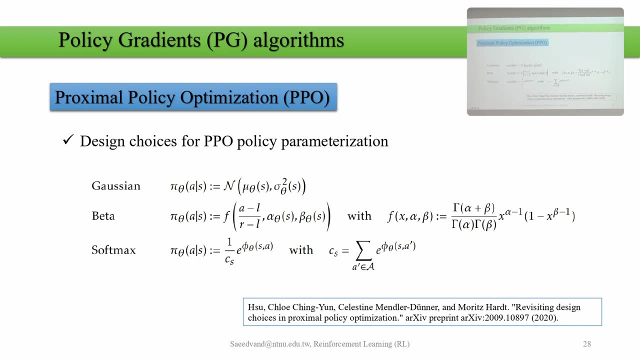 You can update the weights inside that trust region in something similar to clip are different, But yeah, I don't know why, why that's too much different anyway. So Not only that one. we say PPO can be design choices for Different parameterization and the parameterization can be like here: caution. 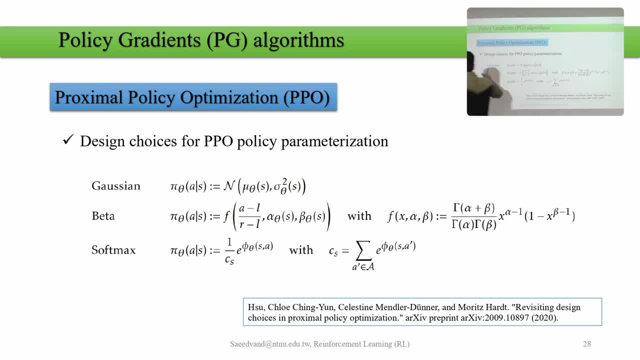 So the parameterization that we have can be caution, not only that one that policy pie can be Can be represented in caution for the policy they did. a TPO parameterization can be based on the beta distribution. You remember beta distribution you implemented, you did examples. so PPO also can be implemented by the 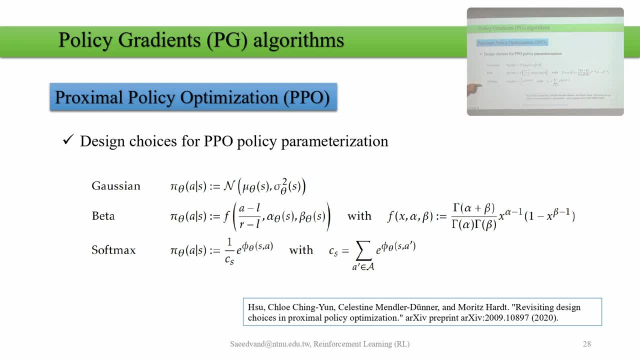 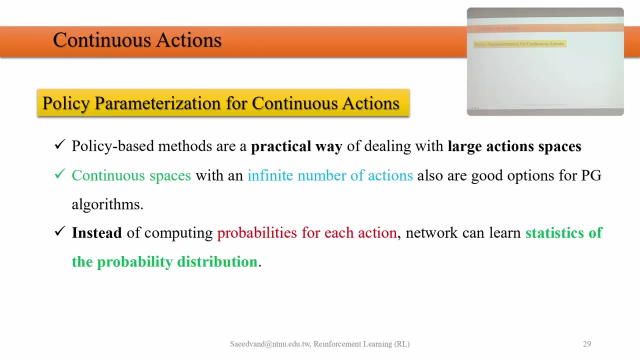 Data distribution that we've sold already can be by softmax as output of the network that I stated many times. So these are representing the outputs of the distribution of the action that can be happen And what does that mean. So in next slide we are going to talk about the continuous action space. so far, 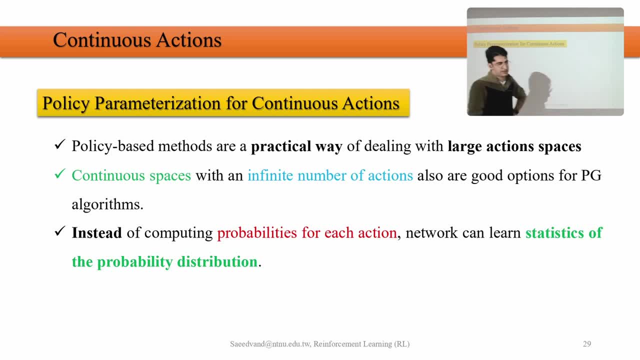 whatever we explained, we mostly talked about the Discrete actions left, right, up down, or or the action space, like it's 360 of the actions. but what if The action space we need to consider as continues to solve it? Now we can answer it. Any idea from you, you guys, how we can bring the continuous action space? 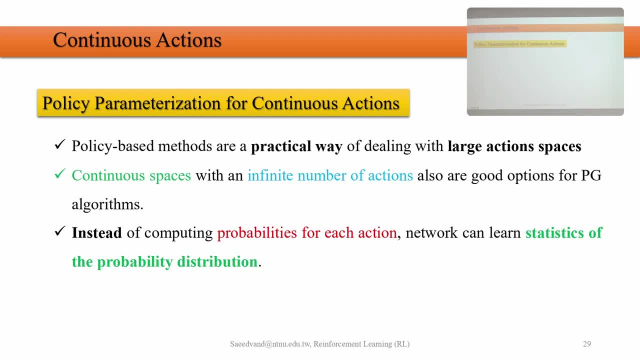 Actions into the game of the, for example, policy gradient. Students who are in Islam class should be easily answered, Because we did a lot with that concept in Islam Okay, so this slide is also very important because it opens a new window to you That you can work with continuous action space. 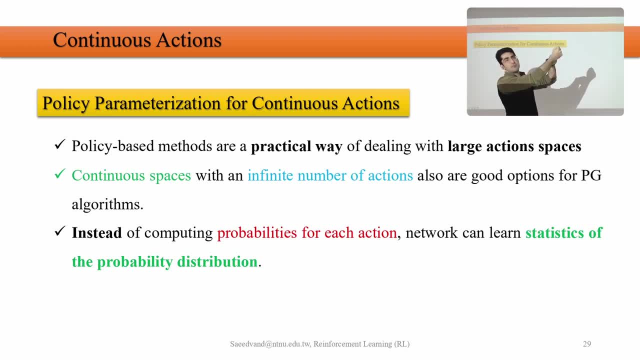 It means that if I'm solving the problem of industrial arm, instead of defining each joint as Discrete reactions, limited number of actions, I can cause it as continuous and say: this is action one in continuous form, This is action two, This is action treat and solving in three continuous forms of the 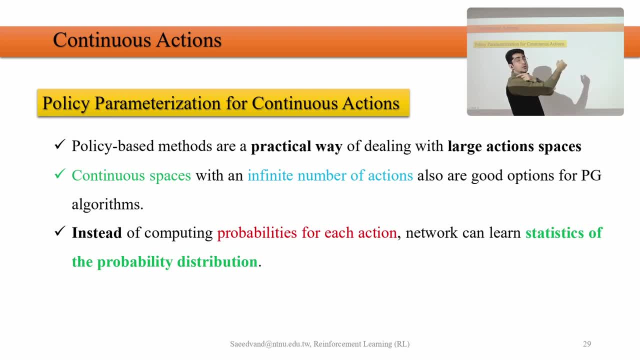 With everything same. we don't need to change anything. We just need to ask the top network should be changed somehow. that I'm going to explain, then solve problem in form of continues How that can happen. we say, Okay, policy based methods are practical way of the dealing with large action spaces, because if they can come, 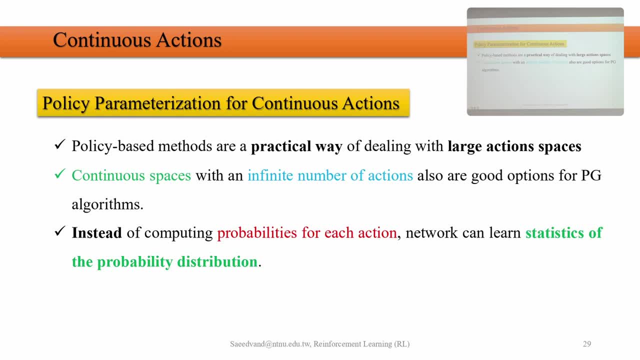 Consider continuous action space. in continuous spaces we have infinity number of actions, even for one, and There are there are good options for policy gradient algorithms and, instead of computing probabilities of each action, We are learning a statistic of the probability of distribution. and what does it mean? 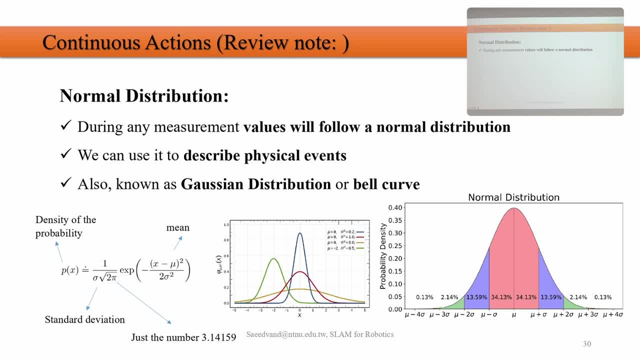 It means that we need to have a look at caution distribution. So if you remove caution distribution, normal distribution, from computer science, robotics, We will fall down. That's, that's very nice distribution. so What is happening with normal distribution? If anybody doesn't know, let's have a look, we can. we can use it to describe the physical events and and. 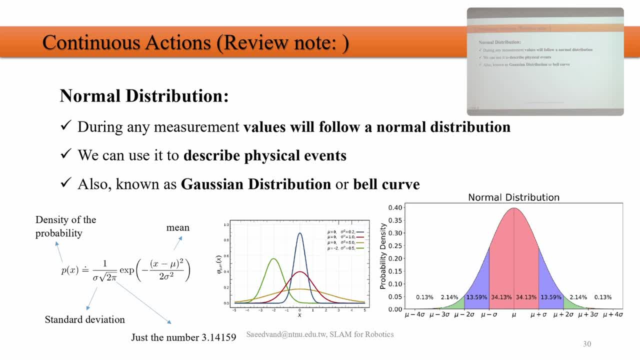 They have different names for that normal distribution on Gaussian distribution or bell curve, and looks like this. Everybody are familiar, most of most, most likely, and we were doing a lot with we did in In Islam course this semester, We have the distribution that you can see. this is the. 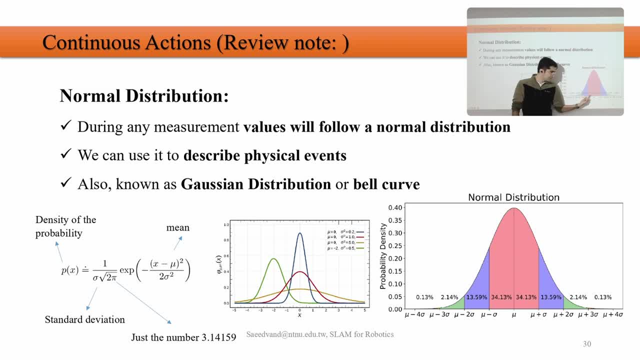 normal distribution and here, in this Variance between minus 2 pi and pi, we have 90 percent, 95 percent of probabilities. and what does it says? It seems that says that if this is proper probability of occurring something, the probability of occurring like in Center is higher. 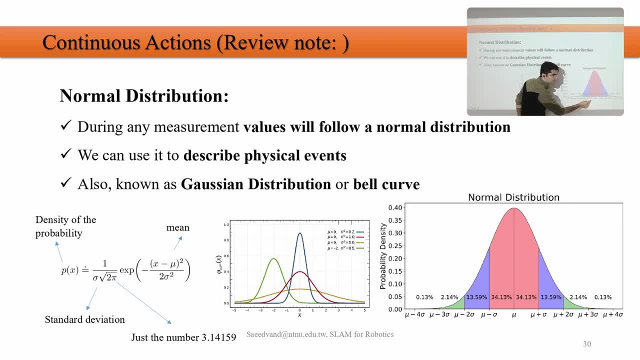 Here is lower, So we show it with mean. mu is mean. that shows very the center of the distribution, probability distribution. so we have the meaning of the mean and meaning of the covariance over there so that if we consider We can represent the normal distribution with this term over here, the long term of the 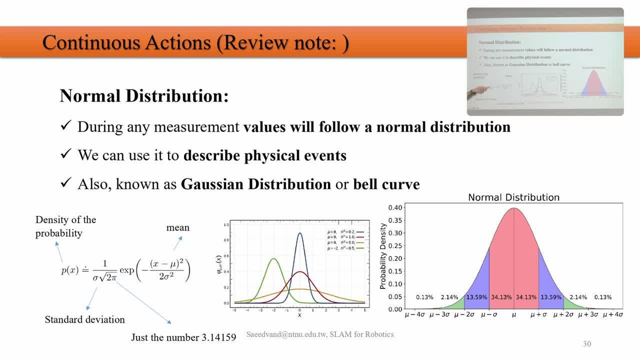 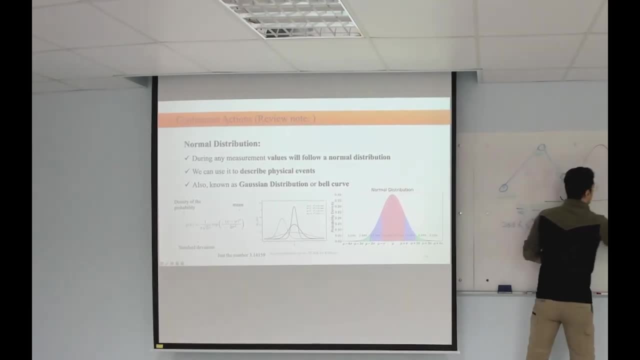 density. probability P of X is equal to This term over here, that here we have the mean and here we have the covariance or standard deviation. What does it mean? It means that it says okay, probability of Happening something means, says that is more likely here. with what kind of comma? how much error. 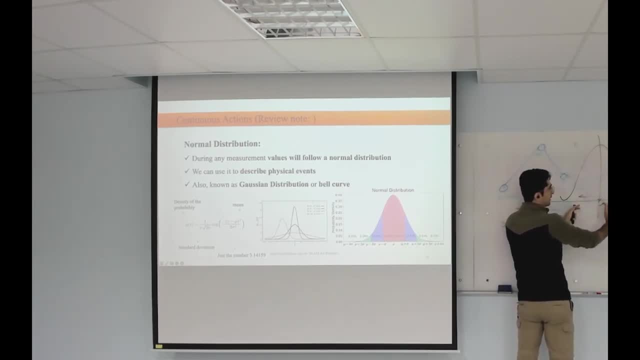 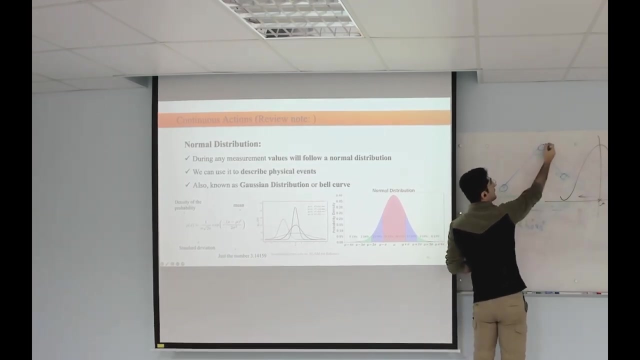 this is Mean and this is covariance. That's how much error and How. where is the probability of the happening? now, before even continuing forward, Let's say- Let's say this joint over here- that we have as a robot. so this is, This is 0 to 360 degrees. 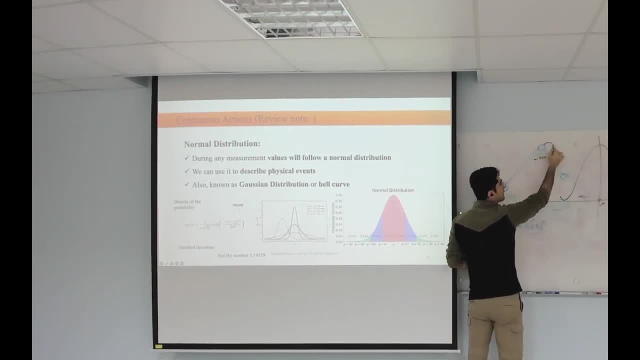 If it's revolution, then if I can consider it as this part over here, Then what can I do? this is continuous action space. then I can show my action space By mean and covariance of what is the probability of the one action to happening over here. 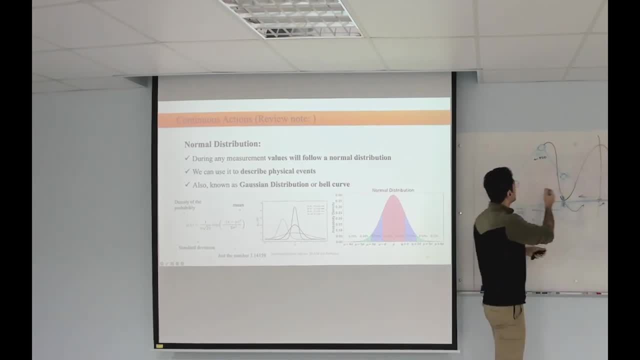 So that, for example, this is: if you consider rotational like this is like zero, rotating 360, then we can say that, okay, Here is the, for example, this action And how we state it, we state it by the mean. And what is the error of the? 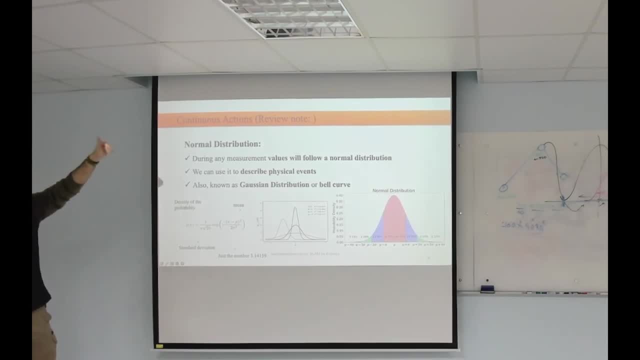 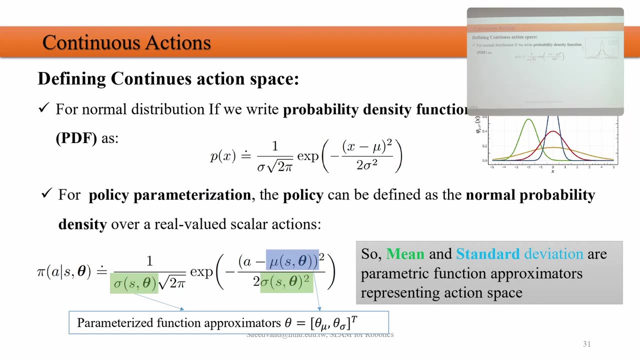 So if that Gaussian distribution, This mean and covariance, can be adopted on the action space that I have, then I can do this one. The probability distribution function, PDF, can be really turn some weights of the neural network so that we are trying to parametrize the mean and 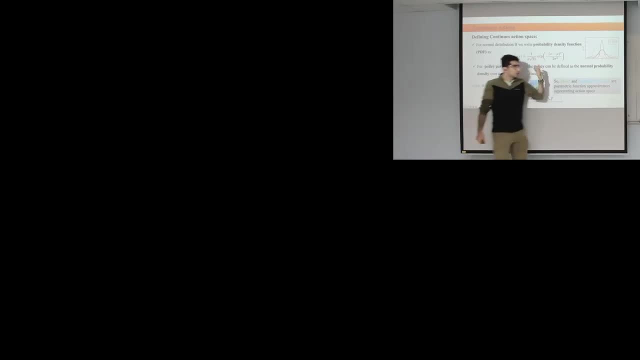 The data, covariance and the mean. Try to learn, find where the mean and covariance should be. this Accurature will follow the mean. for example, their action should be performed here, here, here, here I'm changing the probability And the covariance. how certain it is. the certainty is higher, more likely. that is better action to do. 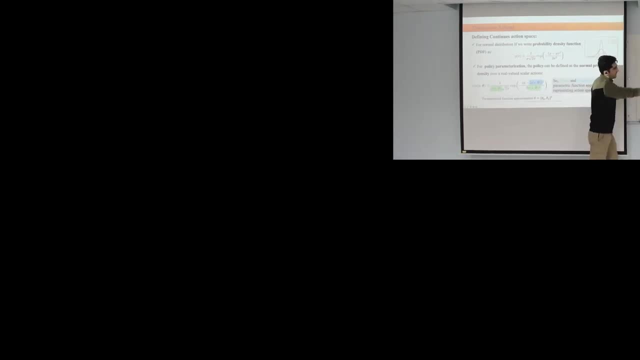 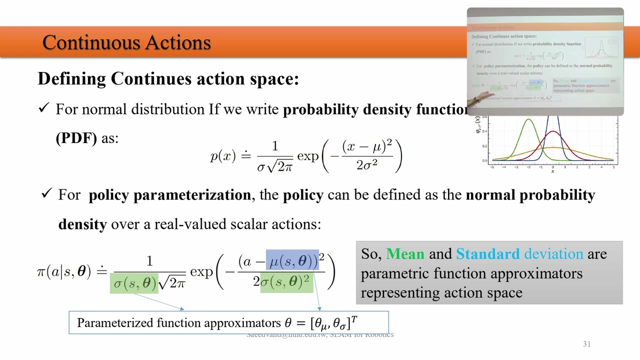 So instead of learning whole action space, I just can learn two parameters- the very mean is very how much error is- and Parametrize it in terms of the policy action given by state and theta in form of normal distribution. Gaussian distribution then solve my problem, Then the output of network. 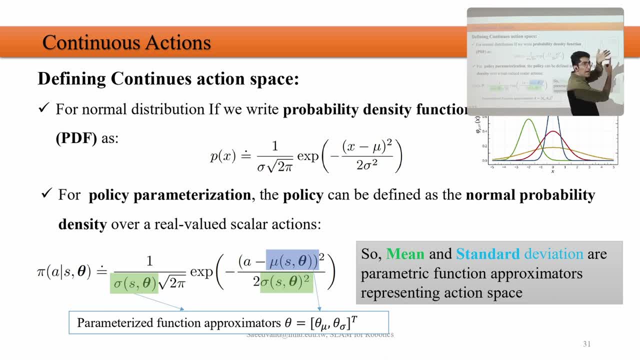 Will be something similar to for each action. If I consider normalize 0 to 1, for example 0 to 1, then I can say for each action, for example for destroyed, I can just learn two parameters, mean and covariance, To say well, what is the probability of that action happening, so that my deep reinforcement learning for actual critical network or policy. 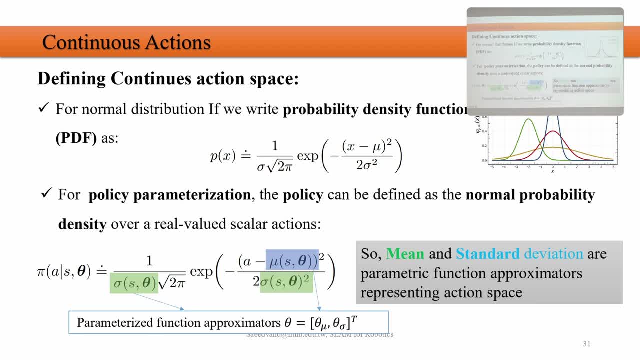 Gradient can learn it Clear. So this is the general concept of bringing mean and standard deviation into game, and this is the term that Can be used in order to do this. there are different other different ways to, but this is one of the common ways to parameterizing the. 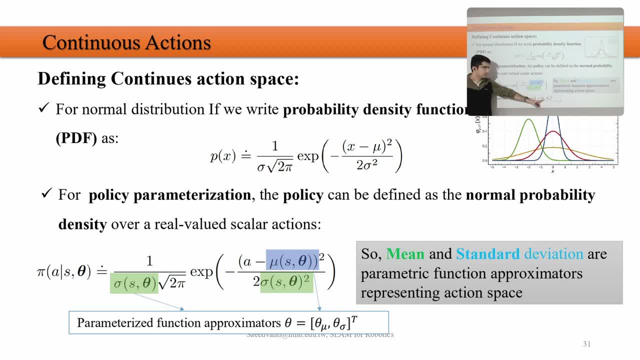 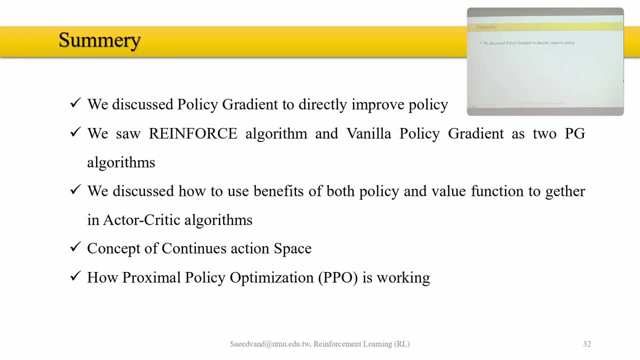 function by adding the theta, theta, theta, mu and theta mean to the, to the representation of the action space. So what did we study today? today we study, discuss the policy gradient and How we can directly improve the policy without calculating value first. then we study to reinforce, and one in algorithms.